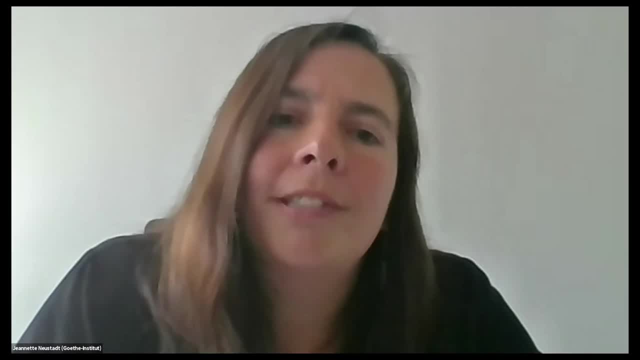 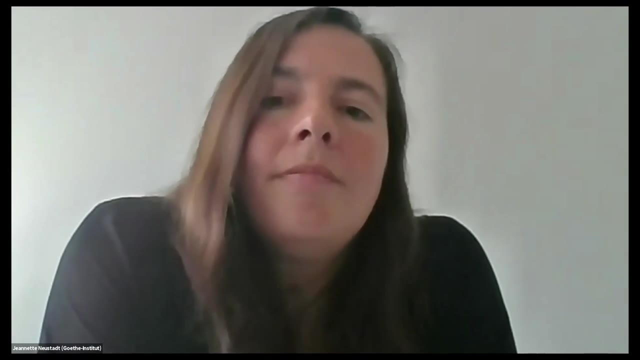 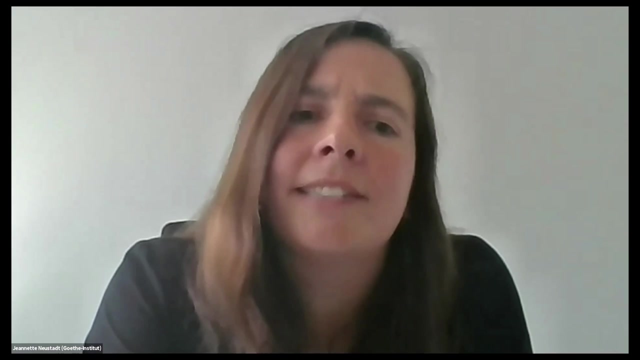 We promote the study of German language abroad and we also encourage international cultural exchange With the Couch Lessons. we want to initiate a discussion outside the technology-savvy community and the Goethe-Institut. The Goethe-Institut deals with this topic because AI has and it will have a huge impact on our society at different levels and in various fields. AI will contribute to a new revolution in human history. 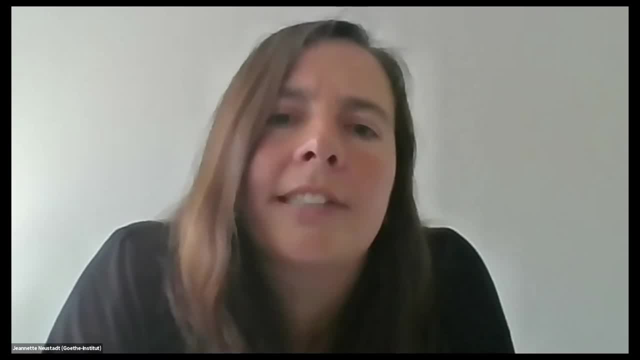 And this fact raises a lot of questions. How intelligent can machines become and can they make fair decisions? Are we threatened by the automation of society through algorithms and AI Will initially human skills, such as the creation of machines. therefore, beyond programming, it Planes. 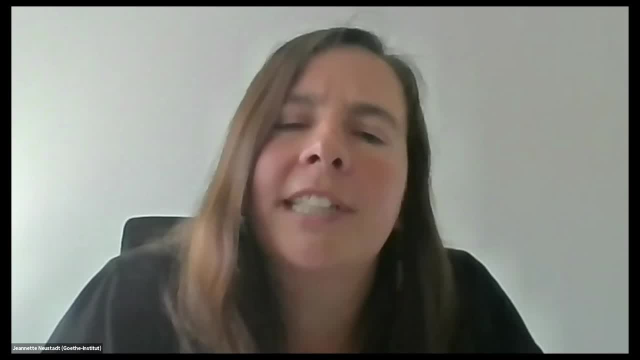 or digital pulsarson? curation of art be computerized, or will AI make the world a better place by helping us solve big problems such as climate change, pandemics or inequalities? Do we still have to work in the future? And if we don't, 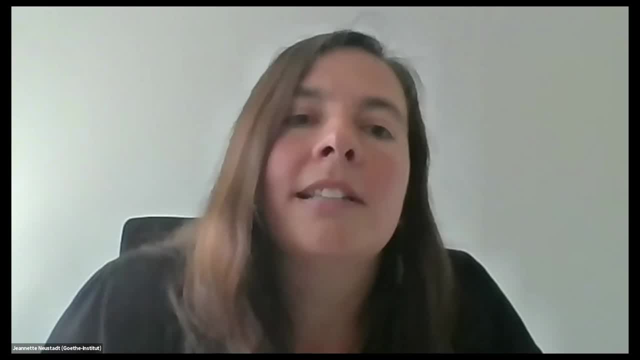 as AI shapes our society for better or for worse, it should be on all of us to decide what direction we will take. The Couch Lessons are an invitation to find meaning behind technical developments in the field of science, field of AI, inspire new ways of thinking and create our collective future. 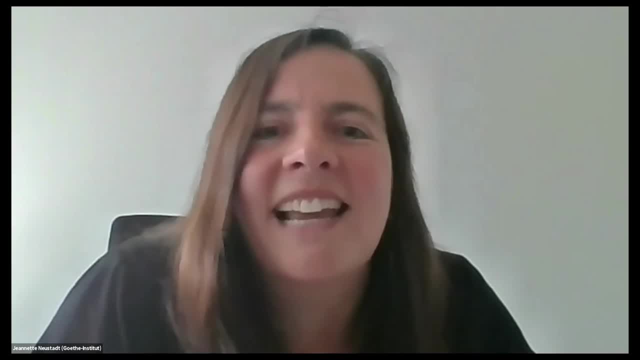 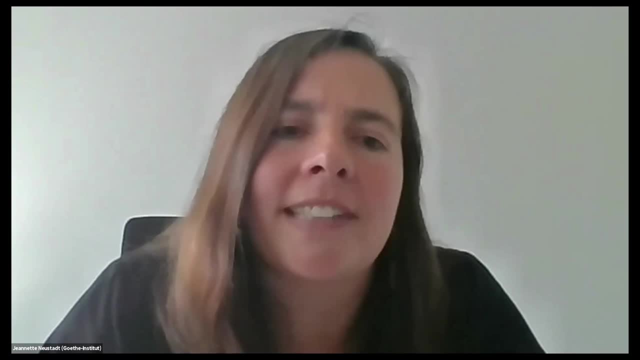 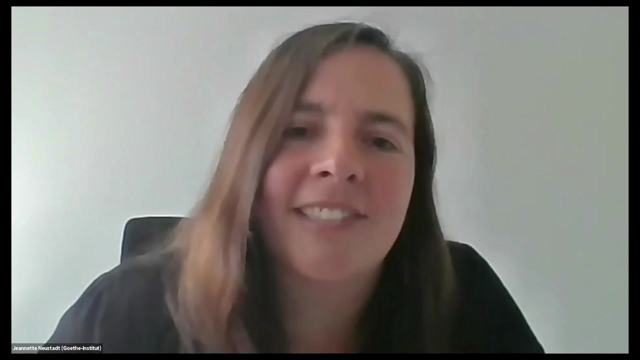 Today we will ask what robots can and what will they do today and in the future, and how they interact with humans. And for the beginning of this couch lessons, we have prepared a poll for you, and maybe my cohost Martin can read them, because I cannot right now. 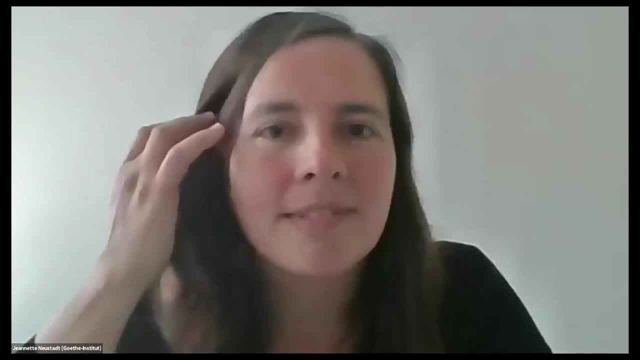 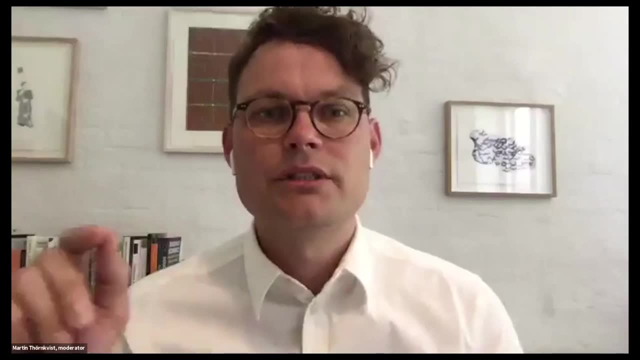 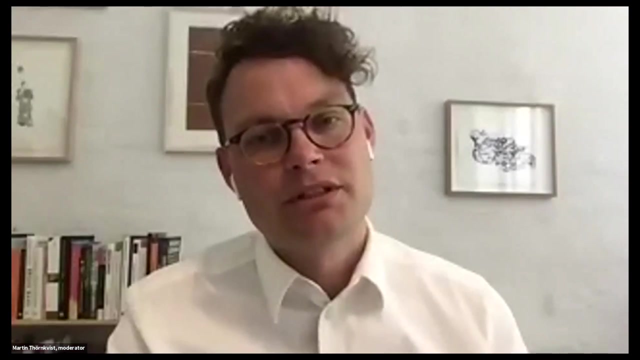 Martin, can you read the questions? Sure, So I think everybody can see the questions as well on your screens now. And the first question says: will robots replace humans? Can? and the second one is: can you imagine a robot taking care of you when you're old? 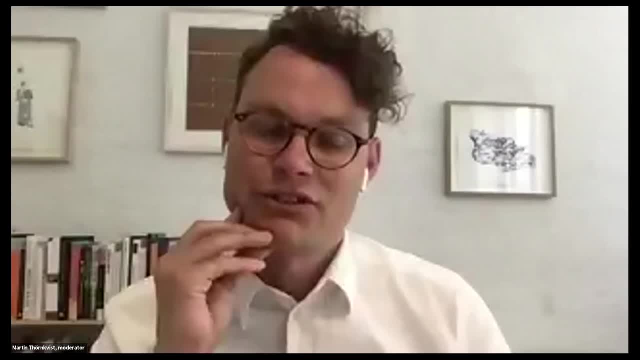 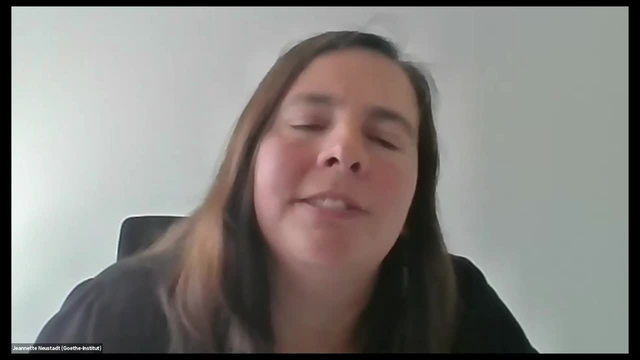 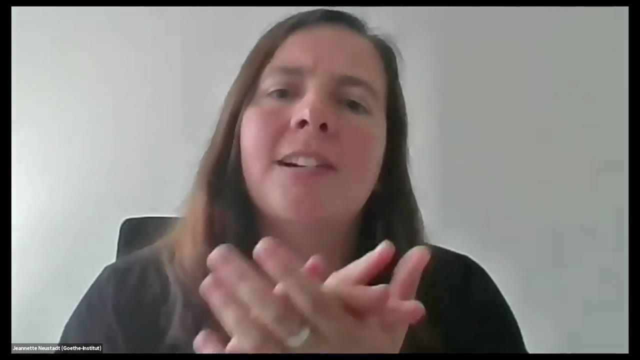 And the third one: can you feel for a robot? Can you have feelings for robots? Yeah, And as long as we wait for your answers, I would like to inform you briefly about some guidelines of the couch lessons. First, our two experts will give an input, each about 15 minutes long. 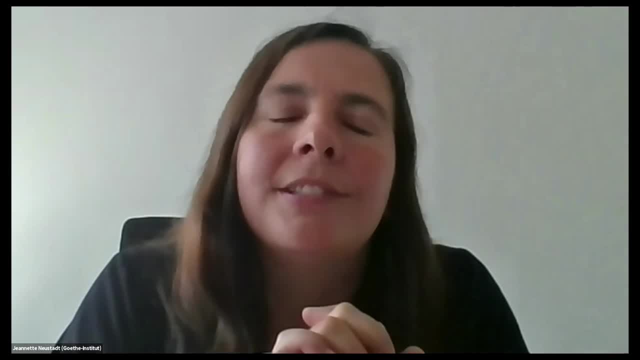 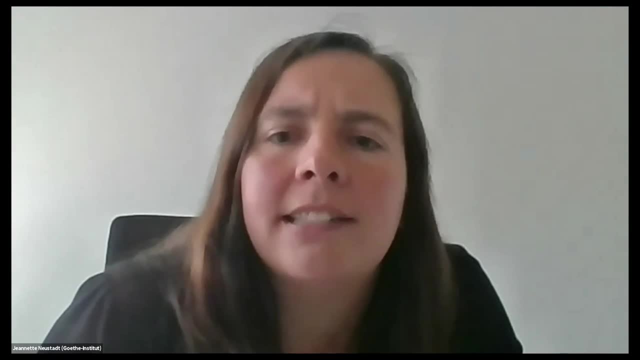 And after that we will open the discussion for all of you, And during the whole time you can ask questions or contribute your opinions in our chat, And I will go through the chat and pick out some of the questions and thoughts and then we can discuss them later. 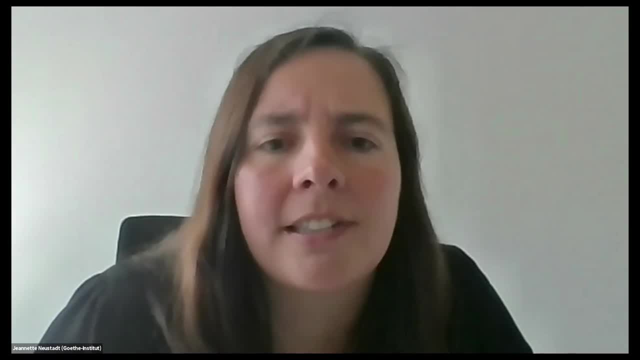 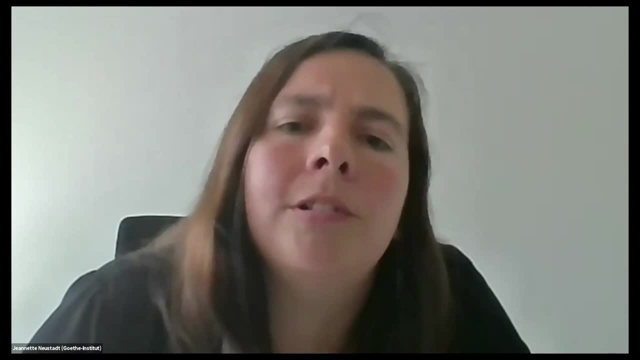 I will ask different persons to contribute the questions personally, but if I don't ask you to talk, I will not be able to answer them, So please turn off your microphone. I also want you to know that the whole event is recorded, but we will just record the persons that are speaking. 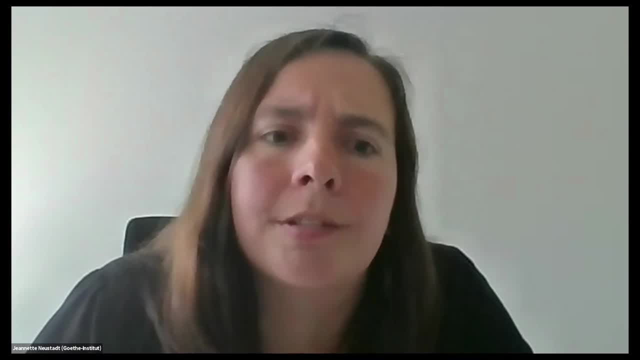 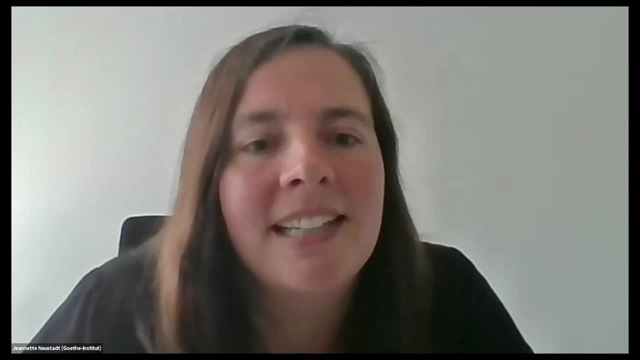 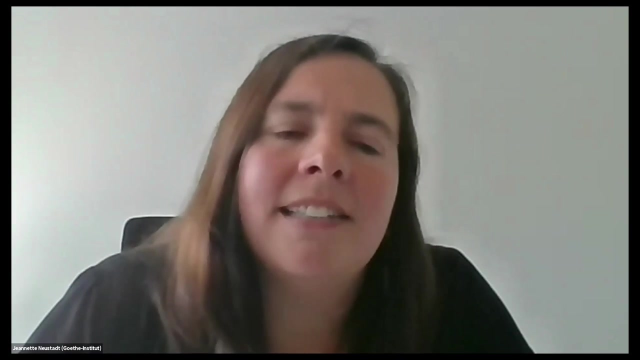 You can always turn off your video and switch off your microphone, Although we would invite you to switch on the video so that we all can see all the participants of this event, And for that we would recommend to use the gallery view. So let's have a look to the results. 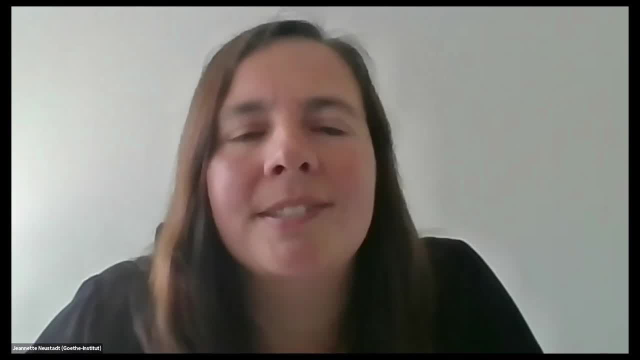 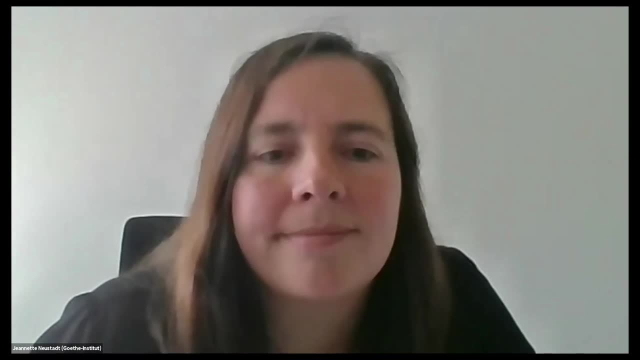 And with this I hand over to my co-host, Martin, from Sweden, who helped me with the presentation. He helped me curating the series and who will moderate it. Thank you very much. So, yeah, I think you can all see the results of the poll. 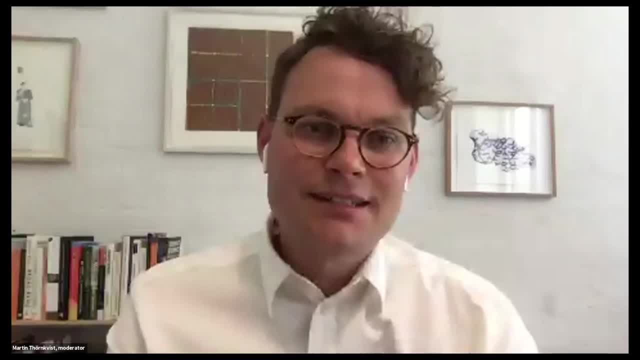 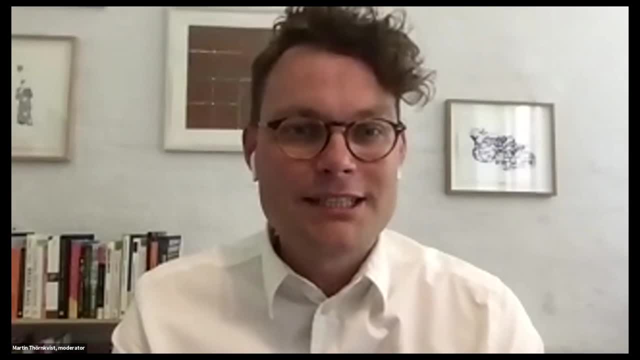 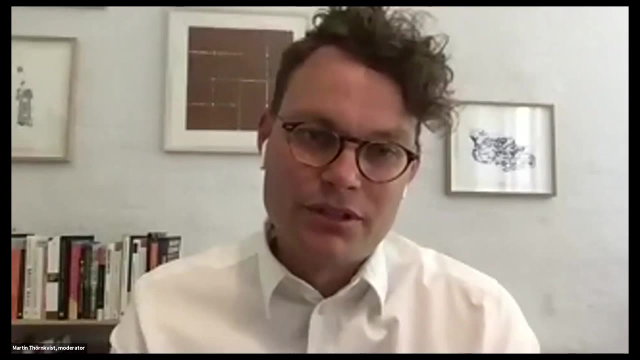 And most of you- 63%- think that robots will replace you in the workplace, but not otherwise, And 50%- a little bit more than that- can imagine having a robot taking care of you when you are working. So yeah, I think you can all see the results of the poll. 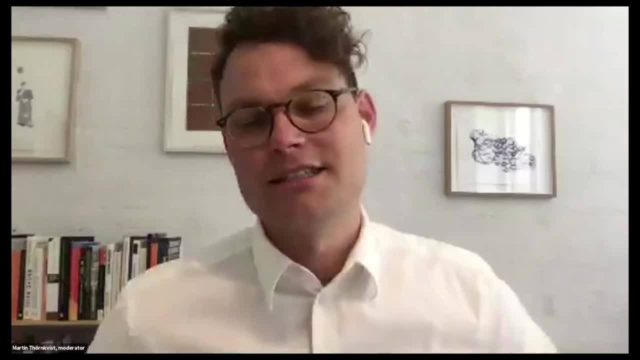 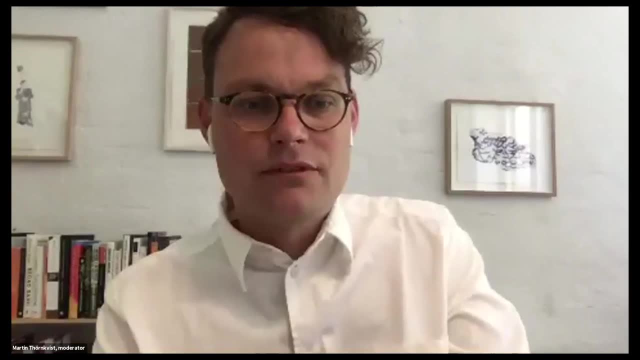 And then can you have feelings for a robot, It's a little bit undecisive. So we're going to share this or take a screenshot of this, And then we will actually ask the same questions again at the very end. 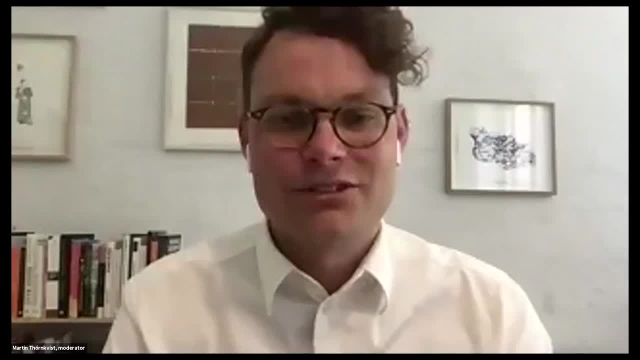 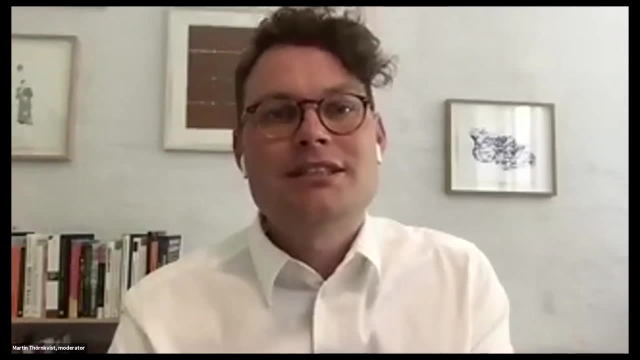 And we'll see. if you have different answers to these questions, then So, as Jeanette said, my name is Martin Tarnqvist And I'm a curator And I'm a researcher And I'm a context maker based in Malmö, Sweden. 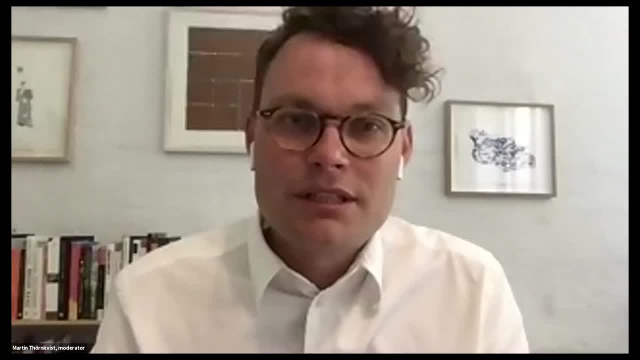 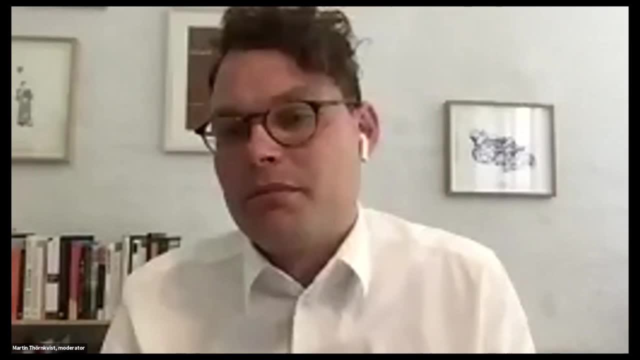 And I know that we have participants from all over the world in today's lesson. So if you feel like it, please say hi and type where you're joining in from in the chat, Because even though these sessions online are somewhat common now, 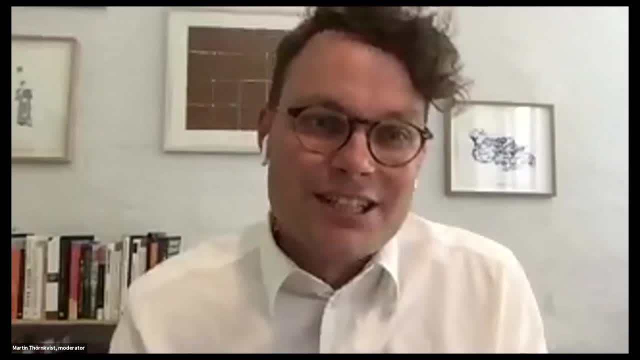 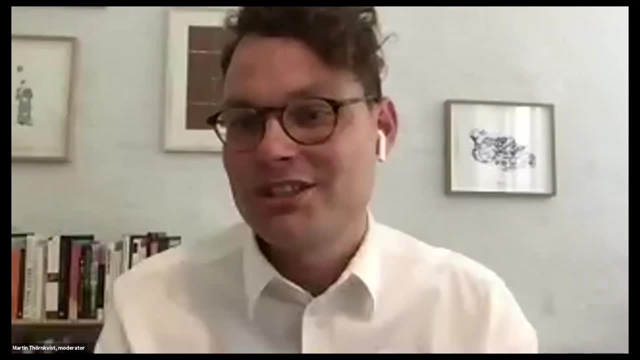 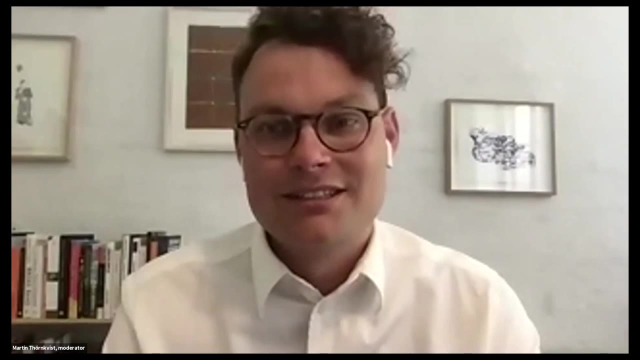 I refuse to take the magic of global gatherings for granted, So it's always a beautiful thing to see, like Argentina, Sao Paulo, Warsaw, Tel Aviv, Johannesburg, et cetera, et cetera, And I think it's amazing that the Goethe Institute have a presence all over the world. 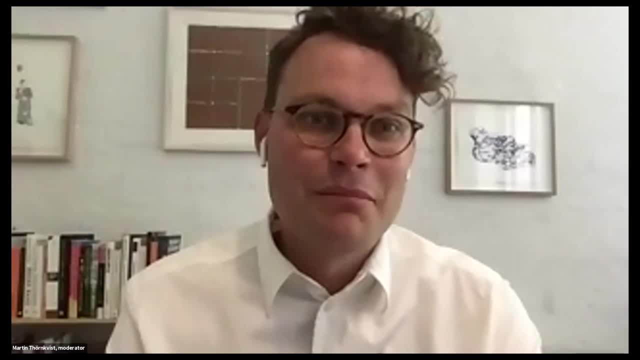 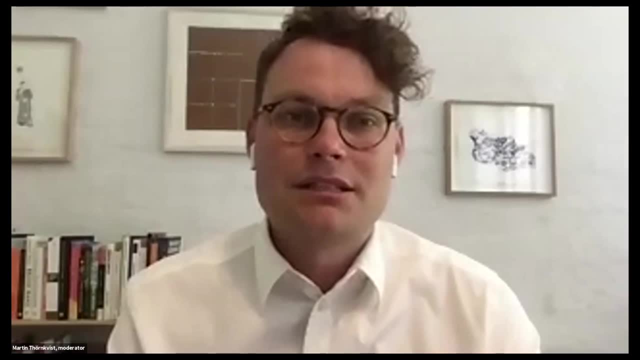 So thank you very much for showing up. It's truly amazing to have all of you here. So this morning I was thinking about the questions we're posting in today's couch lesson And I was thinking about what interactions I've had with robots in the past week. 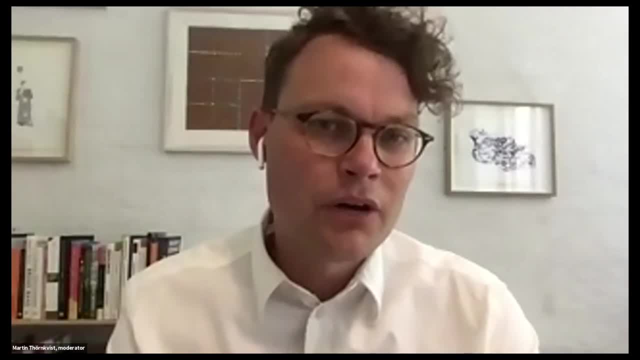 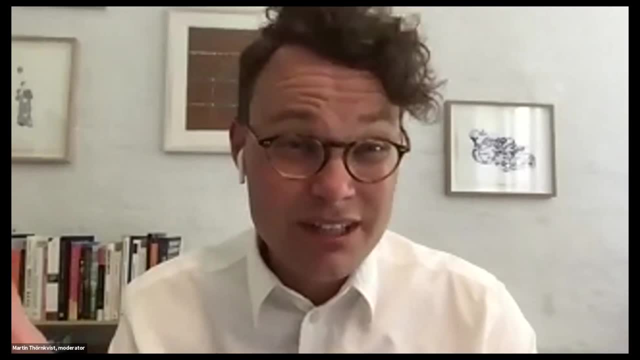 And in the way my five-year-old son would draw a robot. It's none. But then I recall the drive to the countryside, And I was driving in a quite ordinary, yet new Volvo, Of course, since I'm from Sweden, From a carpool that I'm using. 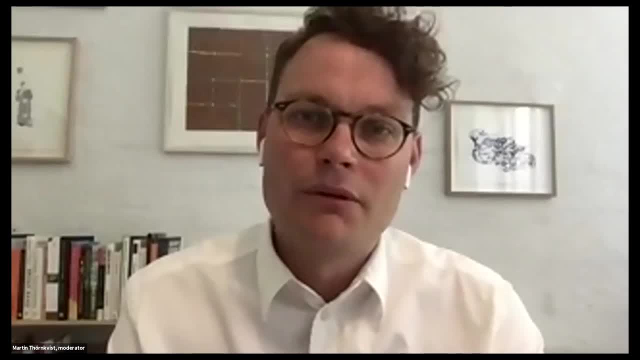 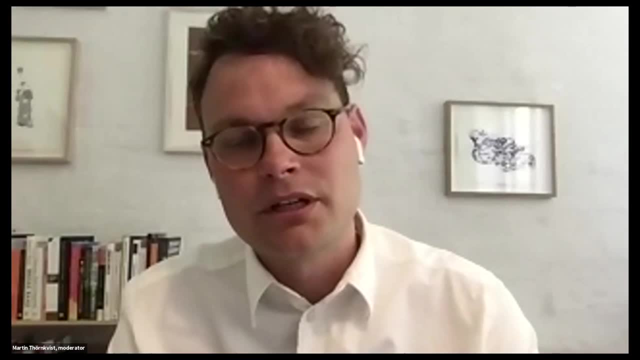 And when I was driving with cruise control on, I was poked to turn pilot assist on And with that on the car not only keeps distance to the car in front, it also takes over the steering wheel and keeps me in the lane. 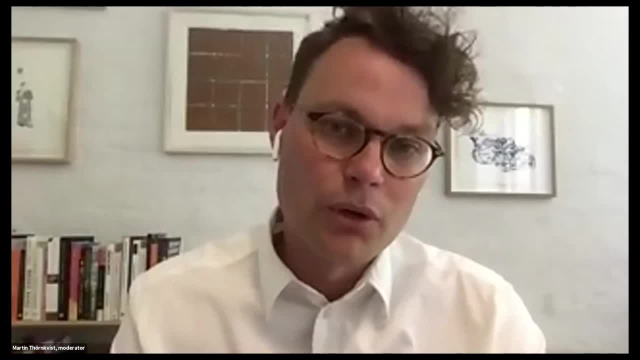 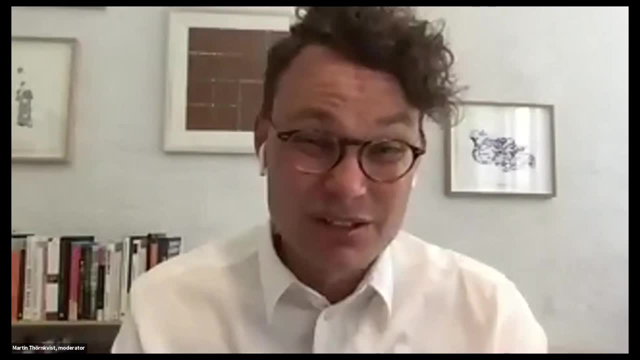 It's not self-driving per se And it doesn't look like a robot, But as a driver it sure felt like it's taking care of itself somehow And also, to be honest, it also feels a bit scary and prompts a lot of questions. 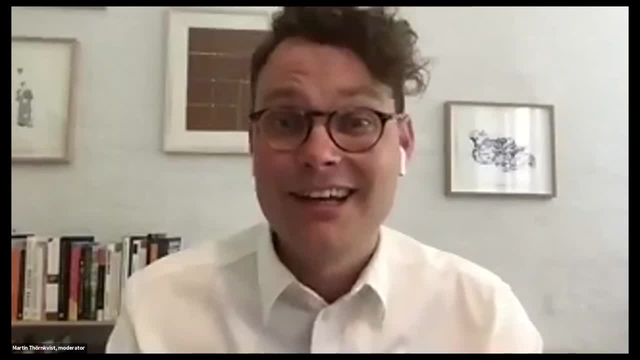 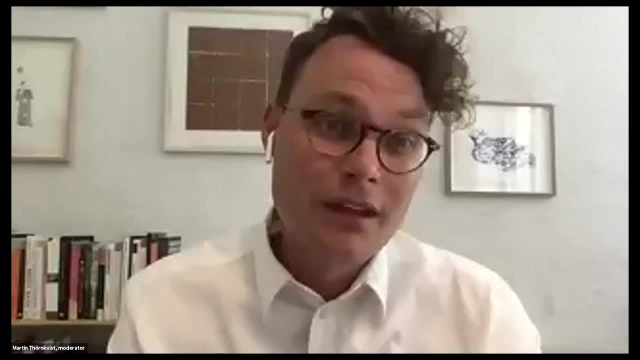 So how does this work? Does it work? Why is it making other choices in micromanaging the steering than I would have, And so on? And so there's always been an interface between man and machine in the case of driving. 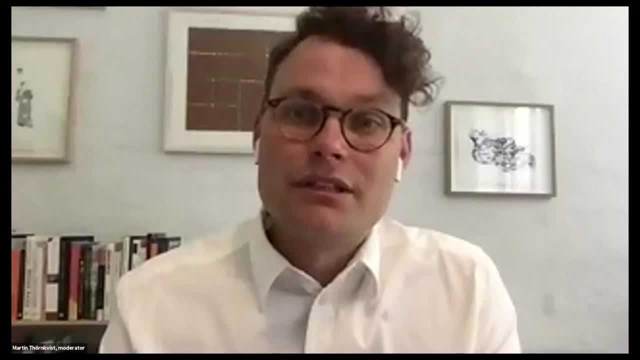 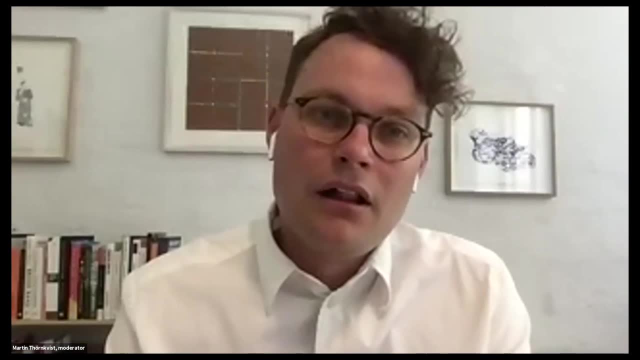 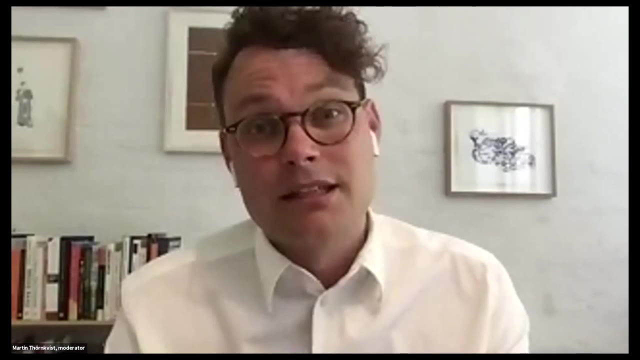 But it's slowly but surely moving from sticks and ladders that I feel in direct control of to a more intelligent and autonomous set of technologies, And although it's not yet fully self-driving, this example made me realize that it's the word interaction that is the one to look out for today, if you think about the title of today's session. 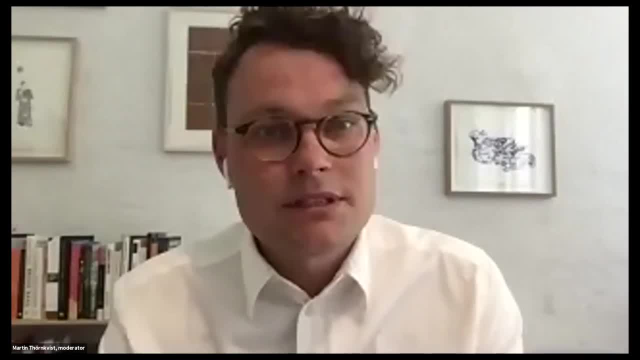 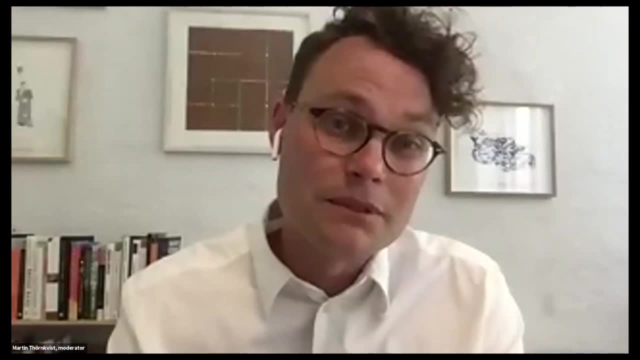 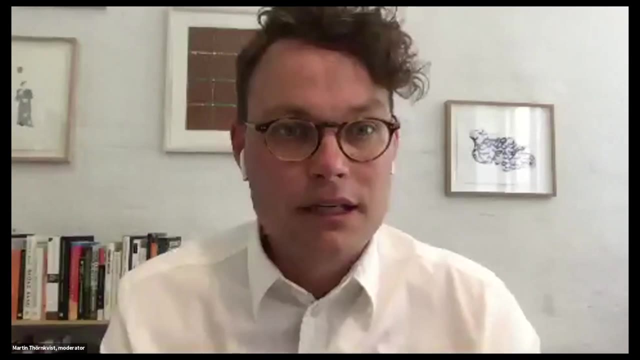 Because intelligence machines are a part of our lives, but it's up to us to see them, acknowledge them and either feel empowered by them or address the problems that might arise in our developing relation. And it's this emerging interaction between humans and the increasingly intolerant technology. 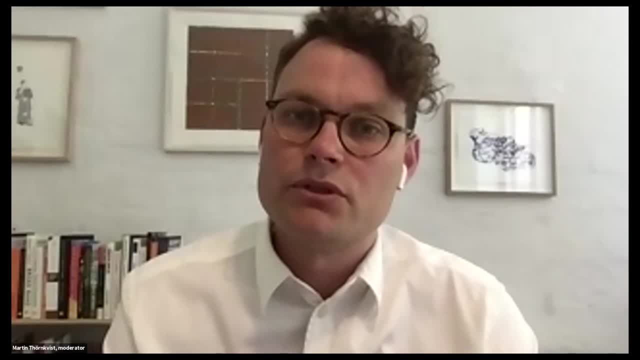 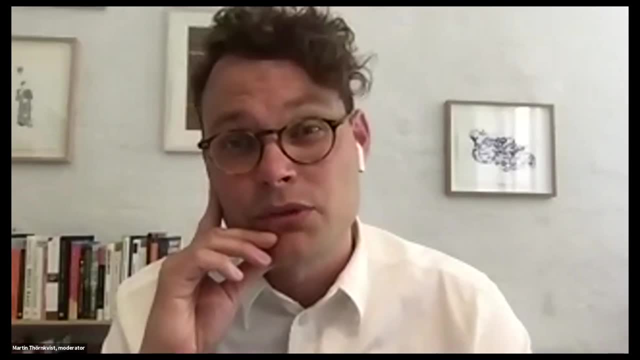 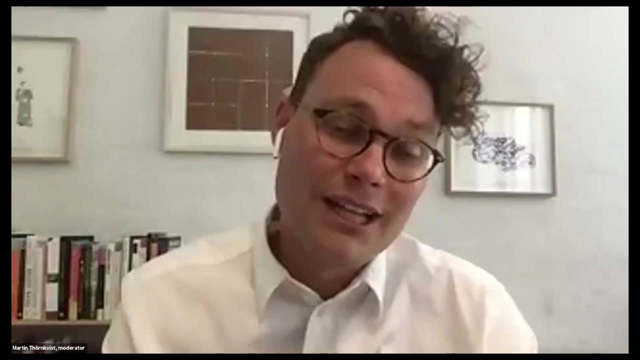 that this Couch lesson is going to revolve around, And with us to explore the potential and complexity. we have two distinguished speakers. We have Professor Sami Haddadin and also Dr Kay Darling, So let's jump right into it. Our first presenter is Professor Sami Haddadin. 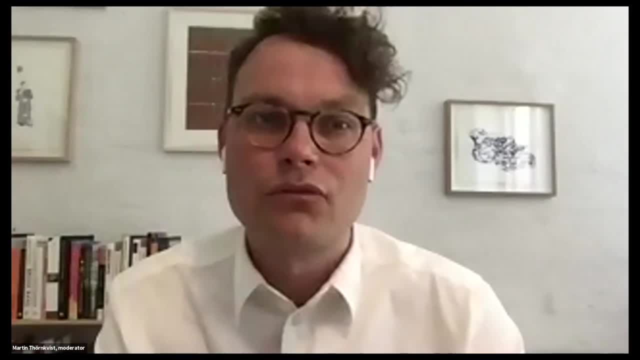 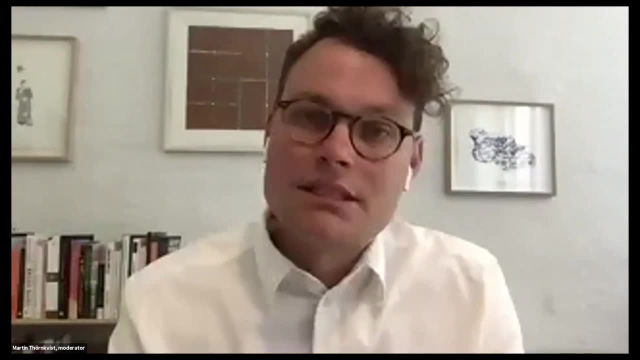 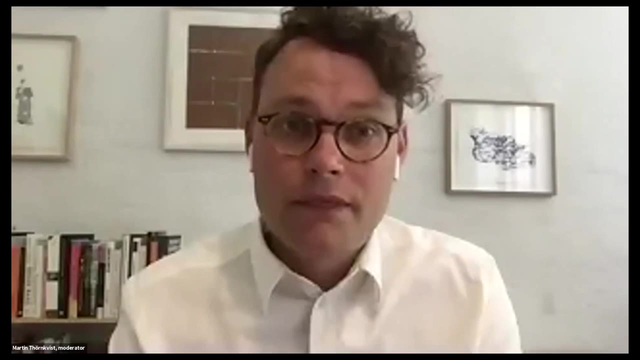 He is the director of Munich School of Robotics and Machine Intelligence at the Technical University of Munich And he holds the share of robotics and science and systems intelligence For us. he's going to define what a robot is, give an overview of what they're currently capable of. 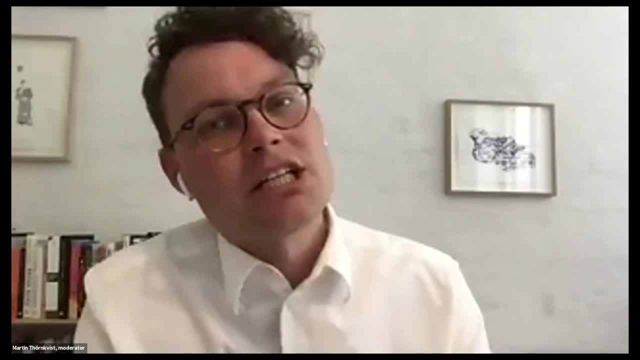 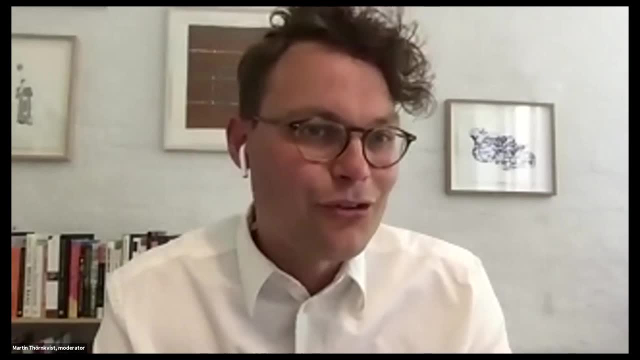 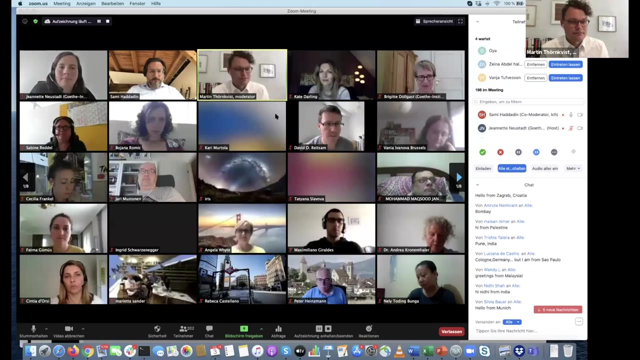 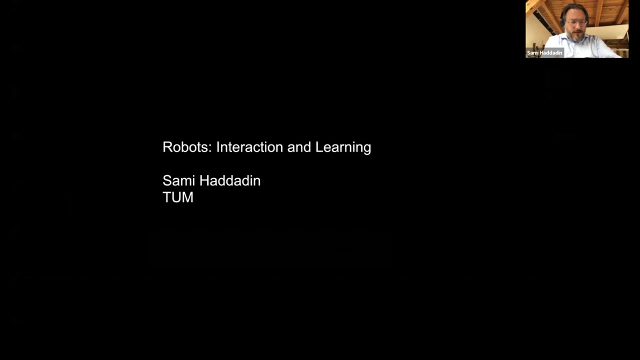 and also hint to how human-robot interactions develop in the future. Please beam your energy to Sami. The screen and microphone is yours, Sami Wonderful. Thank you, Martin, for the introduction and also to Jeanette for this wonderful invitation. 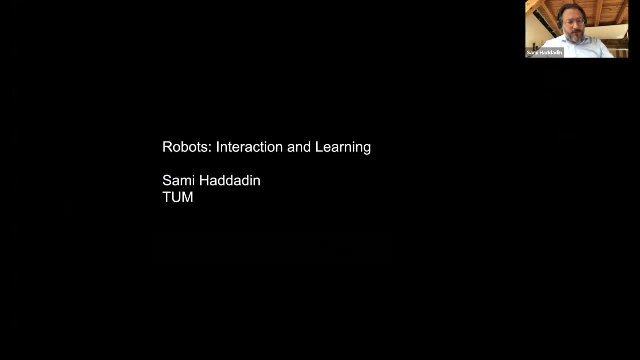 It's a great honor to be here And maybe you could just quickly confirm that you guys can hear me well, and the screen is shared. Maybe just give me a hint. Great, awesome, Okay, so Martin was basically taking away everything that I'm going to talk about today. 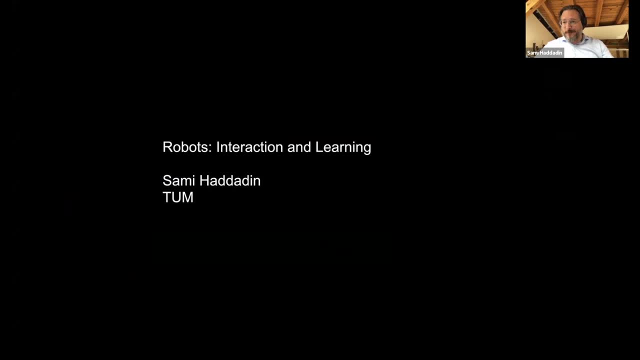 At least 50% is going to be about interactions. So I'm going to talk a lot about robots interacting with the world, and this being the primary thing about robots, And I think it's kind of interesting if we look at kind of the future. 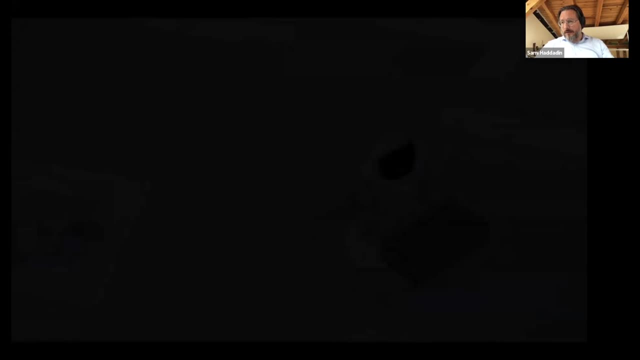 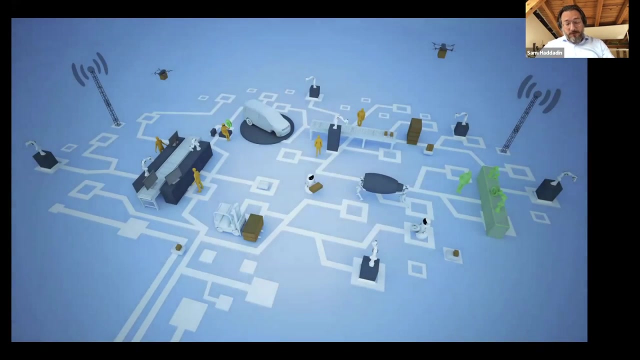 that we all, I guess, are looking forward to. We all are kind of facing a future society that is living about. it's about living with machines, interacting with machines, humans and humans, humans and machines in the future of industry. 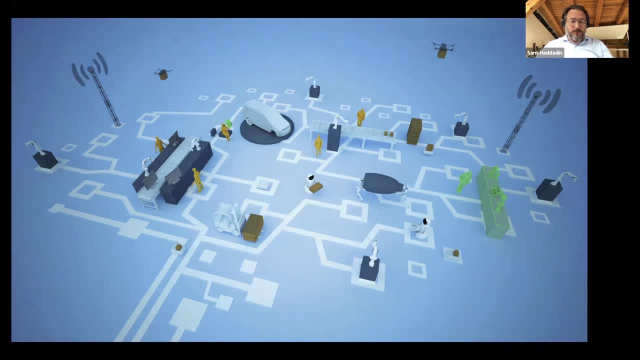 future of work mobility, but I guess also in the future of our general society. We can see that these machines, I mean this is the reason why we can all come together, this wonderful happening that Goethe-Institut is kind of giving us. 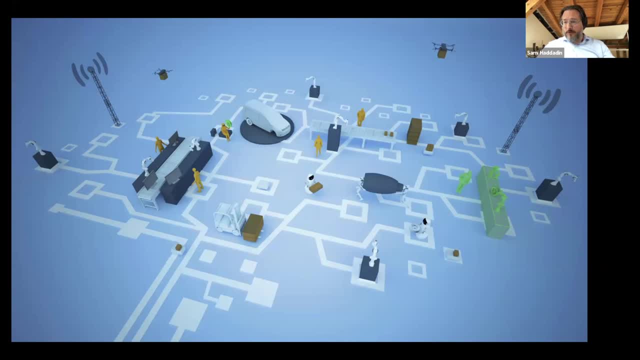 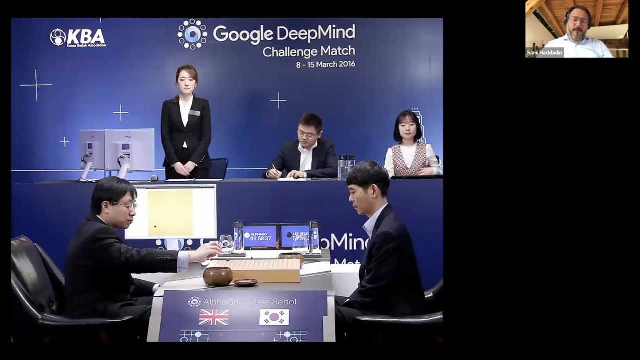 that these interactive machines are part of our society. They're becoming more and more. However, I think it's kind of interesting if you really look at the way that these big leaps forward that we have seen in the last decades are being perceived. I mean, we have all seen Google's DeepMind beating Lee Sedol. 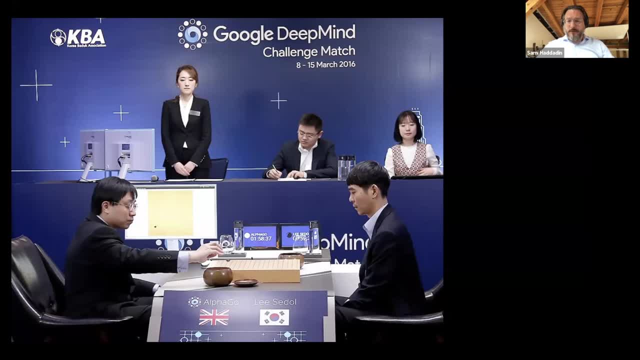 who is sitting here on the right side in the famous game Go. He's a grandmaster of this very complex game. However, when I saw this, this was running on YouTube, running around the globe in 2016, and really showing what current AI technology is capable of. 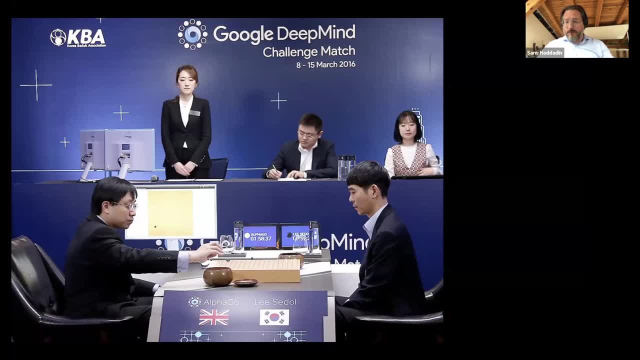 it was kind of interesting when I saw this picture, because you should ask yourself a very distinct question as soon as you look at it, because there is Lee Sedol sitting on the right side. there is AlphaGo, the machine in the back. 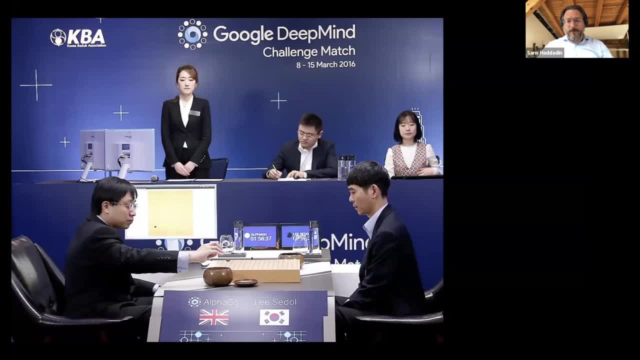 doing the computations. However, who the hell is that guy on the left side right? So, interestingly, this person is solely there for executing the steps that the machine is planning and deducing in order to beat Lee Sedol. So when I saw this picture, 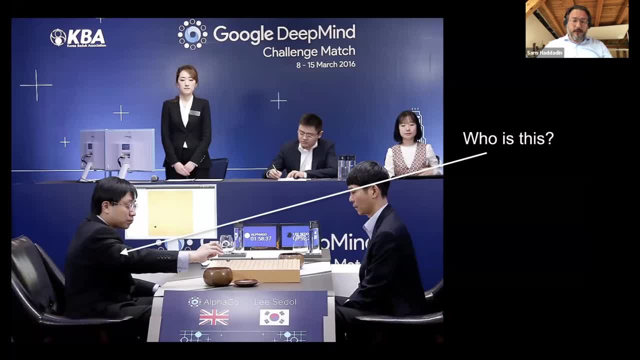 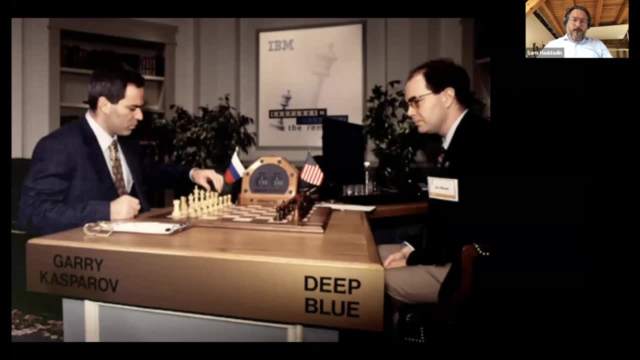 I was really thinking about my own childhood when I was in high school, because I kind of had a similar experience already. So there was a deja vu that I basically had, And this was in the year 1997, when essentially the same situation happened. 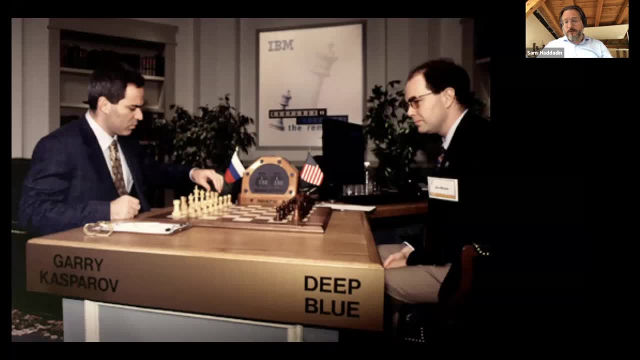 Deep Blue was playing chess against Garry Kasparov. Deep Blue was the previous DeepMind, And the company at hand that developed that system was IBM at that time, And we could ask the same question, right? I mean, on the left side there is Garry Kasparov. 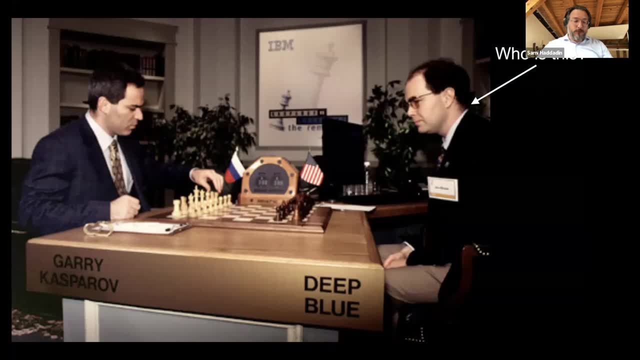 but who the hell is the guy on the right side? So obviously we don't believe that, within more than 20 years of research, the only thing we could do is to place a human from the right side to the left side. However, there seems to be. 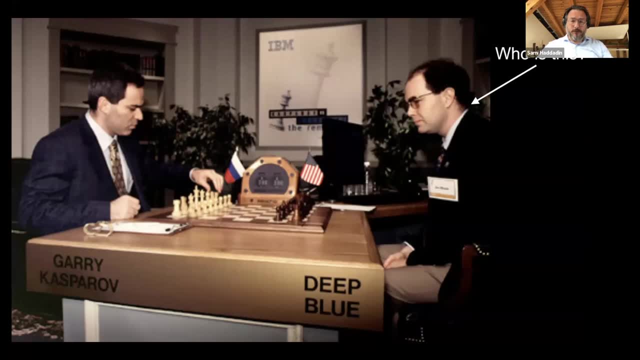 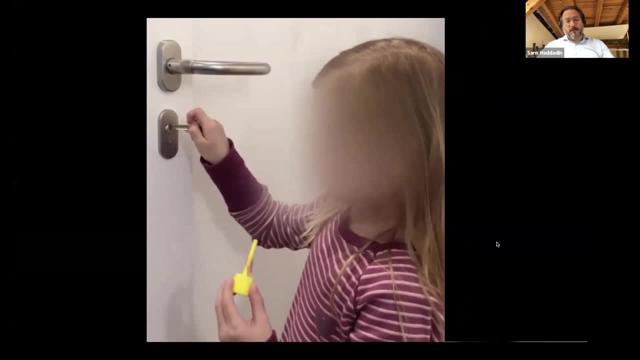 despite all the tremendous efforts and advances we have been seeing in AI, that there seems to be something that we are not entirely capturing. And if I look at the experiments I typically do with my kids- so I've got three kids and I always let them do all kinds of experiments- 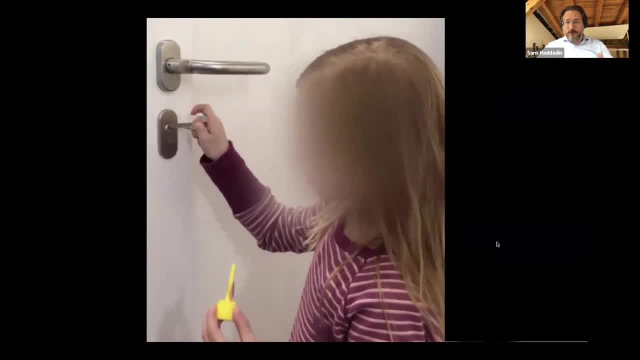 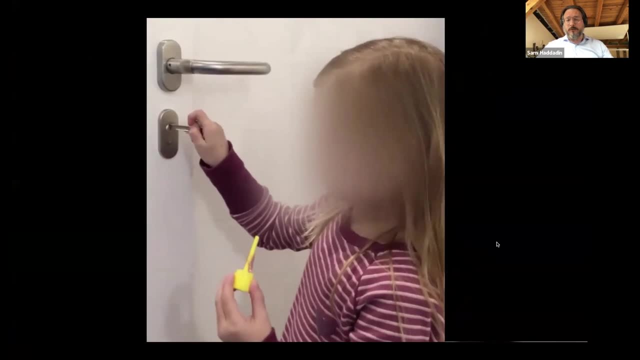 especially, I call them sensory mode experiments. So this is my eldest daughter, when she was around five years old And I was working on learning algorithms for robots. So I wanted to give robots the ability to grasp the world, interact with it. 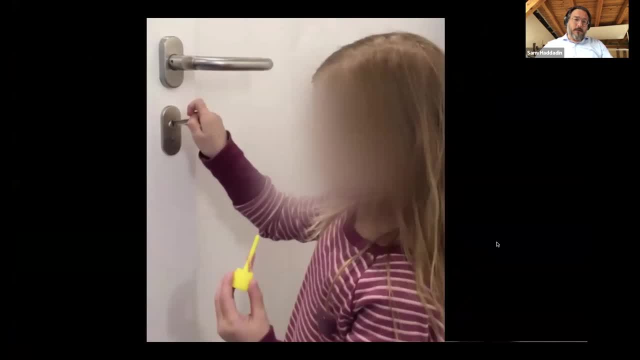 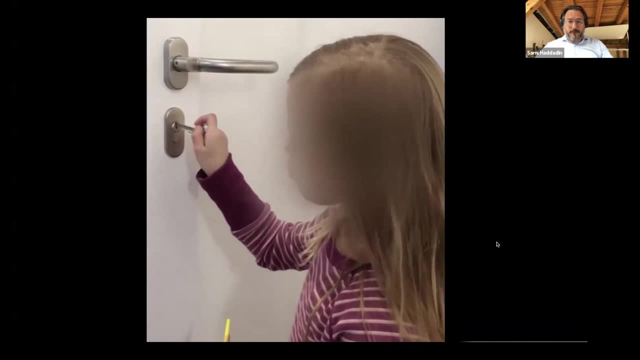 and really manipulate it. And I was thinking about what is a kind of challenging task, but not too challenging, so that I can really make some steps forward. And the great thing with kids is that they create kind of situations in which you can really kind of create a reproducible. 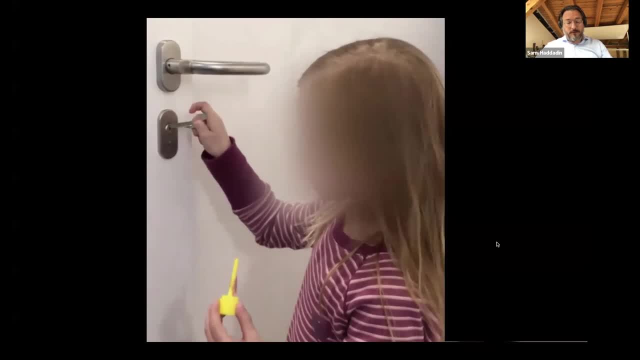 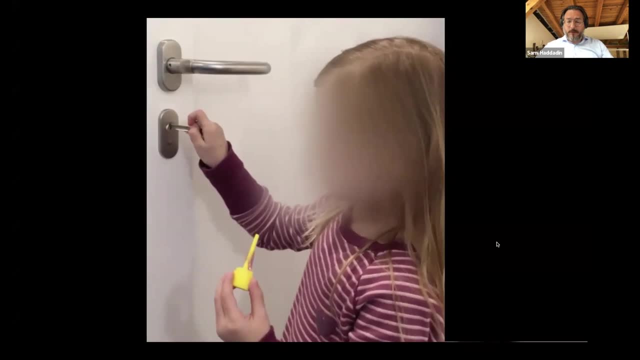 meaningful situations, meaning they basically make a big mess every day, right, So we all know that. But this also gives you the incentive to create some experiments. So I asked her when she was kind of making a big mess in our living room. 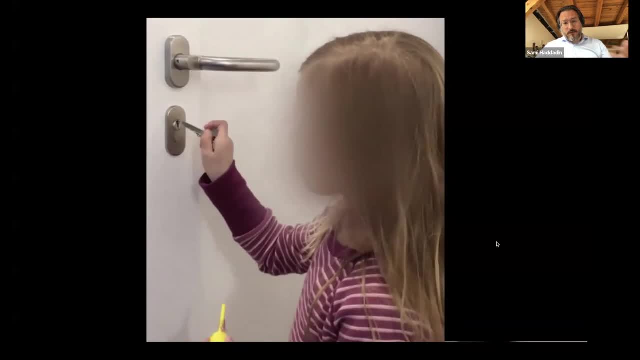 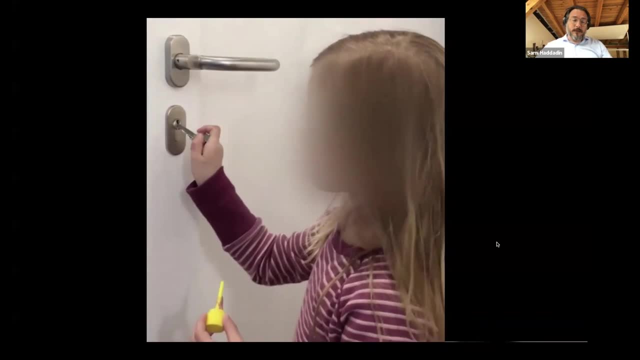 to get the key and open the door, And I gave her the task of doing this within less than 10 trials, And if she would have been successful she would need to clean up, So the incentive was set. in some sense, She was running to the door. 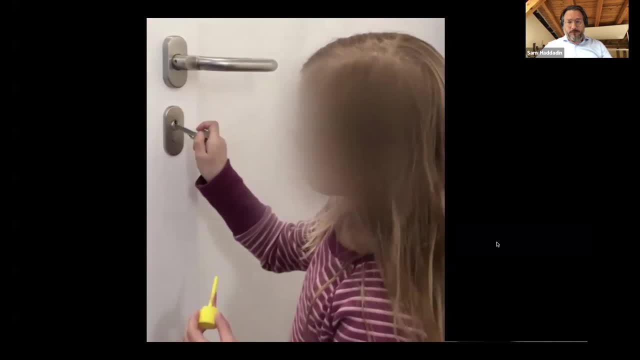 and I was kind of expecting two possible outcomes. Either it's so simple that she would be doing it immediately, or that she would not be able to do it at all. The result was kind of astonishing to me. It was only seven trials. 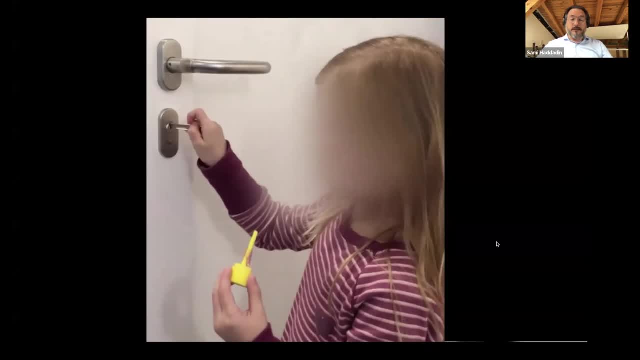 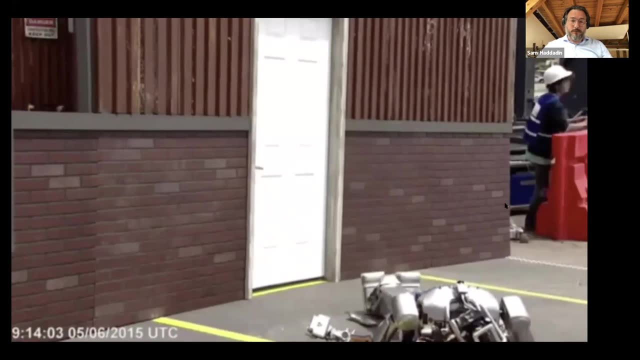 so obviously not a big data issue, but still seven trials, and she was already five years old. Around the same time, there was the so-called DARPA Robotics Challenge running, when some of the most prominent researchers gathered together close to LA and we basically tried to solve a challenge. 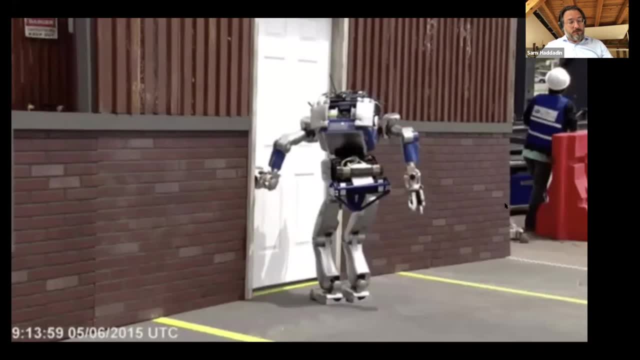 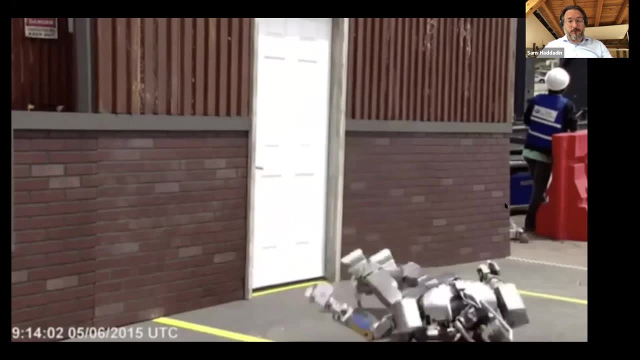 that my daughter was able to do at the age of five and in seven trials. However, the best robotic teams and the best robots in the world were not really able to do this on the same level, So there seems to be something that is here a bit different. 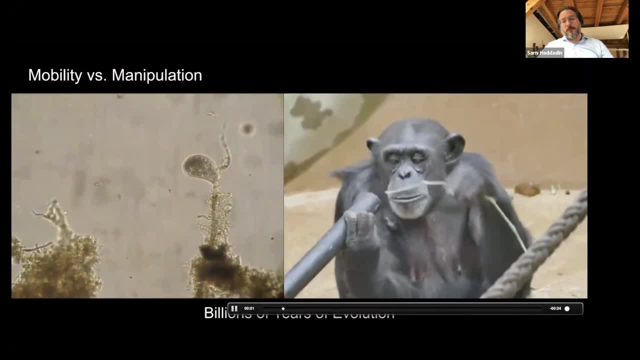 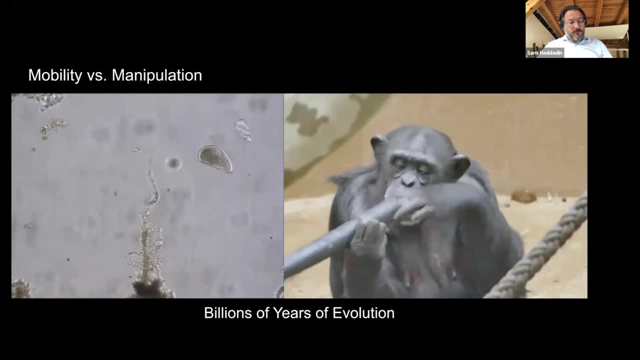 between humans and robots, And I just want to give you an analogy why this seems to be a very complex thing, And just by the concept of mobility and manipulation. So Martin was talking about mobility. so the autonomous driving assistance that helps you to stay in line while you're driving. 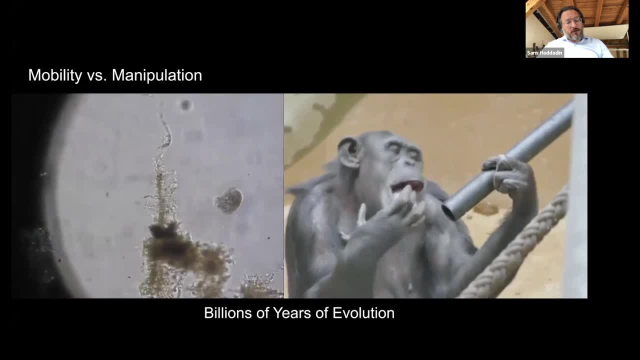 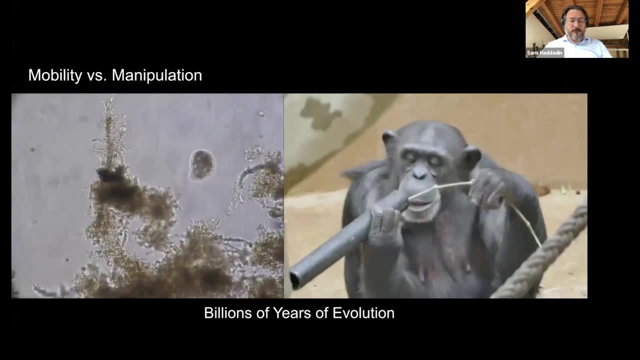 However, if you look at biological analogies, then it's kind of interesting that the concept of mobility- so moving from A to B without colliding with the world- is something that already single-cell organisms have developed billions of years ago. So there seems to be a very simple ability. 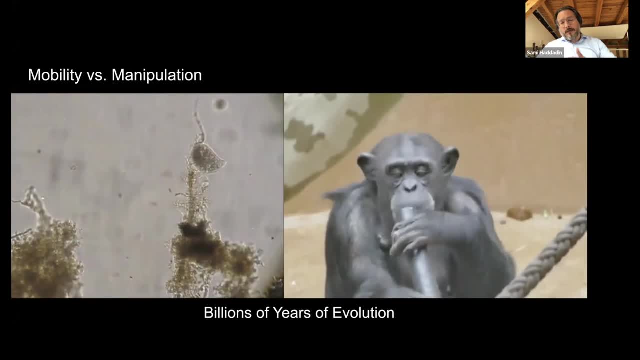 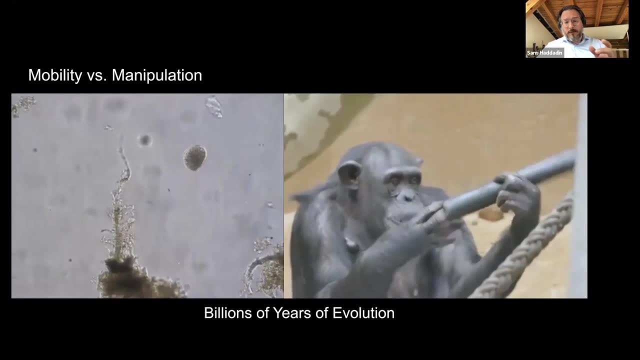 to execute from biological perspectives. At the same time, the concept of manipulation, so using the tool hand grasping the world, manipulating it, interacting with it- seems to be something that really took billions of years of evolution and only primates are able to do this. 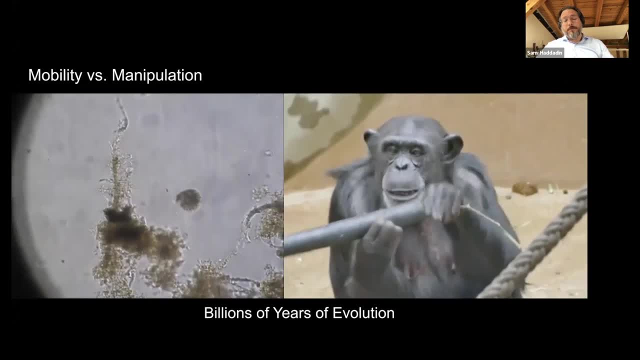 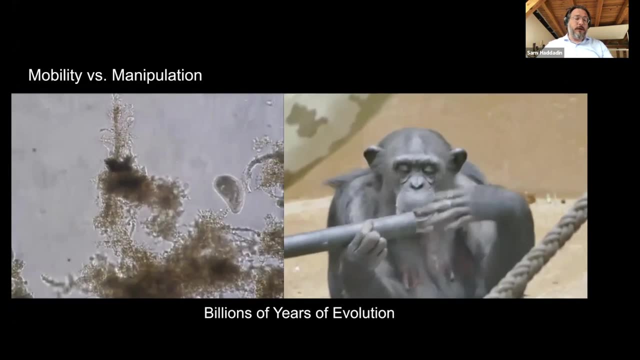 on that level of complexity And it seems to be the tool of our creativity, of our expression. also. the co-evolution of hands and the brain are kind of well-known concepts And it's kind of giving us a more humble perspective on the concept of manipulation. 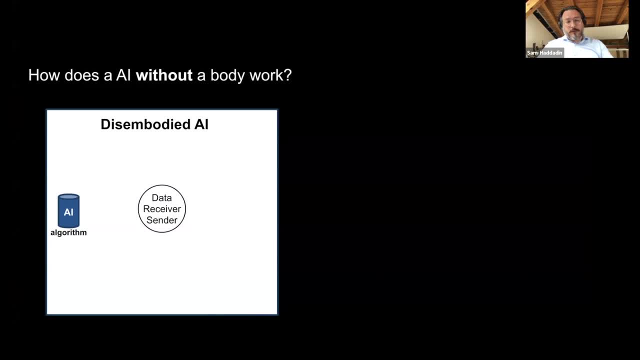 and the abilities that humans have on that level. And this brings me a little bit to this distinction about what AI is, what is embodied AI and what is really a robot- A little bit what Jeanette was referring to, or I think no, Martin was doing that. 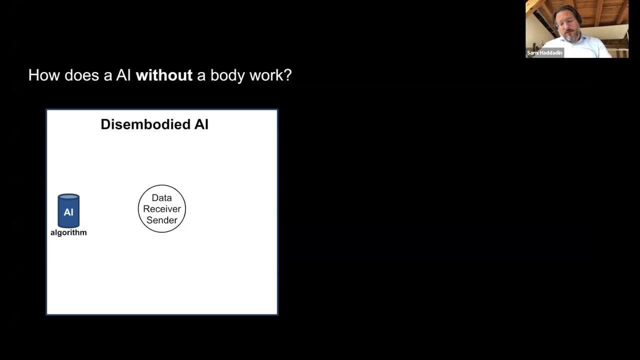 So, when we look at the famous systems, we all know, then the concept of disembodied AI. so a body without an AI is essentially consisting of a data receiver-sender system that receives data, sends it to an algorithm and then does the processing. 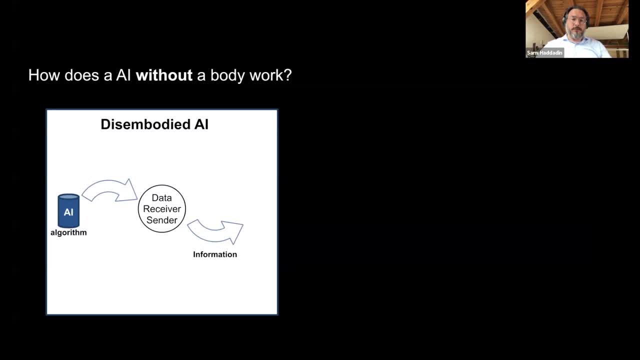 in order to give you some information back. If we go on the real world, then obviously we all know these devices, like Alex and other personal assistants. they essentially record the data, the speech data. we send it into the cloud, that the algorithm computes some results. 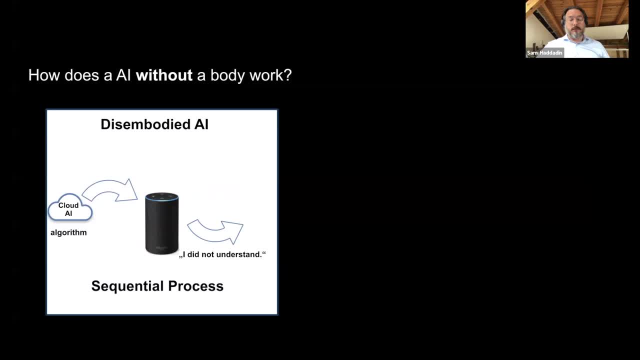 and then, in this sequential process, we actually get the feedback, the result of this process. So it's a purely sequential question and answer process in terms of systemic responses. However, if we go to the real world and physical interaction, the difference in what we call embodied AI, 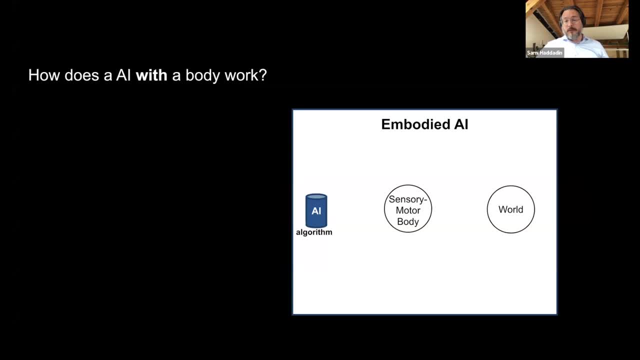 so artificial intelligence with a body is essentially that we don't only have a sending and response unit, but we actually have a so-called sensory motor body, And that sensory motor body is not only interacting with the world via data, but also via energy. 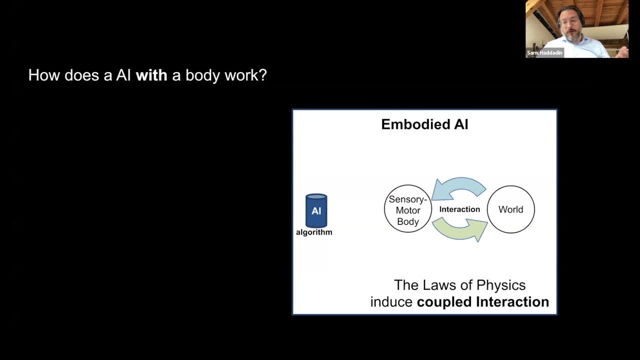 So action and reaction. Obviously, this is what we call the laws of physics. So the presence of a sensory motor body induces ultimately the concept of interaction, which is an action-reaction process, a systemic process as we call it. And obviously, if the body is interacting, 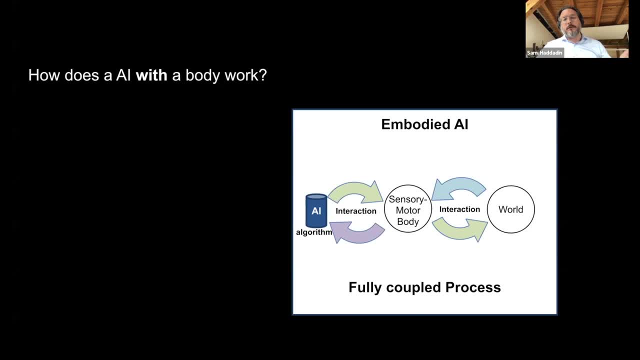 with the world, then the AI algorithm has also to interact with the sensory motor body. So we are talking about fully coupled processes, from the algorithmic to the sensory motor body, to the world that this agent, as we call it, interacts, And when we look at it. 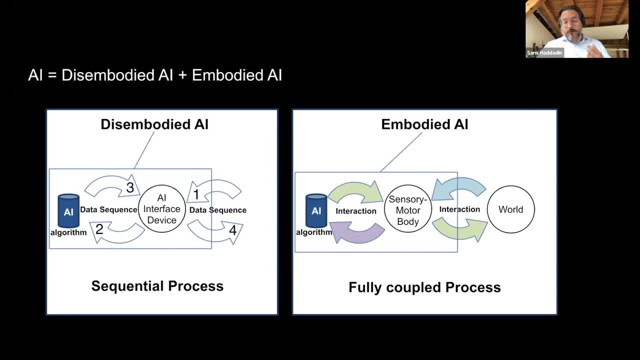 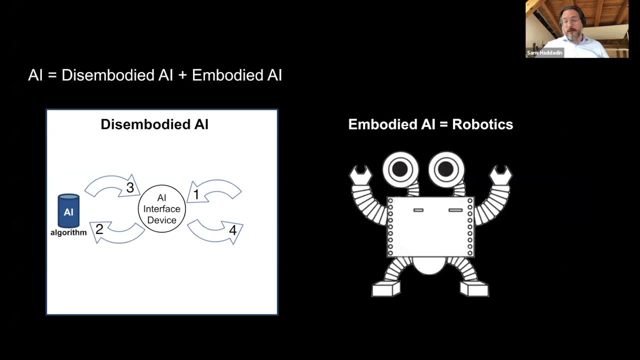 then, obviously, the sequential process is something that is much, much, much easier than the fully coupled process that we see in the embodied AI discipline And, obviously, since embodied AI is a very interesting field, essentially one of the nicest representations of AI systems with the body. 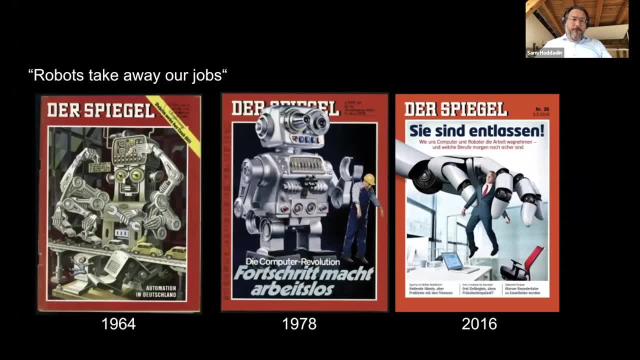 is what we call robotic systems, All right. However, if we talk about robots, then we all know, also from the poll- we are going to lose all our jobs. So this is the famous Spiegel. It's kind of our weekly magazine. 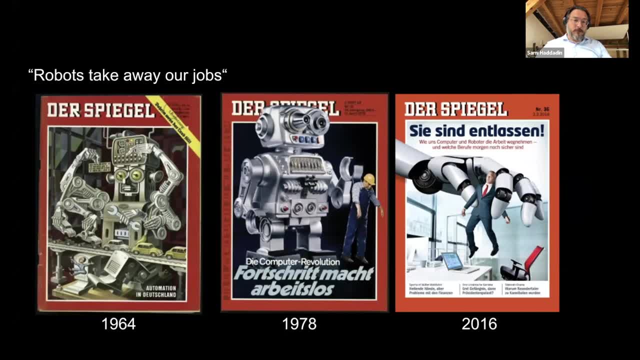 that is kind of famous in Germany And I think it's also internationally a little bit known. So if you look at the cover stories in 1964, 1978 and 2016,. it was always the robots that were kind of responsible. 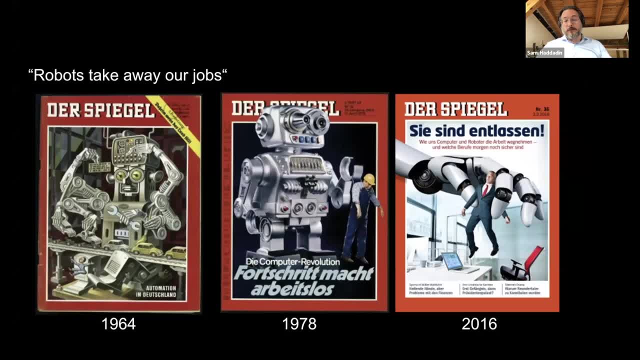 for taking away our jobs In 1964, automation in Germany In 1978, the computer revolution. However, we see a robot here In 2016,. you are fired, The robot's hand grasping you. However, it's not only the typical jobs in manufacturing. 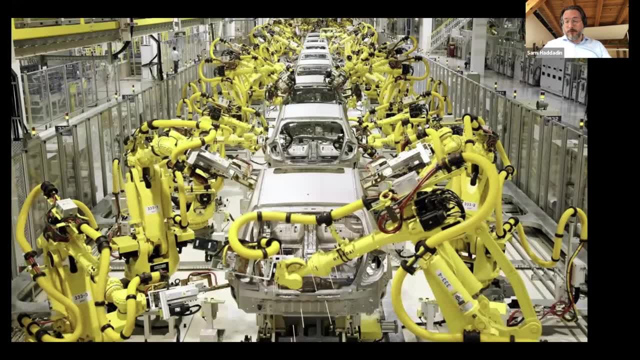 However, if we talk about this, then we should also ask the question: where are all these robots that we're talking about? Interestingly, most of the robots that we see so far are behind fences. They are doing spot welding and painting. Humans are only very seldomly close. 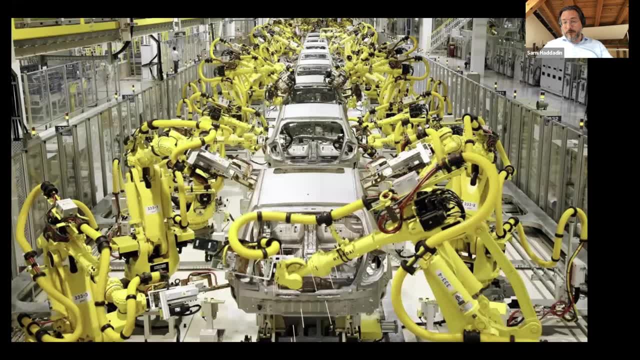 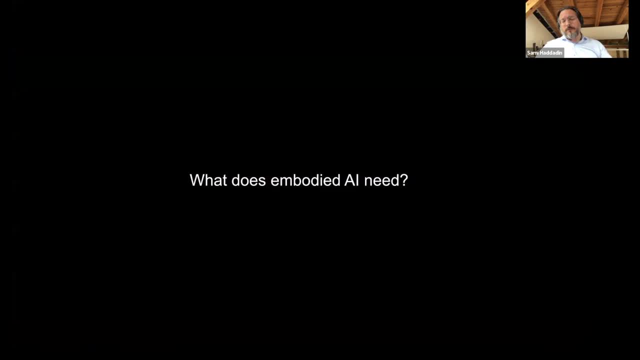 However, they are always kind of segregated from the robots by a safety fence, especially if we talk about these heavy positioning machines that barely have any kind of intelligence. So these are obviously not embodied AI systems. So what does an embodied AI really need? 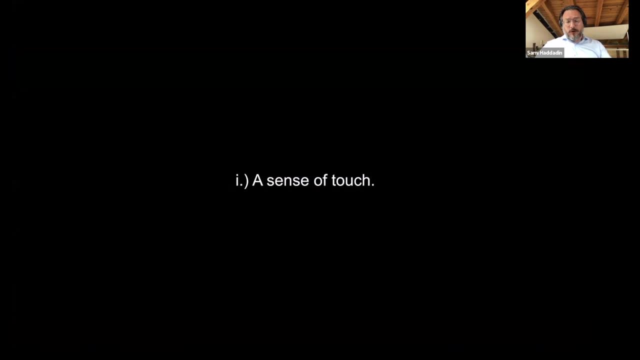 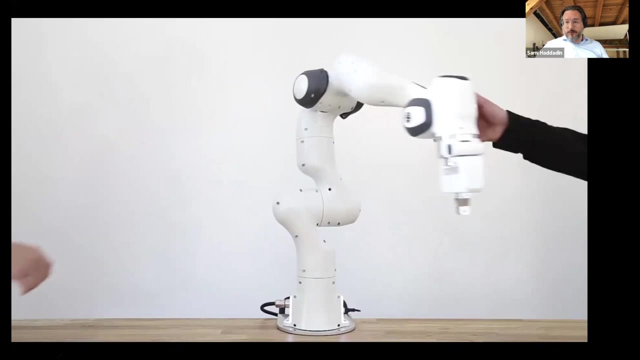 We talked about interaction, not only motion, So obviously we need a sense of touch. This is one of the most crucial things that you need in order to develop a system that is able to interact with the world that can be taken by the hand. 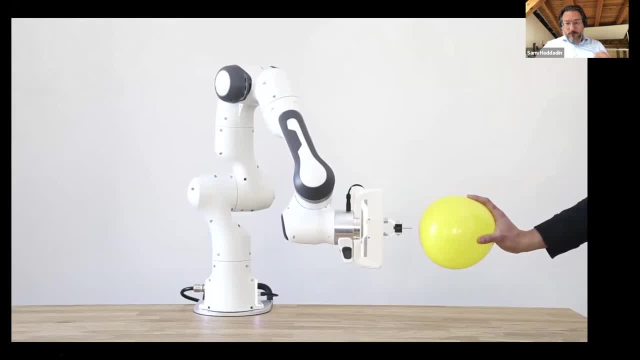 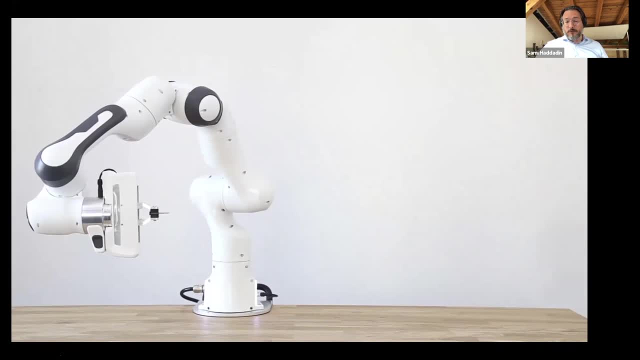 that is safe in its interaction with the world. So you see here a robot with a nail in its hands, And it's so sensitive that within milliseconds- in fact, 60 times faster than a human can do- it is able to detect and respond with reflexes. 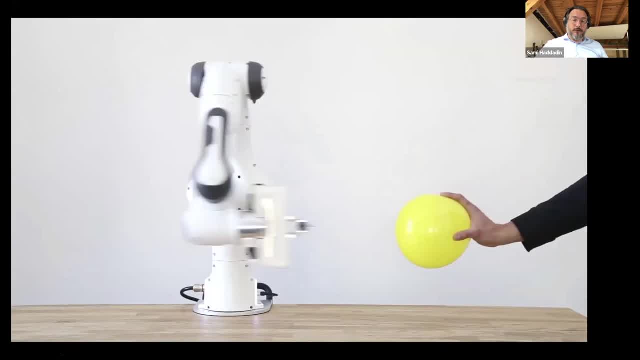 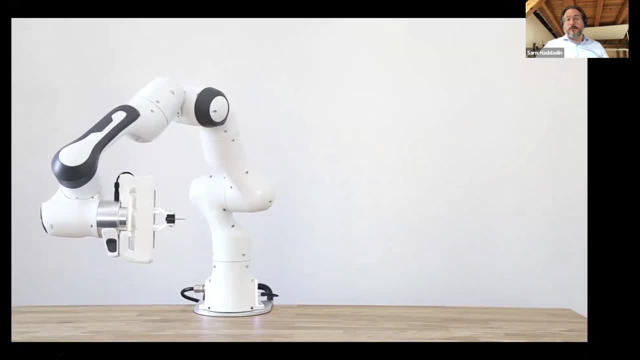 similar to what humans have to a potential collision with the environment. So Isaac Asimov's first law: a robot may not injure a human being, implemented in real physical robots, something that has not been possible so far, for a long time. 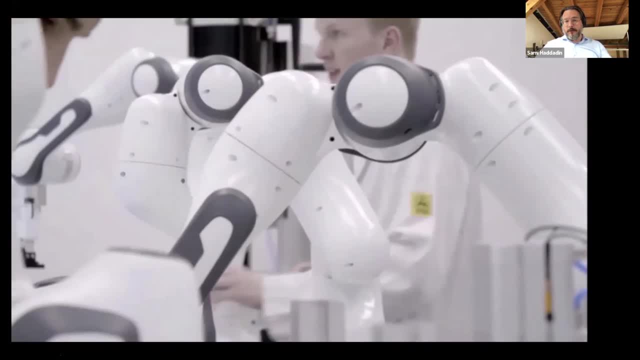 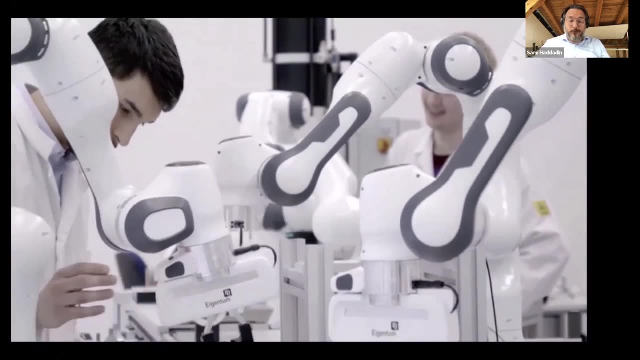 And these robots now can work alongside humans, So they're not segregated anymore from humans, but they are becoming partners, They are becoming tools. So the hammer of tomorrow- you could say nowadays today- is the robot that you can teach, that you can show something that's able to execute. 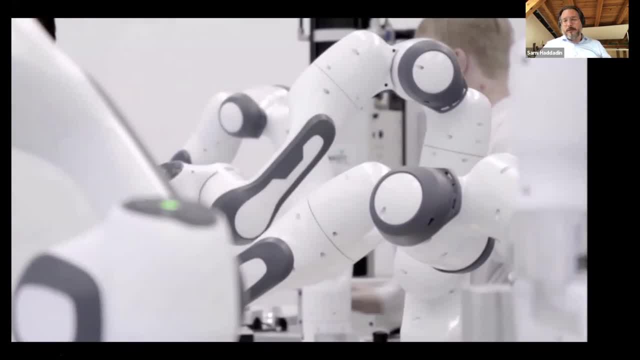 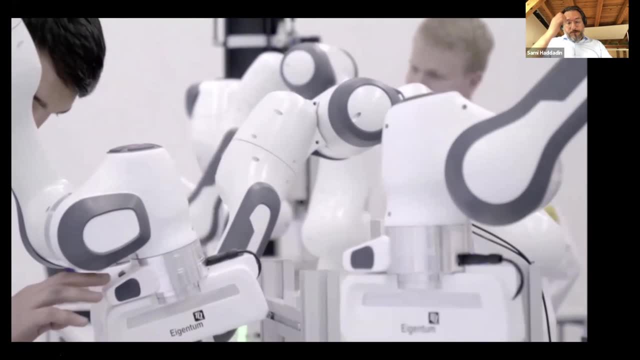 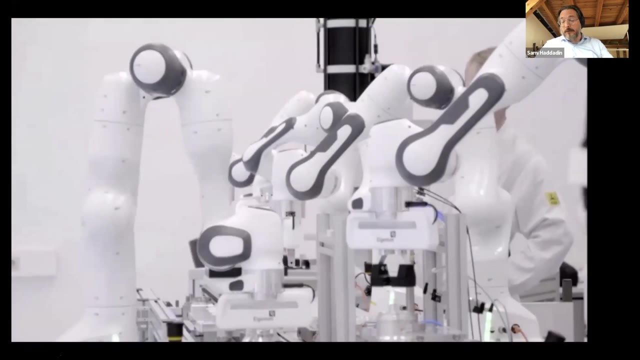 skillful, dexterous tasks that go beyond simplistic what we call positioning tasks, So they can help in assembly. They can actually make human workers be more effective. They can take over things that are done, that are dangerous, dull, and also things that really make us. 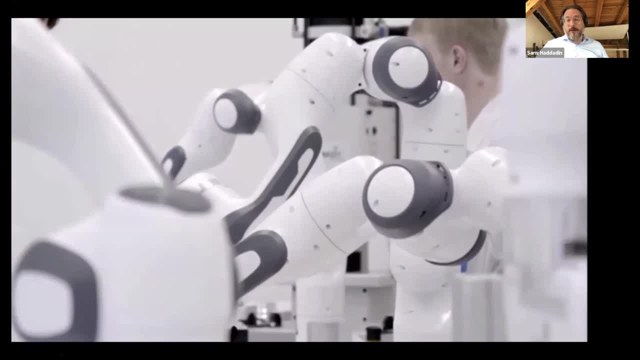 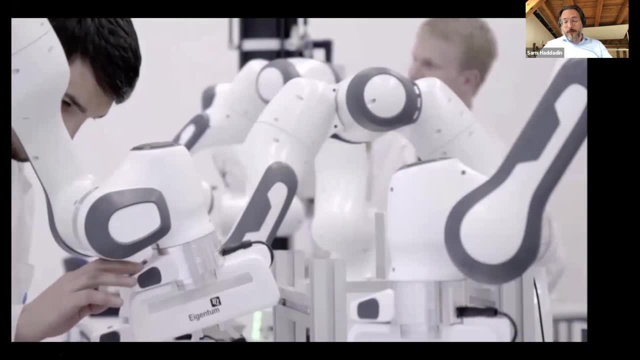 so they actually make us more effective in the way that we are being, that we are using these systems And, in particular, they are, by definition, still for many, many years a tool that kind of make the work that we're doing at the moment. 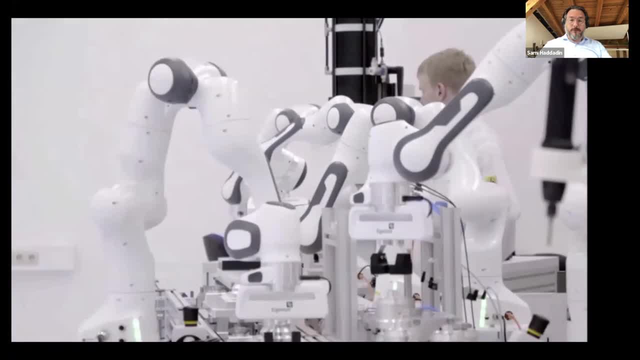 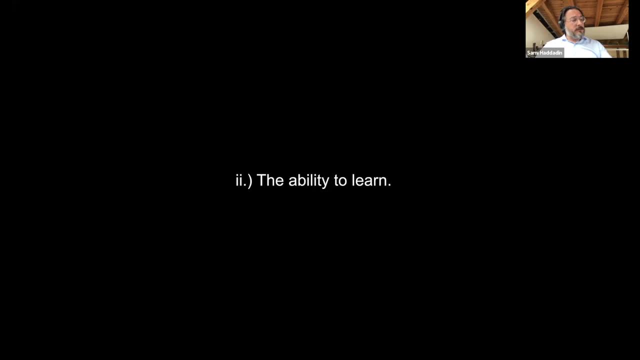 maybe even better than the work we've been doing before the years before. The second thing that these systems need is obviously the ability to learn, So machine learning AI is obviously highly related with the ability to learn. However, the ability of an embodied AI system, 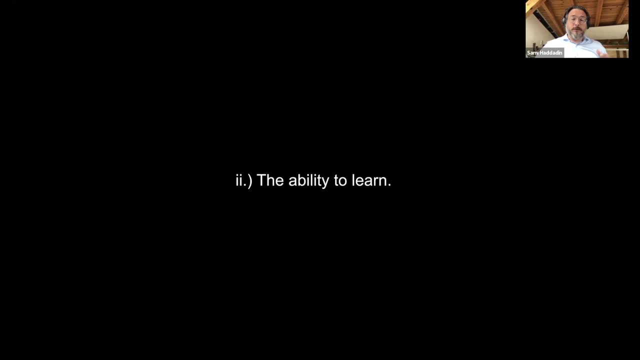 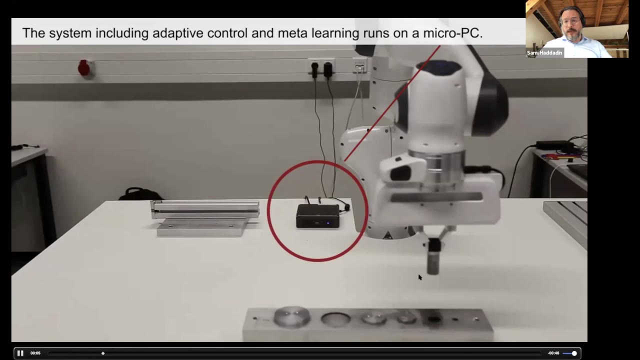 to learn is unfortunately a little bit more complex because of the systemic nature I was explaining. What you see here now is the first robot some years ago that we developed that was able to insert a peg into the hole, just with a very, very small PC. 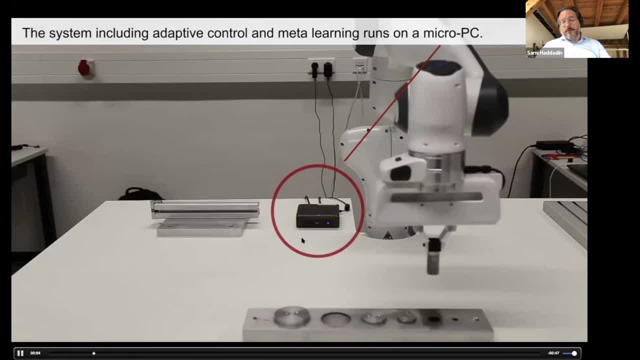 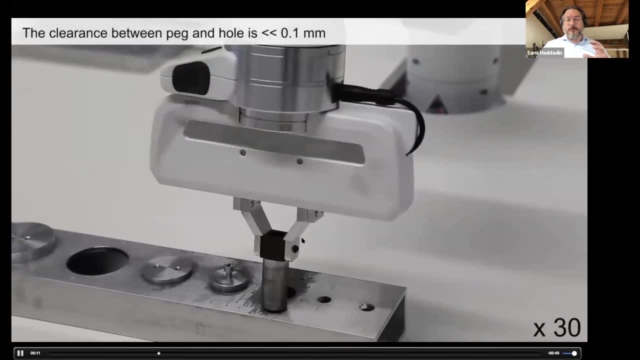 the one that you see here, just a 300 bucks PC that does the machine learning algorithms that are kind of inspired from the human, And we don't need big data algorithms anymore because we basically encode the knowledge that we understand from human and other primates. 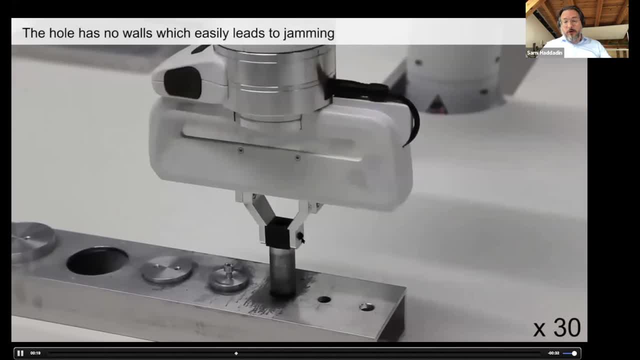 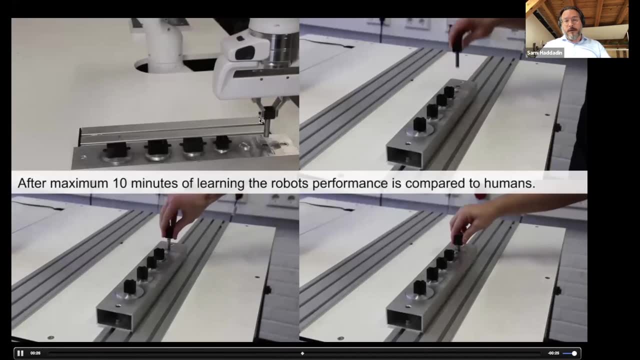 to be able to grasp and interact with the world and learn with highly efficient machine learning algorithms- kind of skillful tasks to a certain extent. And the interesting thing is if you compare this to grownups, so these are now three students of mine. 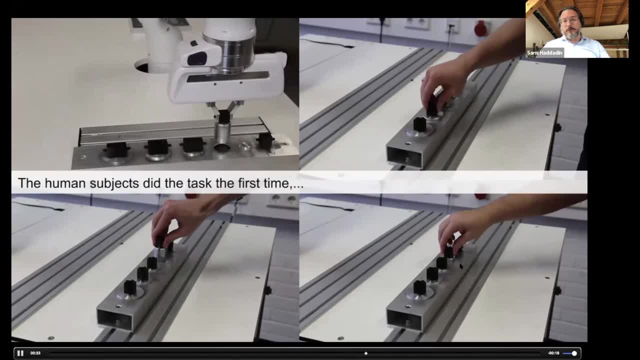 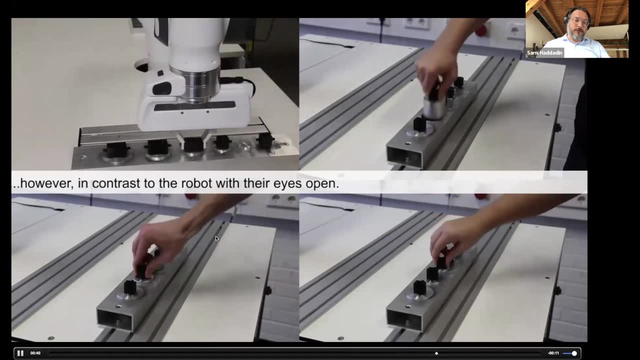 an ME student, a CS student and an electrical engineering student, and they all are able to do this, what we call insertion tasks. This is kind of a very famous reference problem we have in robotics called the peg and hole problem And interestingly they all are grownups. 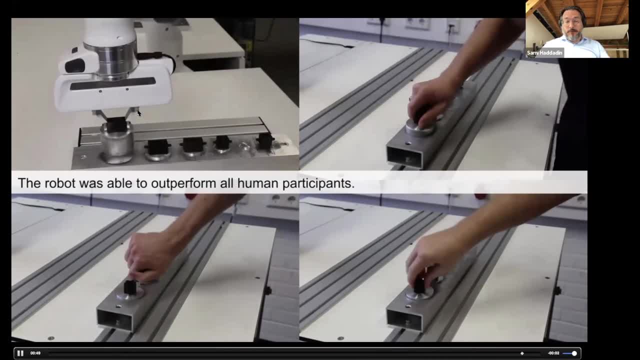 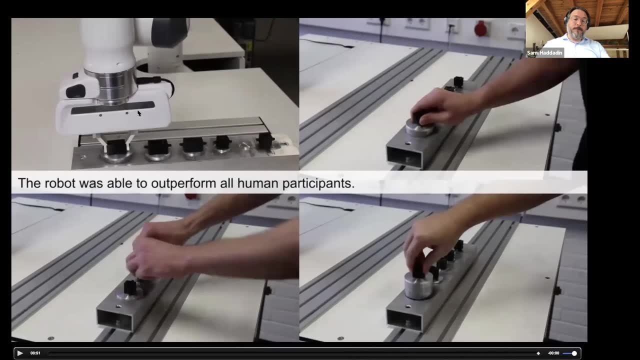 They have opened up their eyes. The robots on the upper left is actually blind, but it's able to execute the task at the same speed as a grownup. So it's not as we saw with my little daughter. However, how about the key into the hole? 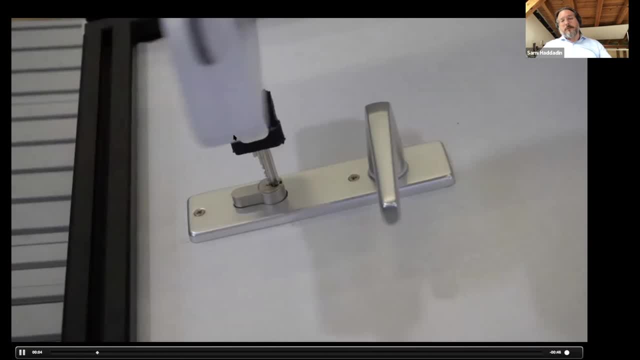 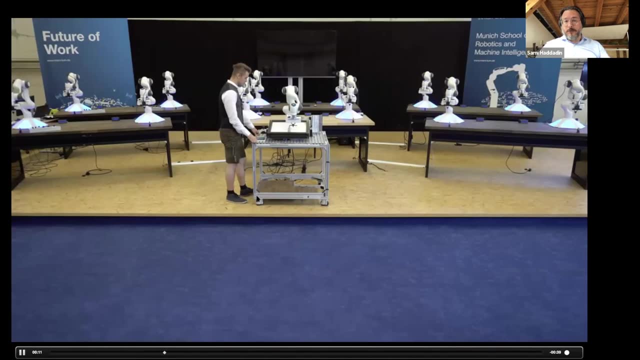 So let's see what happens if we do the key into the hole. And obviously the big question is: if I tell a newborn robot, please insert the key into the hole, then obviously that robot is not yet able to do it. However, one of the questions 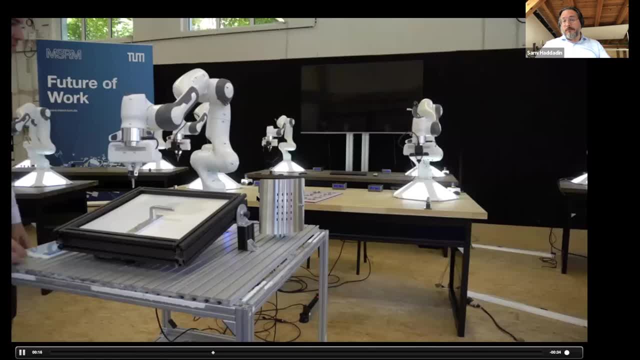 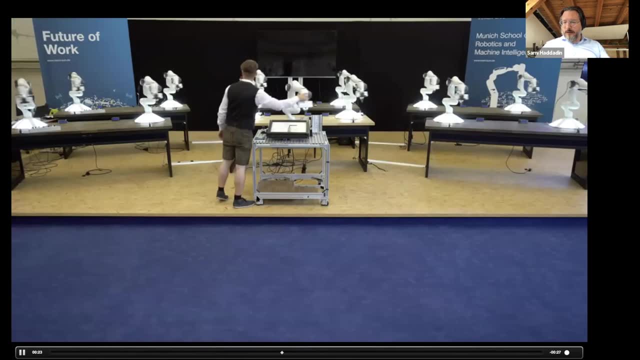 that we also ask is obviously, in a kind of society of digital and network technology as we are interacting today, the question could be what happens if we kind of network into, let these robots not only interact with us as humans, as our tool, but one human to end robots? 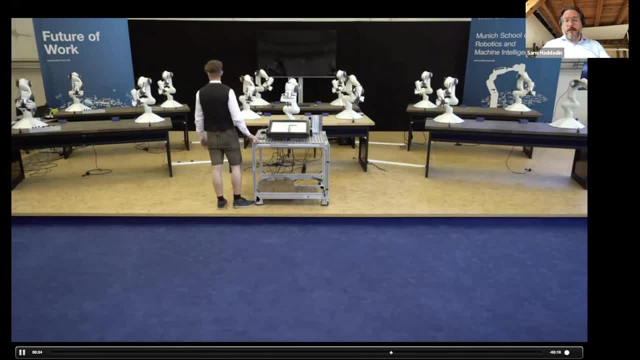 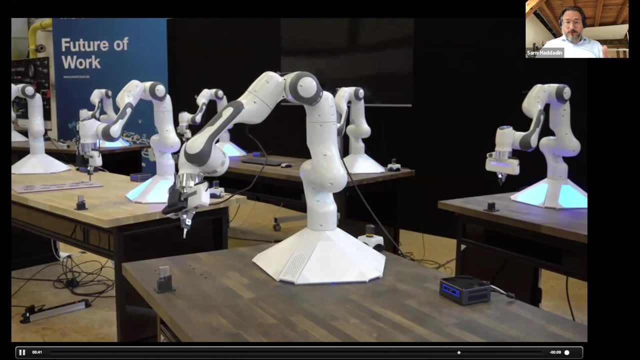 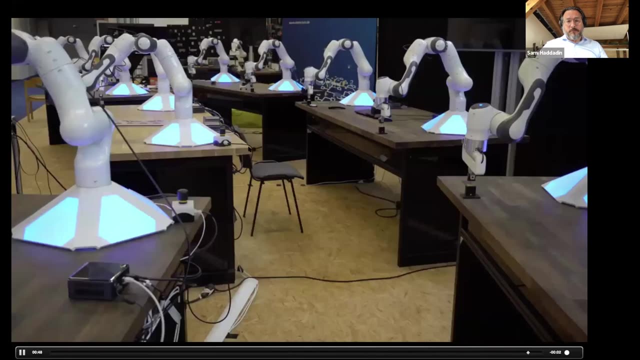 and let them tell, operate them all and interact and experience all kinds of diverse experiences. So they all do the different tasks with different keys. So they now try to learn multiple keys at the same time. But there's one thing that is special: They exchange the information simultaneously. 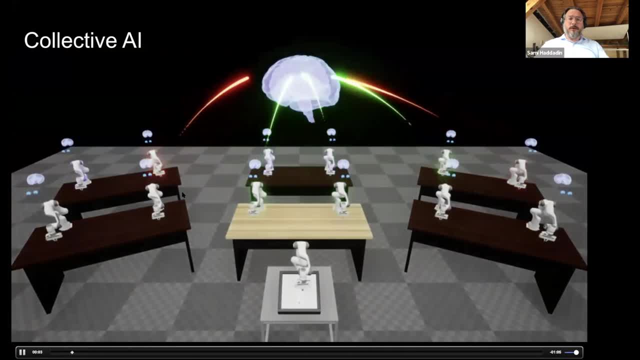 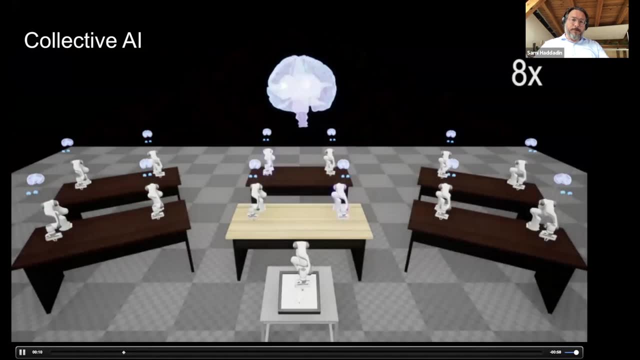 And now let us take a closer look to what we call digital twin of the system, That is, the collective AI of all of these robots. that kind of gathers all the information from the different robots and learns from failure and success how to intelligently and smoothly 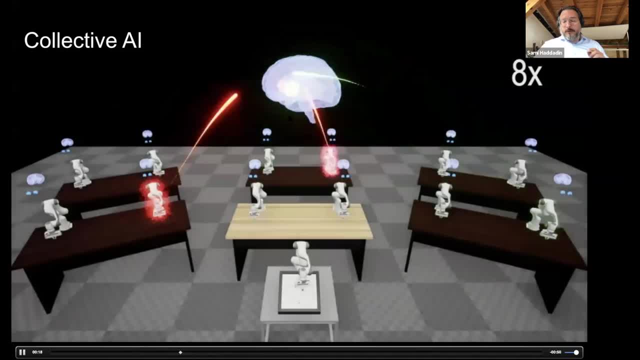 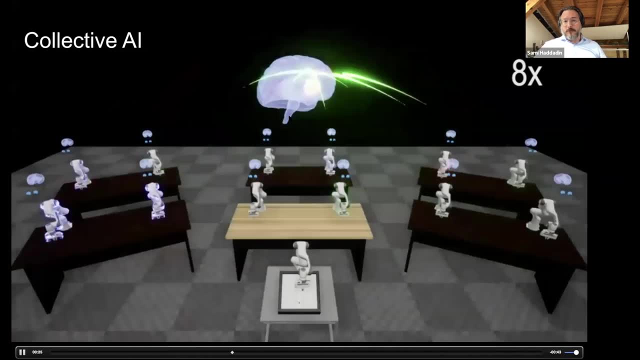 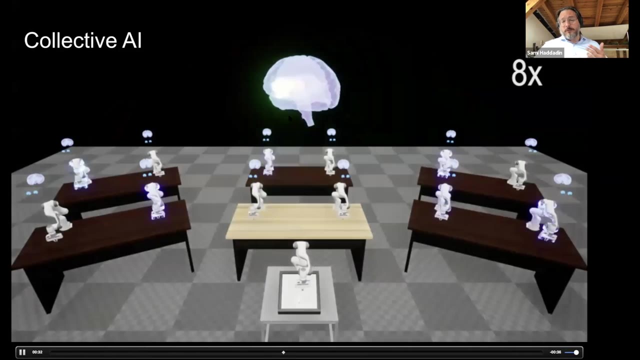 and nicely insert the key into the hole. Not in five years and seven trials, like my little daughter, but in fact it was already in the first trial when the system was successful, indeed. So by interconnecting and letting them exchange information instantaneously, these systems can actually speed up exponentially. 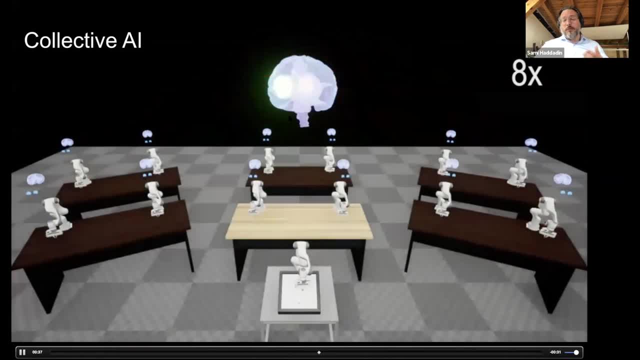 the information and the knowledge acquisition, compared to what single agent systems such as humans alone can do. So the concept of collaboration, interaction, is speeding up the concept of learning by exponential terms. Now these robots, essentially, have gathered this information of success and failure. send the information to the robot in the front. 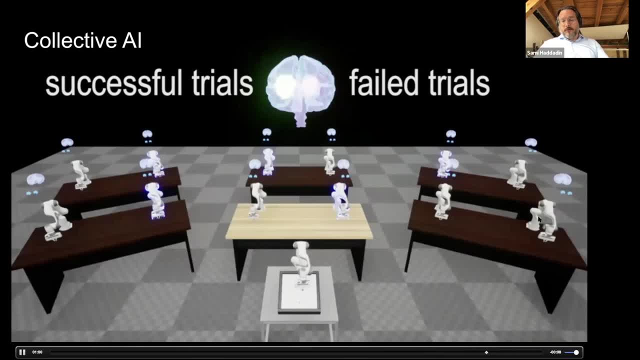 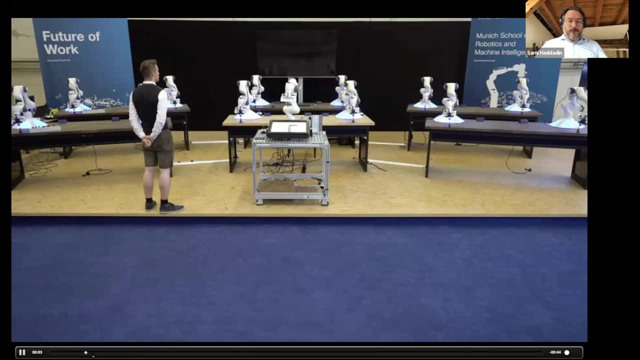 and that robot is now able to execute the task that we saw first. So, essentially, a newborn robotic system is able to do this immediately. So here we can see the real system. I'm going to speed up a little bit so that I don't run out of time. 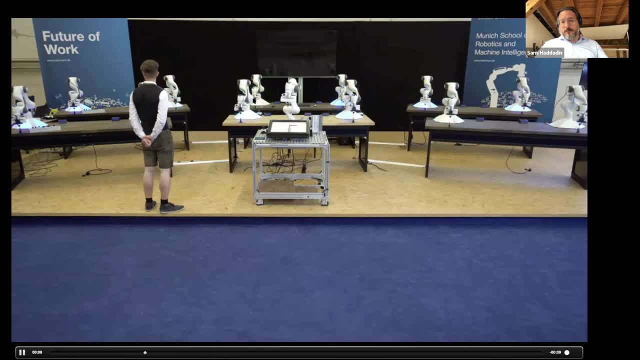 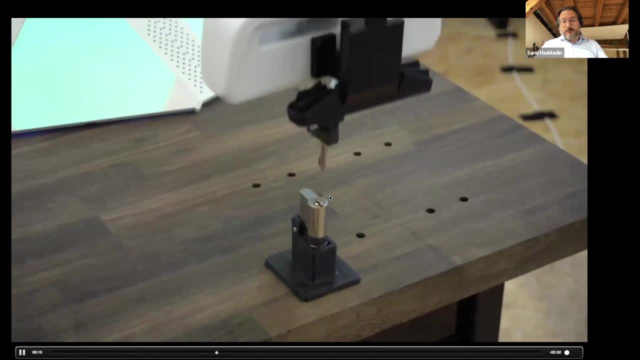 And you see already in the first place, some of the systems, the green ones, have been successful, And here you can see some successful trials of essentially newborn robots never having experience to interact with the world, able to take the key, insert it gently and be able to then gather that knowledge. 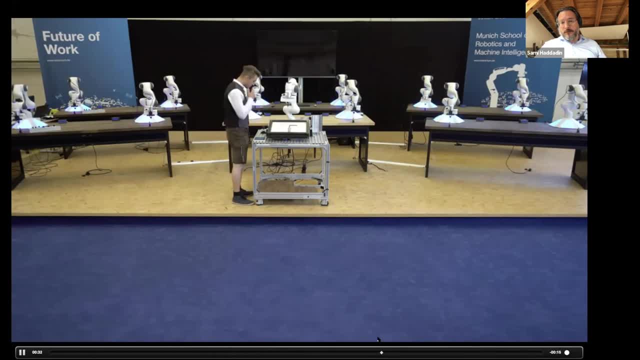 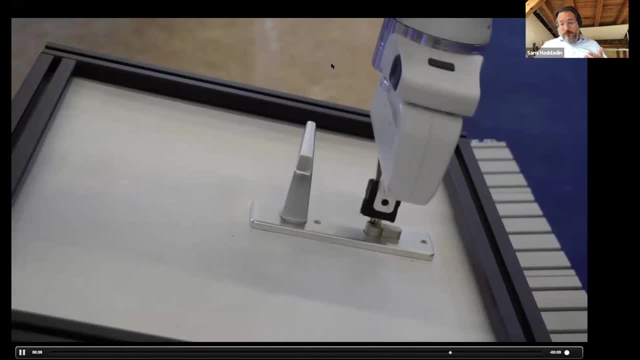 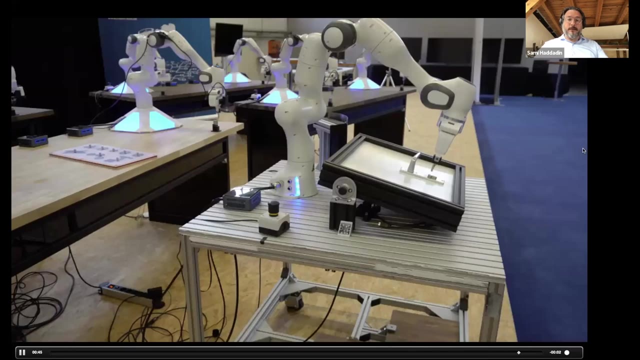 and send it to the robot in the front which you see here. that has not moved during the entire experiment. So the concept of collectivity, of collective learning, is able to learn, acquire information and skills exponentially faster than humans could do in principle. Obviously, these are still very basic skills. 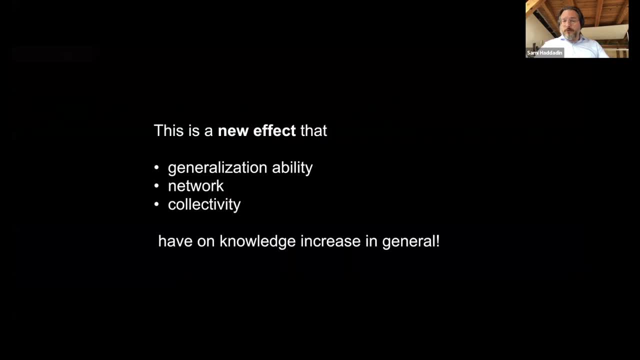 however, the concept, I think, becomes clear. So this is a fully new effect that shows generalization ability in learning. network and collectivity have on knowledge increase in general. So this is also kind of an explanation, I guess, for our network society, showing that just kind of. 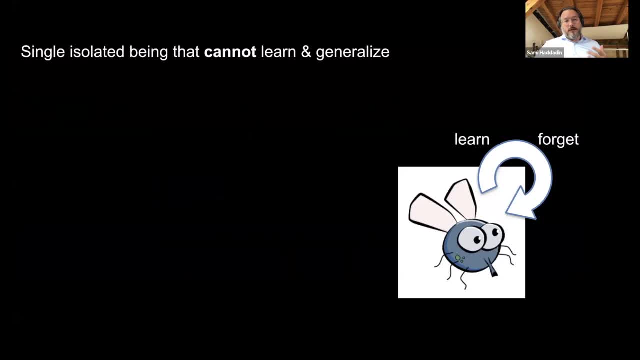 looking at the naive example of a single isolated being that cannot learn and generalize, So learns and forgets something. Let's do a very naive interpretation of what's going on here And let's take the goal of accomplishing 10 to the power of 5 tasks. 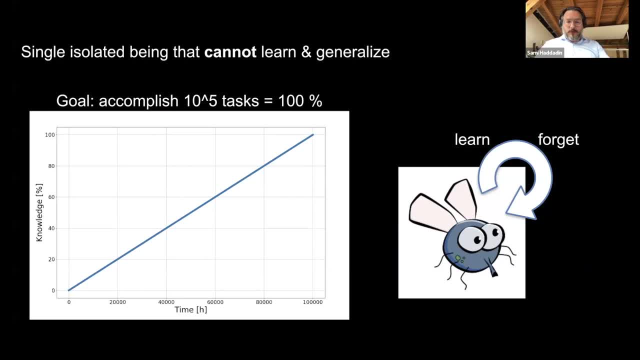 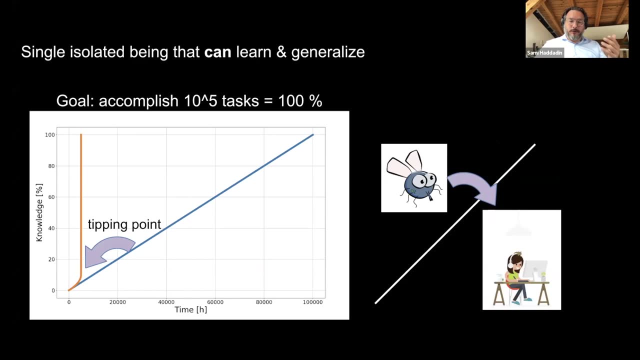 meaning 100%, And obviously such a system would need, if one task takes one hour, 100,000 hours Linear increase. That's, I guess, very clear. However, if we now take the human example, we learn from experience and we go faster, We become faster, we master certain tasks. 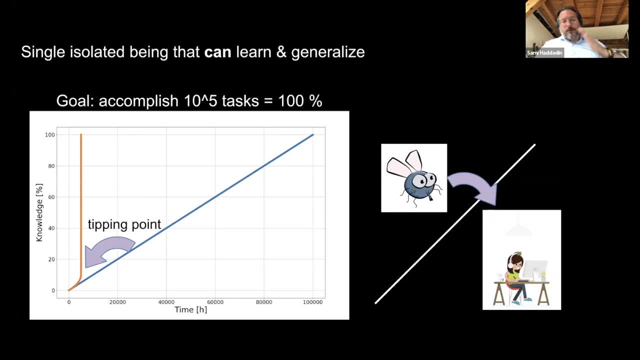 and then at some point we actually have a tipping point when the qualitative nature of the curve actually goes into this instantaneous acquisition of knowledge and skills. And if we now kind of zoom in there, then it's kind of interesting that there is really this qualitative nature. 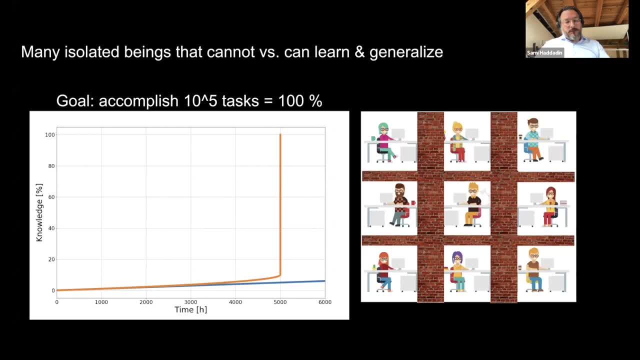 where, at some point, we master a task. However, what have we seen so far over the last years is we could parallelize, we could do big data computing and so on and so forth. And let's have a look what happens if we now let many agents, many robots, 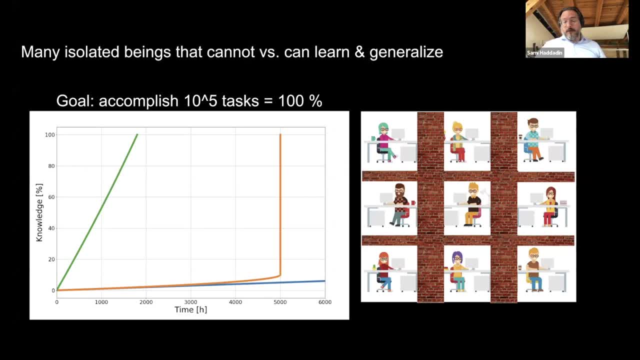 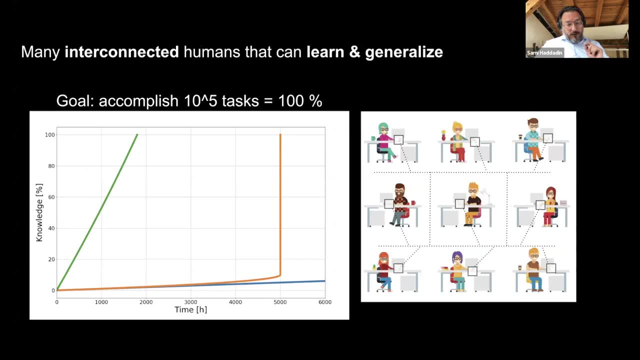 do the same thing. Interesting thing is, there is no qualitative interaction. There is actually just a linear increase. So what does this tell us? We need to network the people, We need to exchange information, We need to be generous in knowledge exchange. 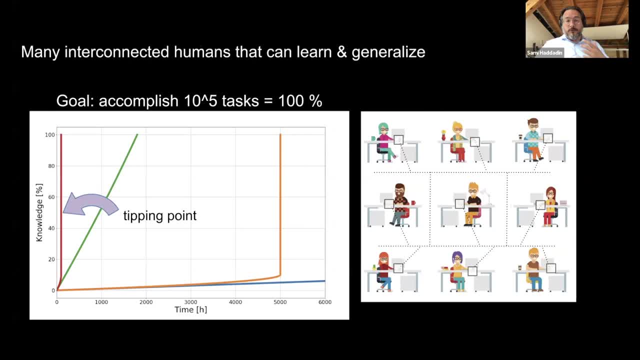 So essentially have a collectivity, to then again create a second tipping point. that really now is what I call the collective learning effect, And this boils down to all kinds of network systems. So, starting from the single cell organism that always has to learn and repeat, 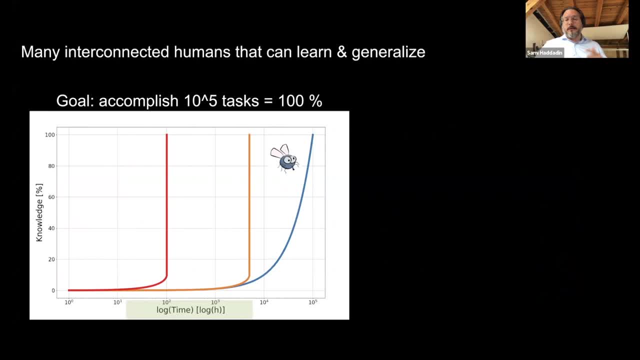 and obviously needs linear time in skill acquisition and in executing these tasks. to the polymath that needs a lifetime on a logarithmic scale to acquire 100% of the knowledge. to the collectivity of humans and machines that all together may be the solution to many of our problems today. 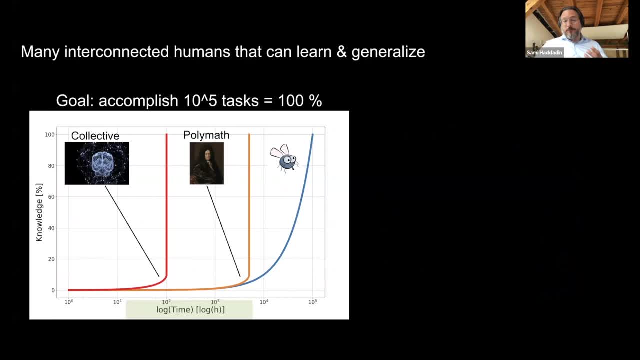 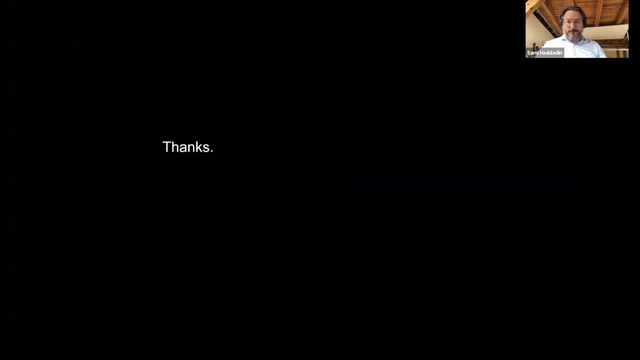 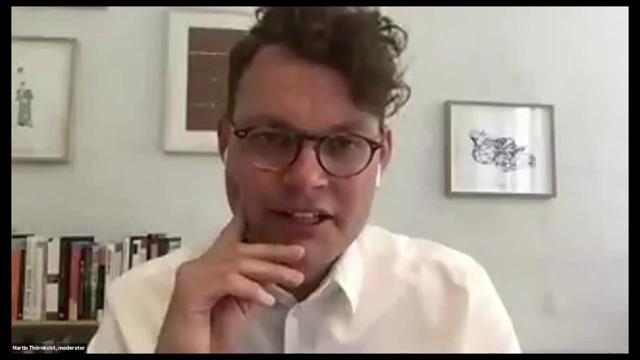 And I think, kind of showing that the interaction between humans and robots is the way to go for the future. Thank you very much. Thank you very much, Sami. Very, very good and interesting, And we will get back to you in a while for questions. 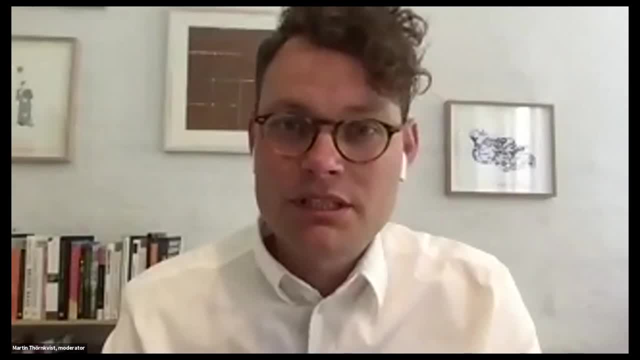 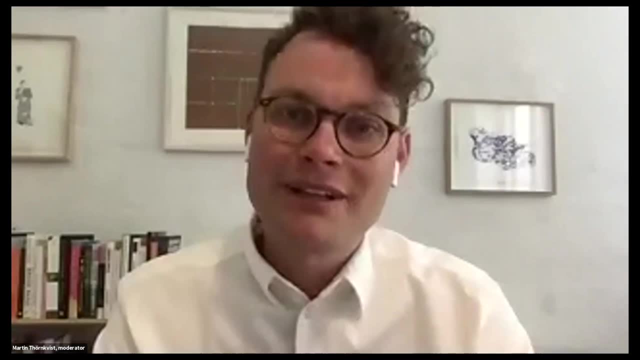 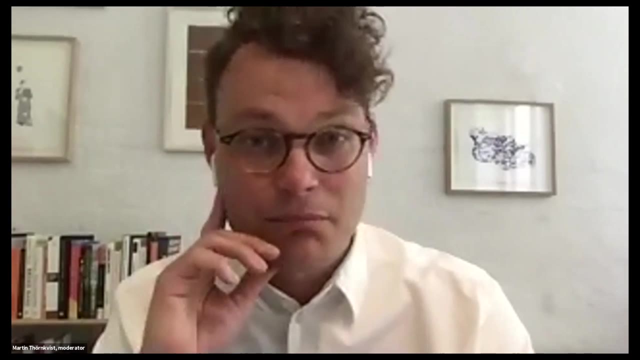 So to everybody following: please post questions in the chat That we can bring up in the end And keep the conversation going in parallel to the talks as well. Now we have our second speaker, So with us from outside of Boston, the USA, we have. 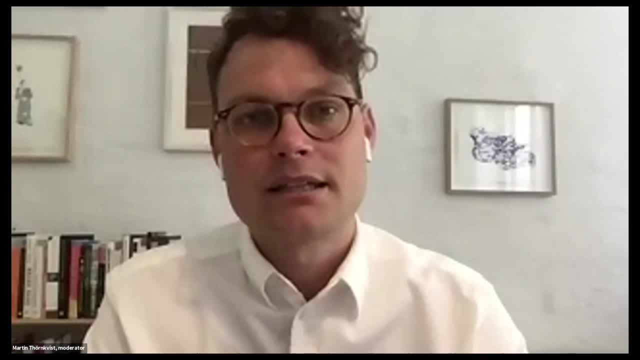 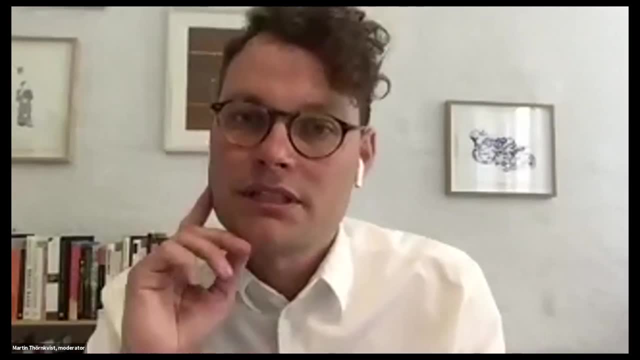 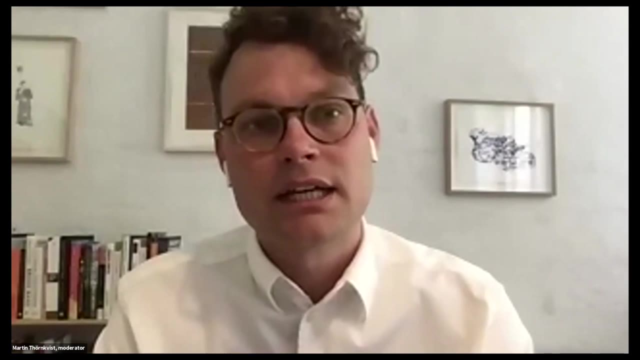 Dr Kate Darling. Kate is a research specialist at the MIT Media Lab, where she works on how technology intersects with society, with a particular interest in law, social and ethical issues. For us, she's going to dive deeper into what the ethical and societal effects of robotic technologies are. 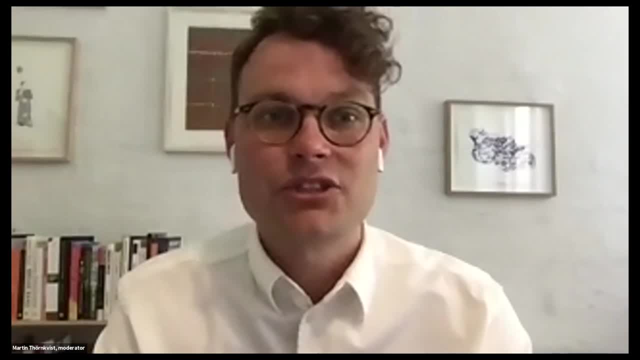 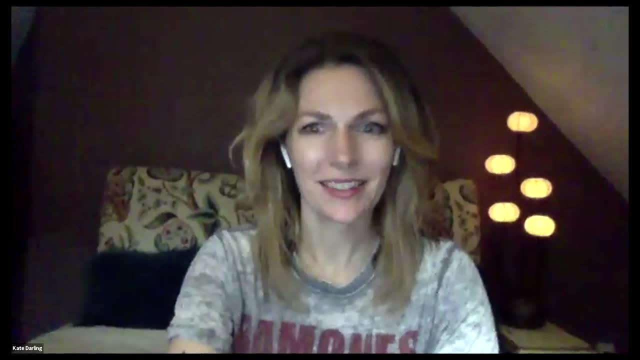 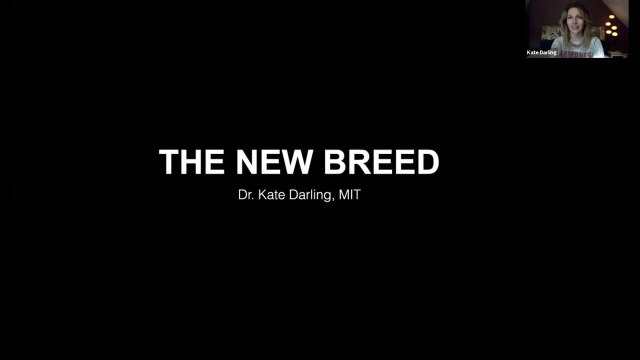 So please welcome Kate. Darling. The screen and microphone is yours. Hi, everyone, Just going to share my slides, Alright? So I really love robots. I love robots more than I love spiked lemonade, And I always have, And when I first started working in robotics labs, 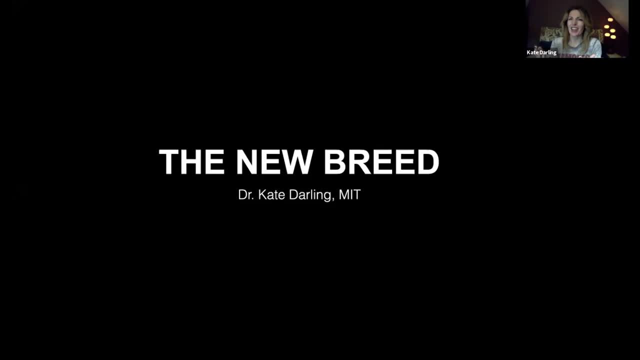 I was really excited to get to see kind of the cutting edge technology that's out there. I mean, people like Sami are doing amazing, very interesting work. But I also realized that if you go to these robotics labs expecting to find the robots that are about to take everyone's jobs, 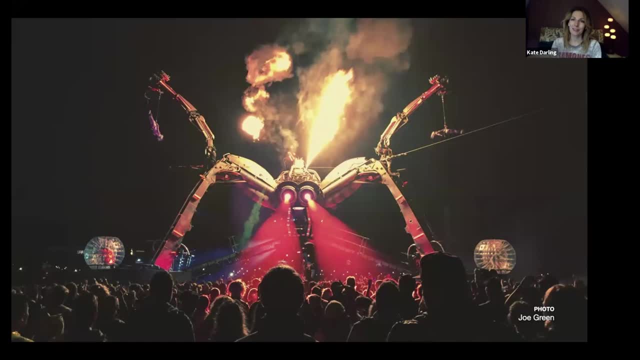 and about to take over the world, you're going to be pretty disappointed. So you know, as Sami showed, most of what our robots do right now is fall over. Maybe some of them can turn a key in a door, but I guarantee you that most of those, if you throw a bucket of water over them. 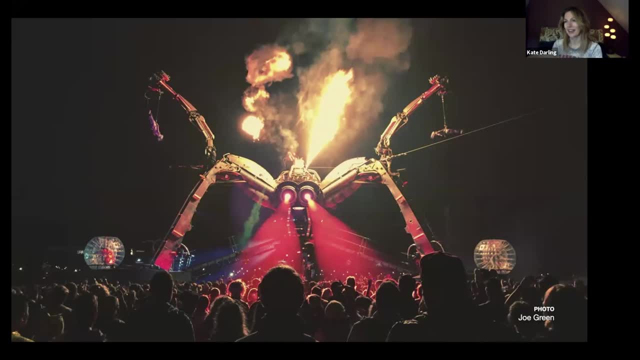 you'll be totally fine. Don't feel too threatened yet. So jobs and robot overlords are two questions that are on a lot of people's minds these days, but they're not the only questions and they're not the questions I'm most interested in. 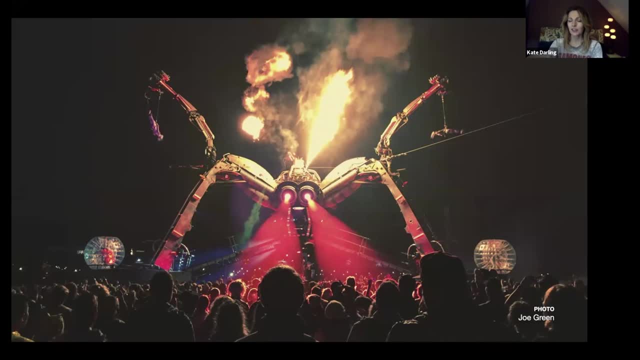 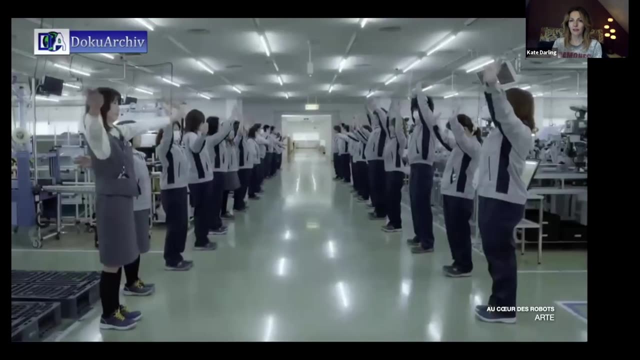 when we talk about robotics. So here's something that I think is fascinating. There is a Japanese manufacturing company that has people working in a factory and the people come in in the mornings and they warm up their bodies for their day on the assembly line by doing these exercises and 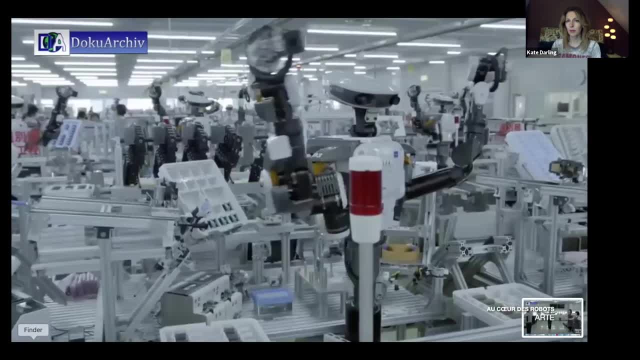 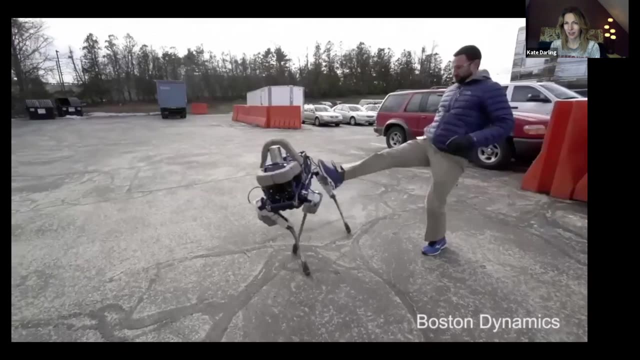 the company will have their robots do the exercises with the people in order to be perceived more like colleagues and less as machines. That's kind of weird. I also think it's really interesting that in 2015, when Boston Dynamics released this video of their robot spot, 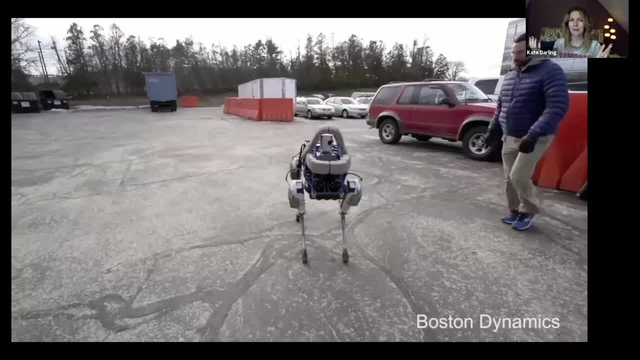 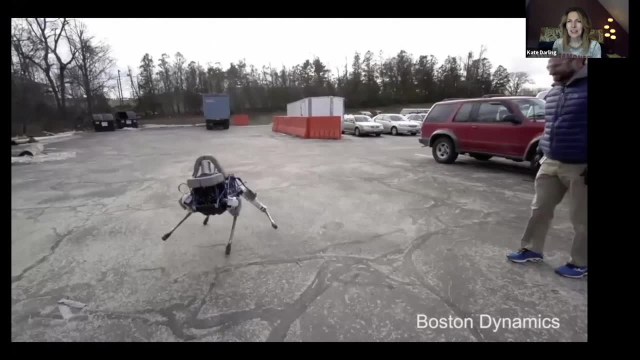 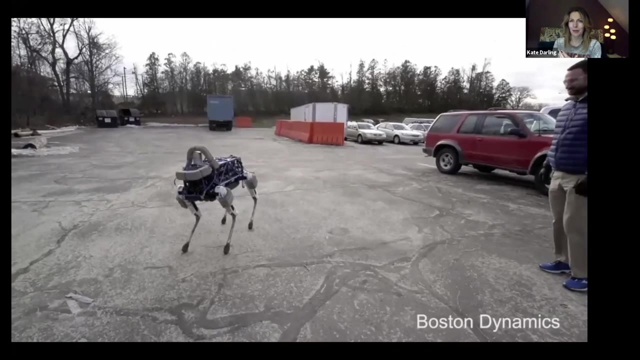 everyone in robotics said, oh my gosh, that's amazing. it didn't fall over and some normal people had more negative responses to what was happening in the video and it actually got to the point where there was so much attention around this that PETA, the animal rights 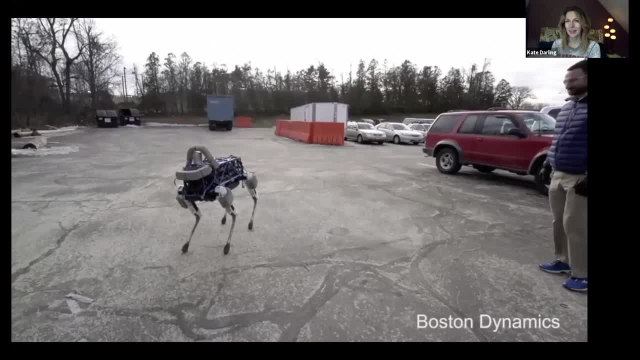 organization was getting so many phone calls that they had to issue a press statement and they didn't take it very seriously. they said: you know, it's not a real dog. but I think that there's something really interesting here, because what I think is interesting about how we're interacting with robots. 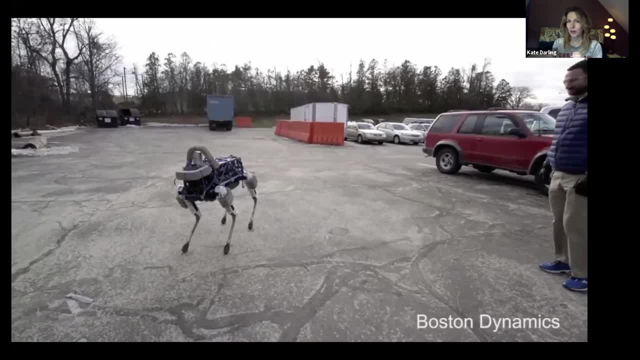 is that people, despite all knowledge to the contrary, will treat robots consciously or subconsciously kind of like living things. Now I was at a conference about a year ago getting a spiked lemonade at the bar and I met this guy. let's call him Scott. 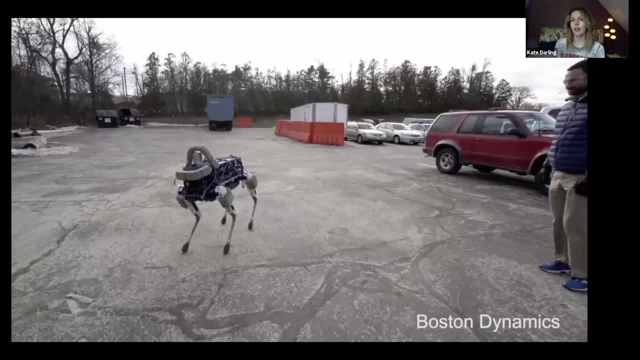 because that was his name, and he asked what I was interested in and I said I'm interested in the fact that, despite all knowledge to the contrary, people consciously or subconsciously treat robots like living things. and Scott said: nah, I don't buy it. We talked for a long time. 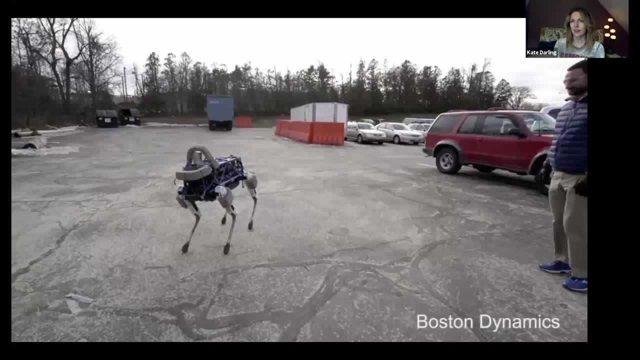 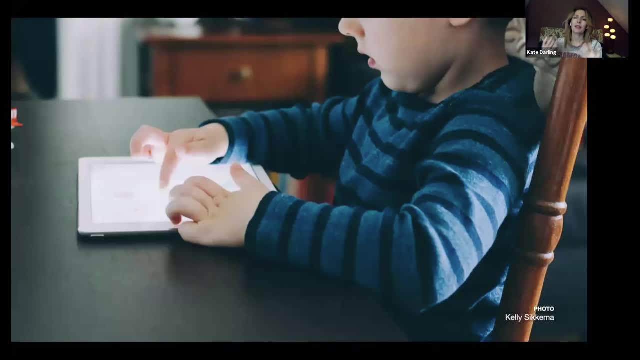 I couldn't convince him. Scott's position was: this is generational. you know, the new generation, as the Goethe Institute calls it, generation A, the devices all around them. maybe the silly people who grew up with Star Wars are primed to do stuff like this. treat robots like they're alive. 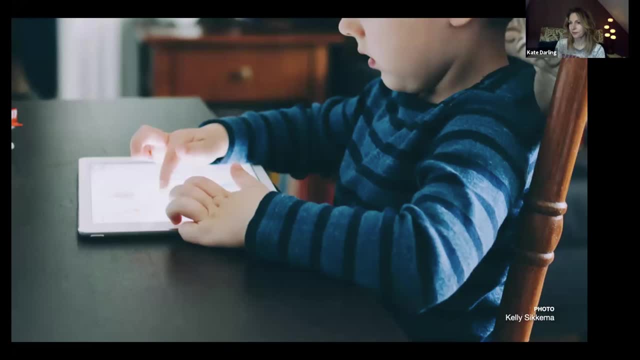 but the new generations, once robots are everywhere, are going to treat them just like any other device. and I couldn't convince him. so I think- yes, I think in part he's right, in part. we have this influence of science fiction and pop culture that primes us. we have the novelty of this technology. 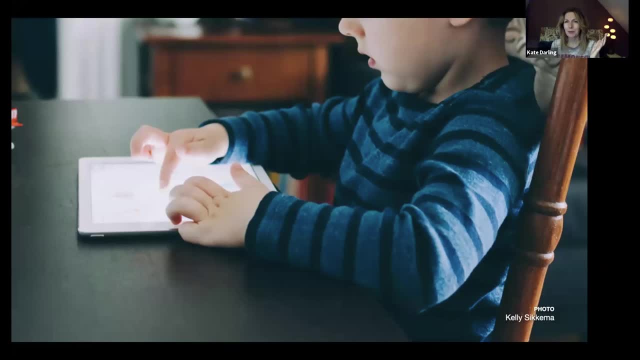 like when a hitchhiking robot got beat up five years ago and everyone was upset about that. maybe that was because of the novelty effect of never having seen a hitchhiking robot before, but there's also a part to this, to our perception of robots, that goes a little bit deeper than that. 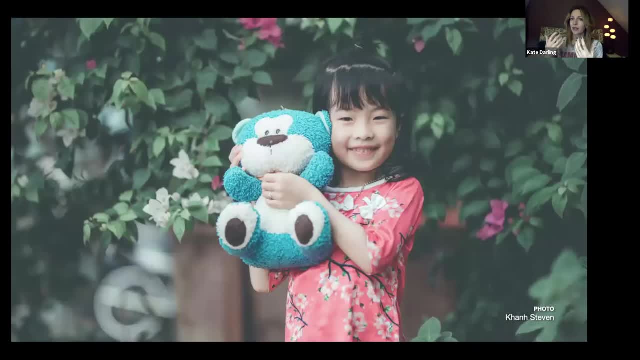 because we have this inherent tendency to anthropomorphize, to project human-like traits, qualities, behaviors onto non-humans. we do this to animals, we do this to objects, even stuffed animals. we do this from a very early age to make sense of the world around us. 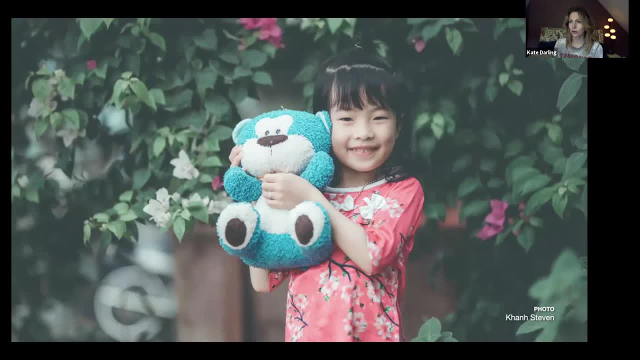 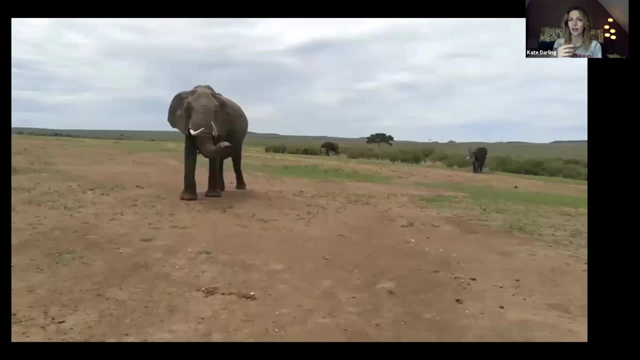 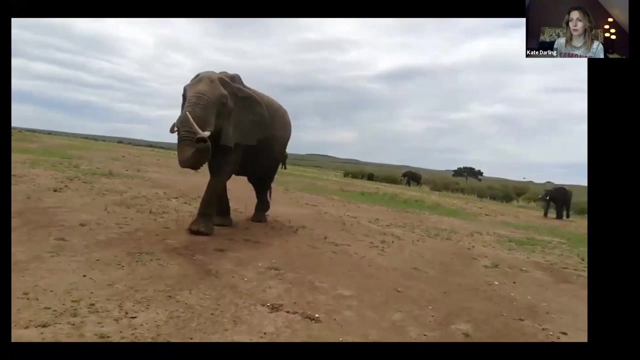 and interpret it, but also to relate to it, because we're very social creatures and another thing that we respond very strongly to in our brains is movement. so we are constantly scanning our environments and trying to separate things into objects and agents, and studies show that this evolutionarily 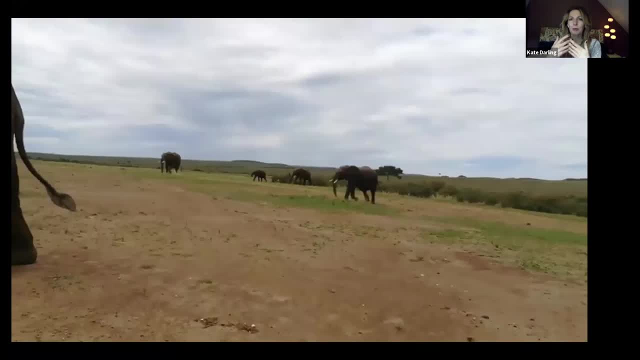 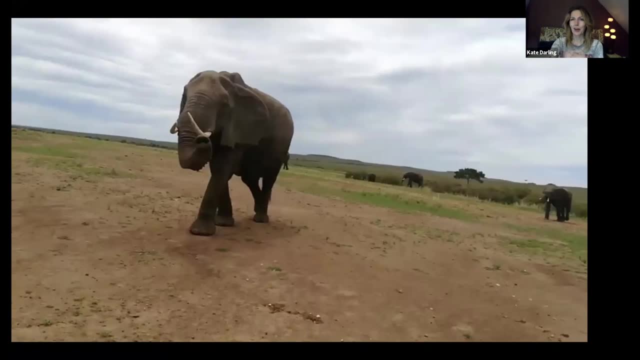 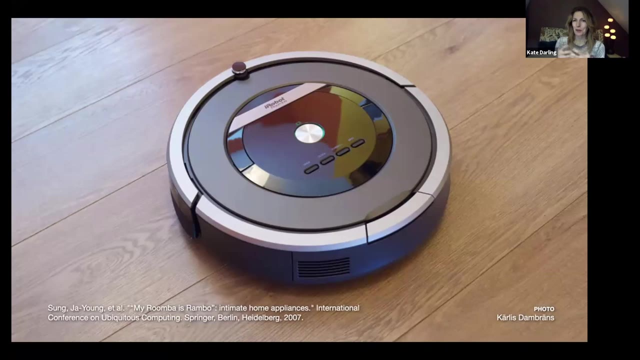 developed hardwiring really makes people project intent onto any autonomous movement in their physical space, and the thing about robots is that they are objects that move like agents, and so people tend to perceive even very simple robots as agents. this is the Roomba vacuum cleaner, not the most sophisticated robot in the world. 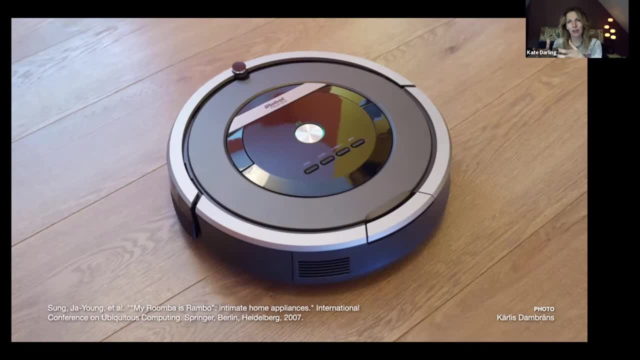 it roams around the floor in vacuums, but the fact that it is moving around on its own through the room with purpose causes people to name their Roombas. over 80% of Roombas have names. don't know the numbers for other vacuum cleaners. 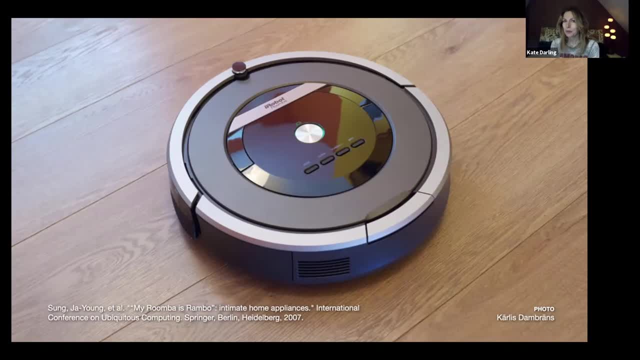 I guarantee you they're lower. people will feel bad for the Roomba when they get stuck in the curtains. people will send their Roombas in for repair. the company has all these stories of people sending their Roombas in and they turn down the offer. 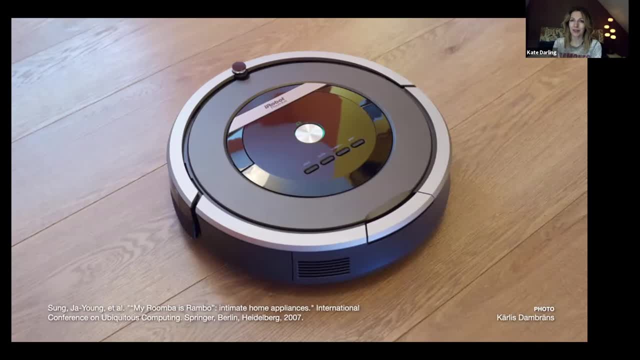 of a brand new replacement Roomba saying no, we want you to fix Meryl's sweep and send her back to us, and the Roomba is just a disc. we also have a lot of more biologically inspired robots that really tap into this instinct even further. 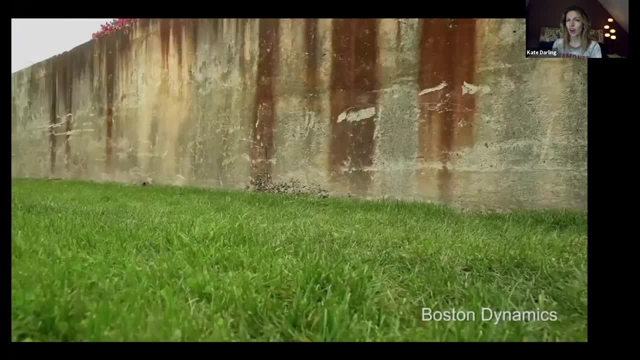 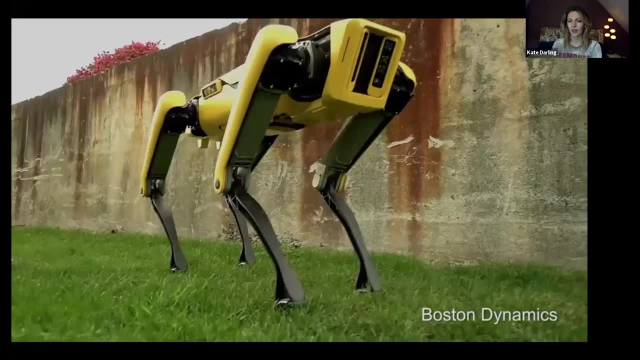 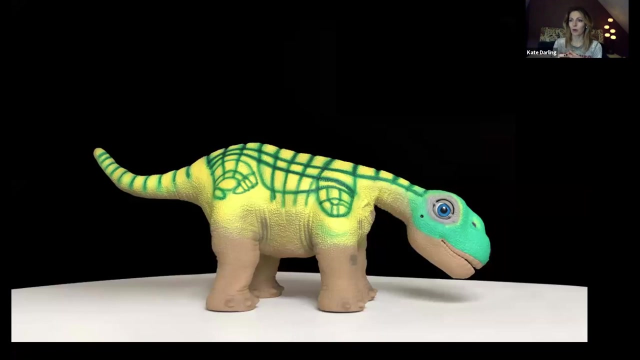 we have another Boston Dynamics robot. it's really hard to watch these things move and not feel like they have some sort of agency. they're very animal-like and this is also something that can be designed intentionally. so social robotics is all about designing robots that are characters. 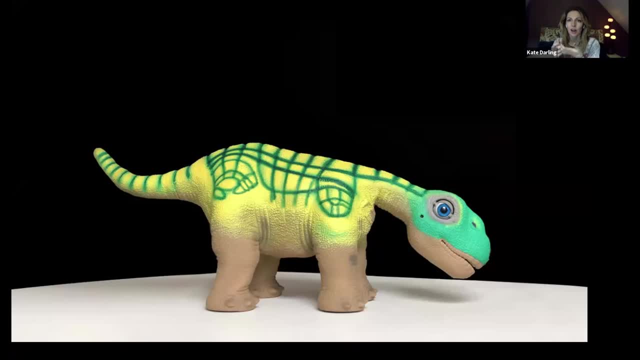 and that mimic movements and sounds and cues that we automatically subconsciously associate with states of mind. I first got really interested in this when I bought one of these. this is a toy called a Plio that came out in 2007 and it's a robot. 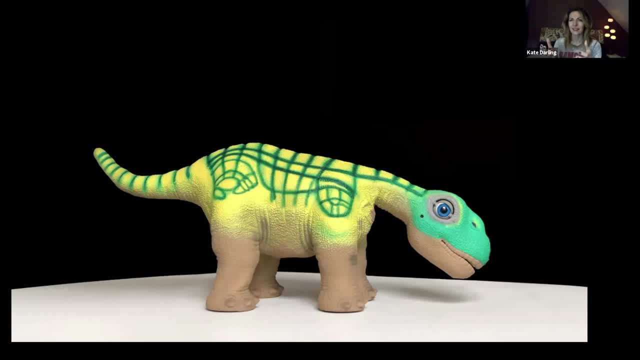 it has all these motors and touch sensors and an infrared camera and it has this tilt sensor so it knows what direction it's facing. and I would show it off to my friends and say, oh, hold it up by the tail, see what it does, because this is what the Plio does. 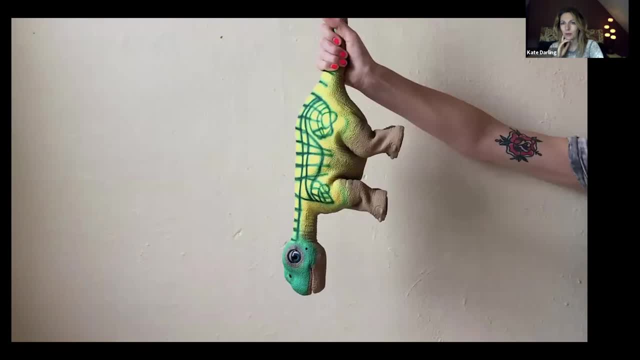 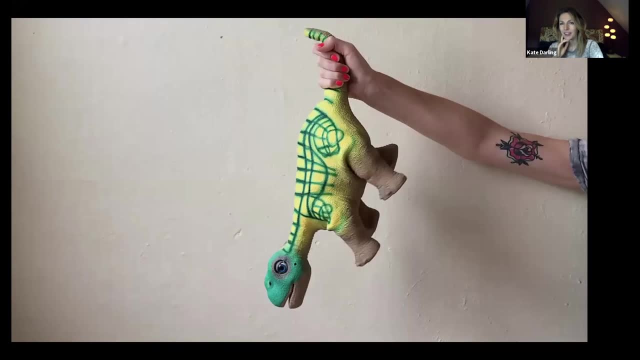 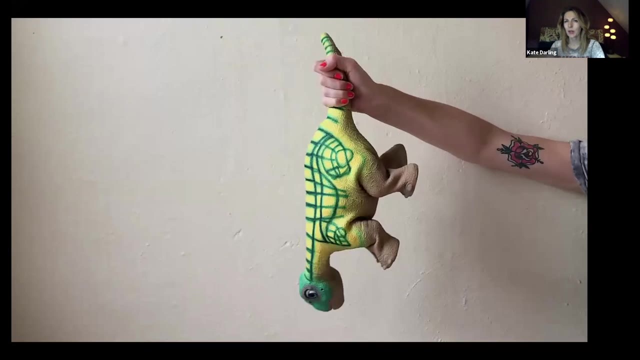 when you hold it up by the tail. I don't think you'll be able to hear this, but you'll be able to see. so it's. but it is crying and what I noticed when I told my friends to do this: some of them would hold it up for a really long time. 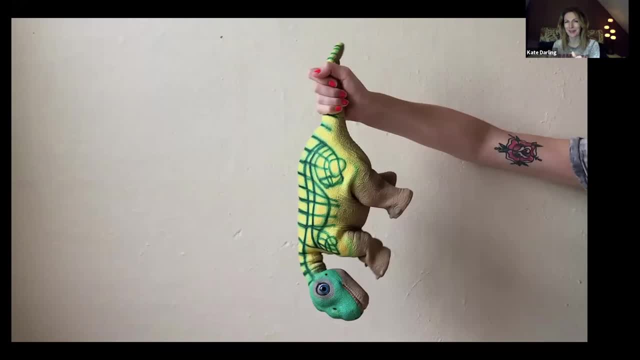 and it started to bother me and I would tell them to put it back down and say, okay, that's enough now. and then I would pet the robot to make it stop crying. so that was really interesting. it kind of sparked a curiosity in me and fast forward a few years. 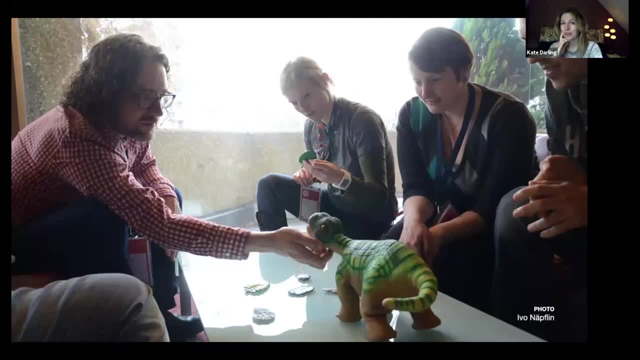 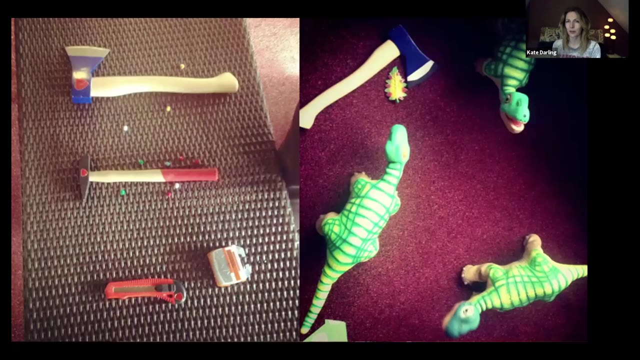 this was years ago now, I did this workshop with my friend where we gave five groups of people. we gave each group one of these baby dinosaur robots. we had them, name them and play with them and interact with them and after about 45 minutes we unveiled a hammer and a hatchet. 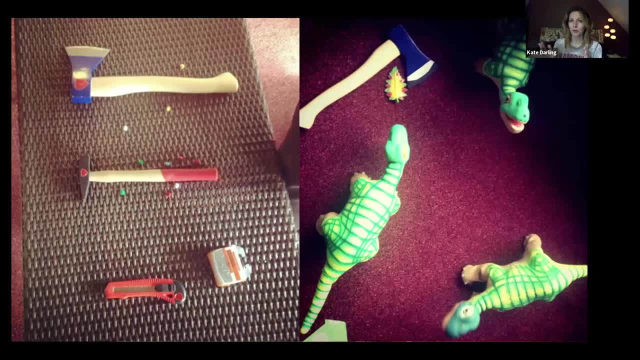 and we told them to torture and kill the robots. and it turned out to be super dramatic, much more dramatic than we expected it to be. people really refused to do it. we had to kind of threaten them that we were going to destroy all the robots unless someone took a hatchet to one of them. 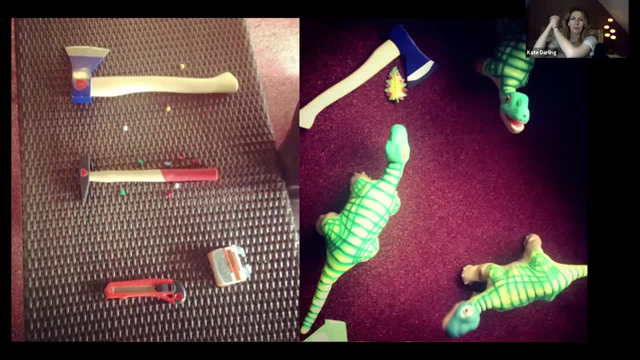 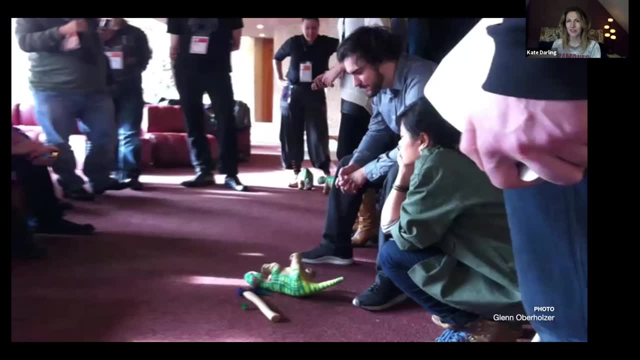 or maybe someone volunteered and we kind of stood in a circle as he brought the hatchet down on the baby dinosaur. and then there was this half joking, half serious moment of silence in the room for the fallen robot. so that was a really, really interesting day. this wasn't science. 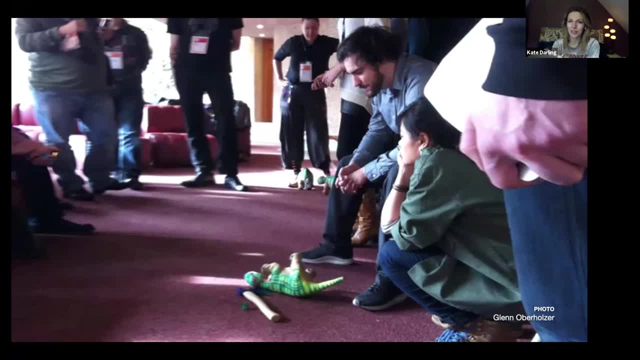 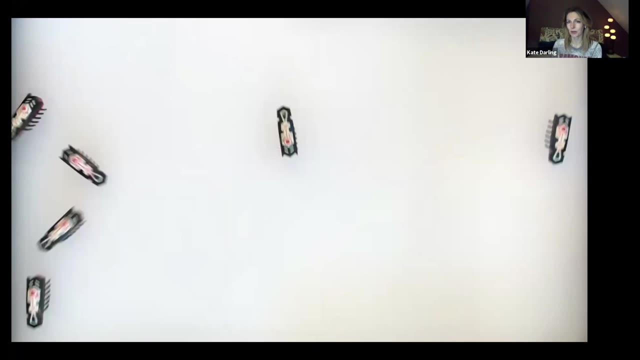 this was not a controlled experiment by any means, but it inspired some later research that I did at MIT with Kalashnandi and Cynthia Brazil, using much more simple robots, using hex bugs, and we had people come in to the lab and smash them with mallets. 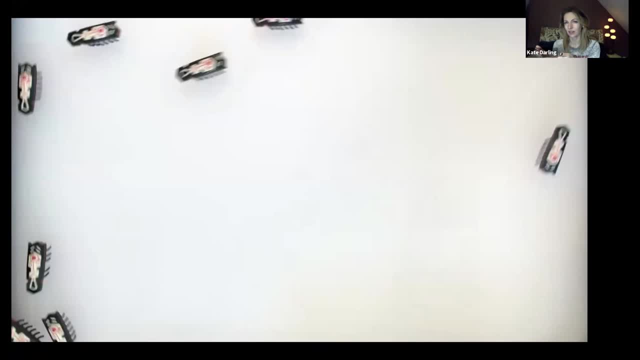 and we were looking at correlations between their tendencies for empathy and their hesitation to hit the hex bug, and it turns out that, according to our results, if you're one of the people who likes to go to Westworld and shoot all the lifelike robots, you might score low on a test for empathic concern. 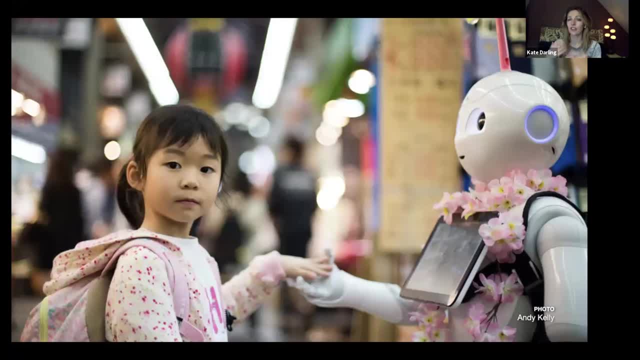 generally. so that was just a little study, but there's a ton of research in human robot interaction that shows that we respond to the cues that these lifelike machines give them, and we respond even if we know perfectly well that they're not real. now, at the end of this conference, 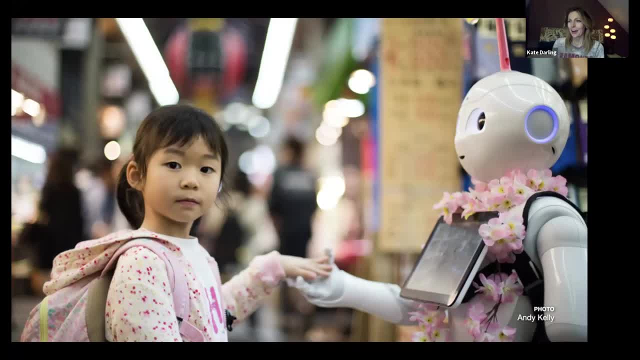 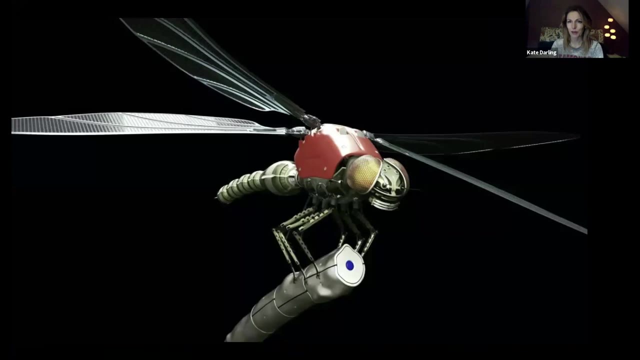 where I met my lemonade friend Scott. we bumped into each other again and he was like you know. I'm thinking that maybe you were right, because he had seen this demo at the conference of a dragonfly robot. it wasn't this one. this is some random rendering of one. 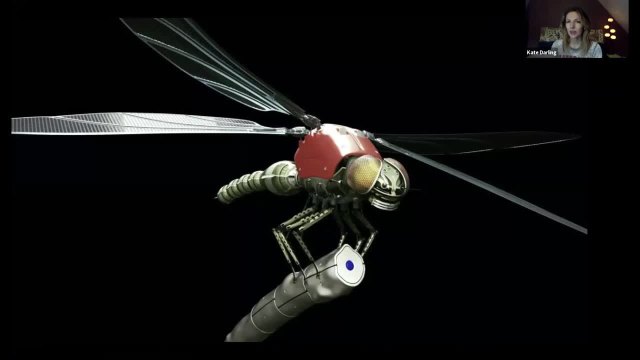 it was flying around a room and he said he had noticed the people watching it were just so transfixed, watching this thing buzz around over their heads and he was like I don't know, but maybe we are built this way, but I still don't buy it. 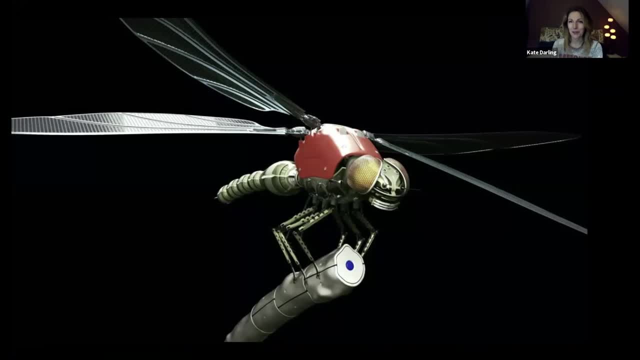 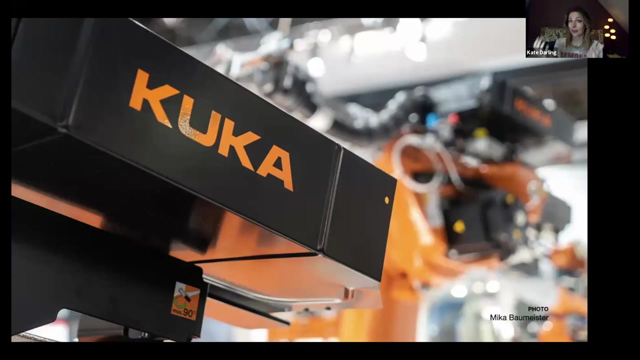 so we shook hands and we decided to come back to it in a few decades to see who was right. but the next few decades are going to be pretty interesting to watch is that robots are moving from factories, as Sami mentioned, they're behind cages, behind walls. 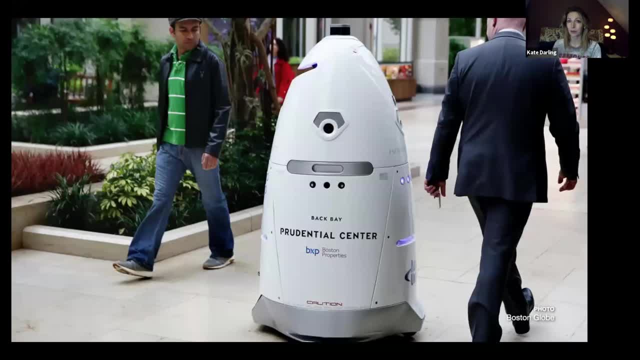 but now they're moving into more shared spaces as the technology improves, into workplaces, households, public areas. so we have these machines that can sense and think, make autonomous decisions and learn, coming into spaces where they're interacting with people and they're not alive, but people sometimes treat them. 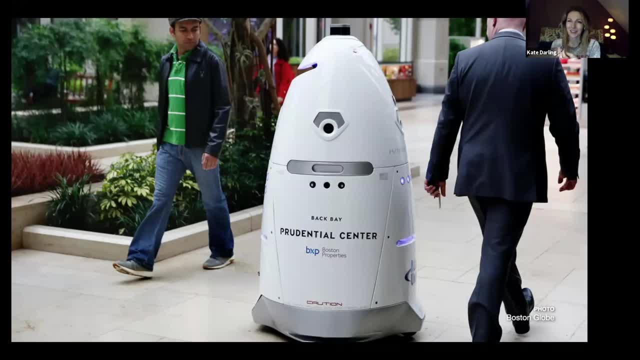 sort of like they're alive, and that's really important to understand, because if we're trying to integrate the technology, we need to understand when and how people treat it differently than another device, and one of the reasons this is actually a cool thing is because it can be harnessed. 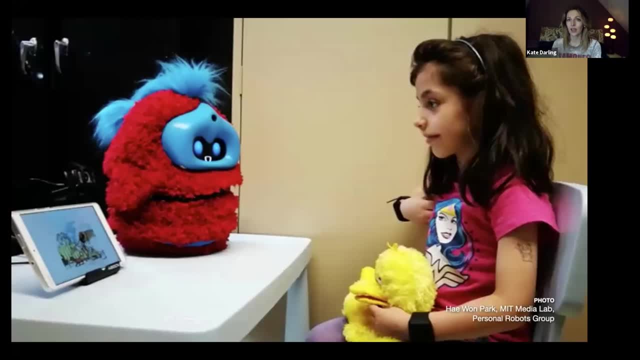 there's already some really cool use cases in health and education for using social robots that rely on this emotional connection. for example, there's some really promising research on using robots in engaging children on the autism spectrum in ways that we haven't been able to do previously. 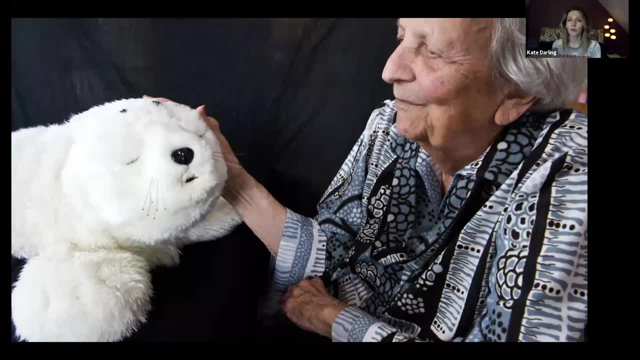 or there's the PARO, which is the therapeutic seal that's used in nursing homes with dementia patients. that's really cute. it really kind of gives you the sense of nurturing something, and often when I tell people about PARO they say: oh my gosh, Kate, that's so terrible. 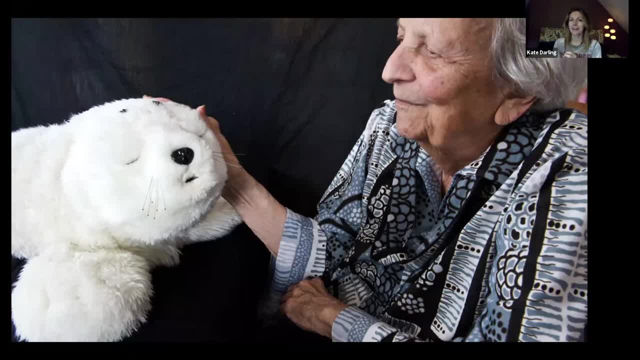 I can't believe we're giving people robots instead of human care, and I think PARO is a terrible replacement for human care. don't get me wrong: the common problem that we have in our conversations around robotics- not just social robotics, but generally- is that we're often comparing robots to humans. 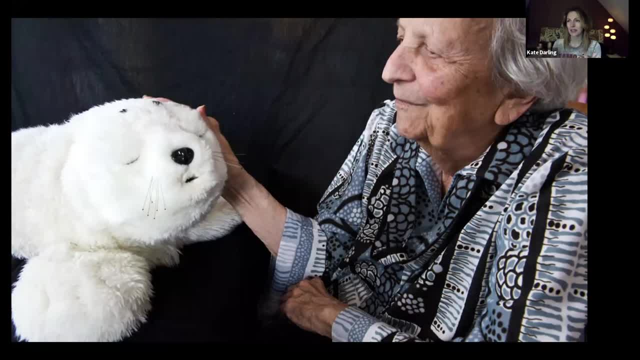 and talking about them as a human replacement, but this analogy doesn't really make sense to me, because artificial intelligence is so different in skills from human intelligence. I think other analogies would make so much more sense, and so, for example, the PARO actually isn't a replacement for human care. 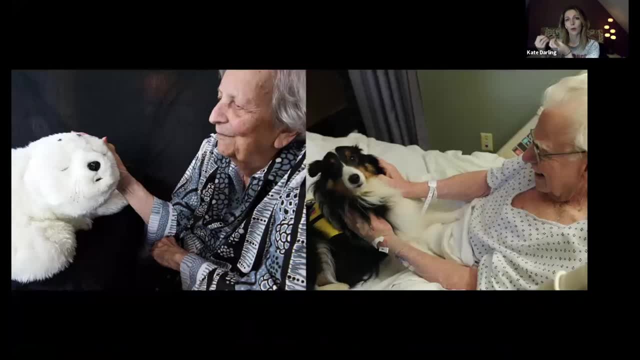 it is a replacement for animal therapy in contexts where we can't use real animals for a lot of reasons. but we can use the robots. they have a very similar effect. they lower people's blood pressure. they cause oxytocin release. they've been able to use it as an effective alternative to medication. 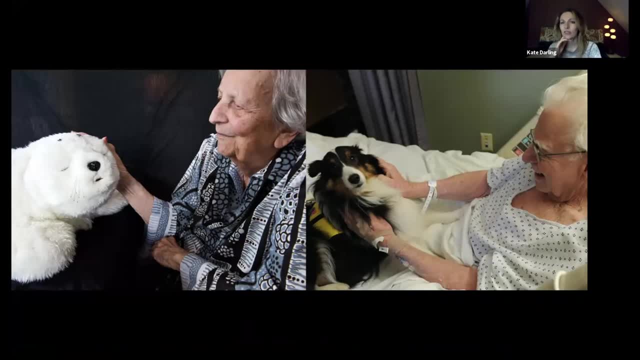 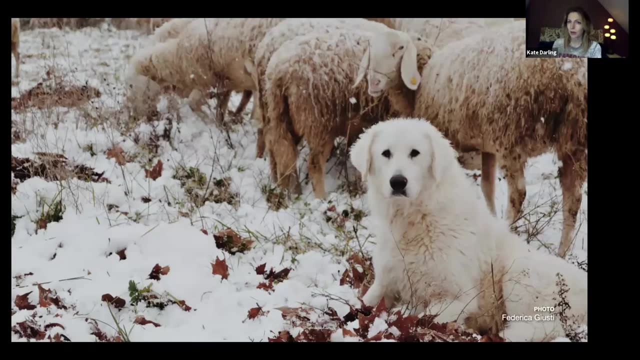 to calm distressed patients. so some pretty cool uses for that and, in general, this animal analogy. we've used animals for work, weaponry, companionship throughout history and we've used them not because they do what we do, but because they do what we do and the true potential. 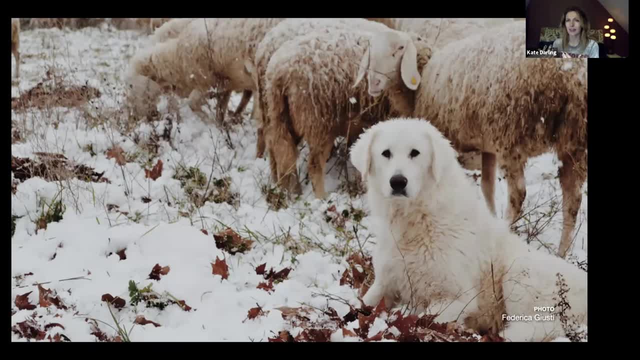 of artificial intelligence and robotics, in my mind, is not to recreate what we already have, unless we're trying to save lives or, as Sami said, the dirty, dull, dangerous work. but in general, the true potential here is to partner with this technology in what we're trying to achieve. 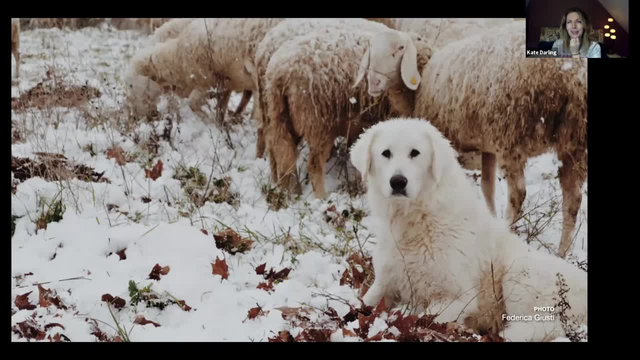 so I totally agree with Sami on that one, and I think this animal analogy applies even further than just the integration of robots in the workplace. I think it also applies socially because, if you think about it, throughout history we've treated most animals like tools and products. 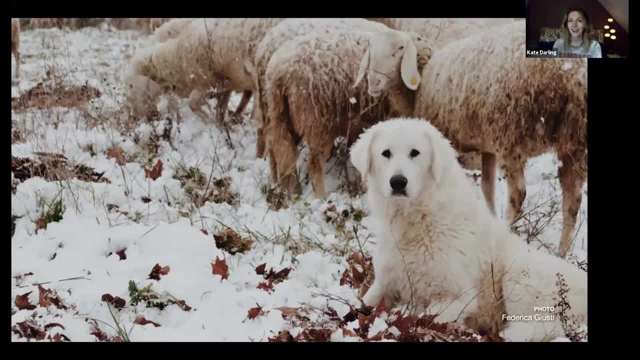 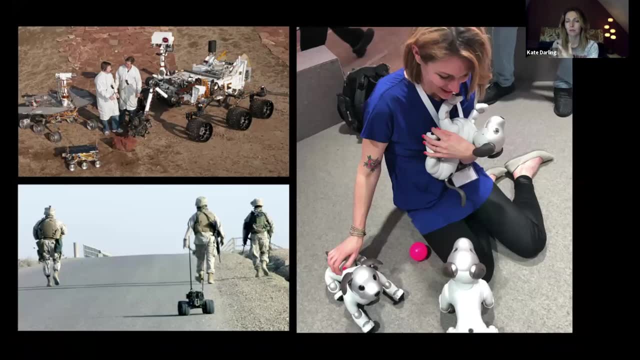 and then some special animals we've given a status as our companions, and I think it's entirely plausible that we might start seeing the same thing with robots, where we treat most of them like tools and products and then some as our companions and have more of a social relationship. 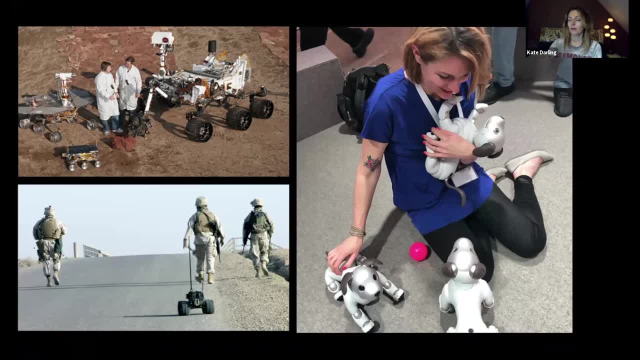 with them. now we know what Scott would say to this. I have this to say to Scott: Scott, maybe you're right. maybe once generation A is out there and robots are ubiquitous, maybe they are going to treat robots just like any other device. but I just don't buy it. 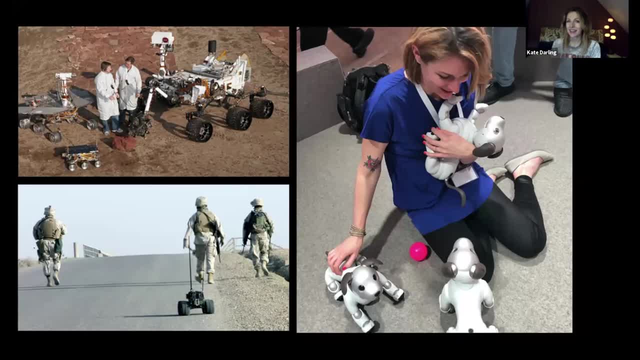 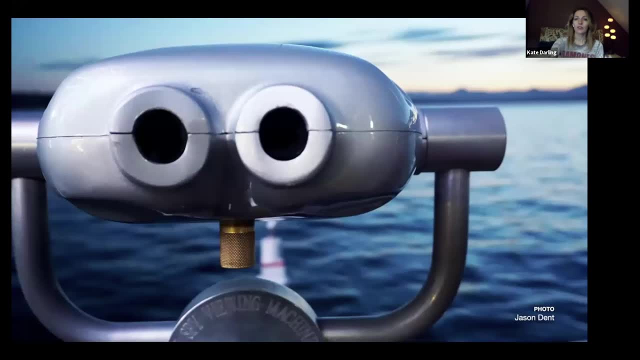 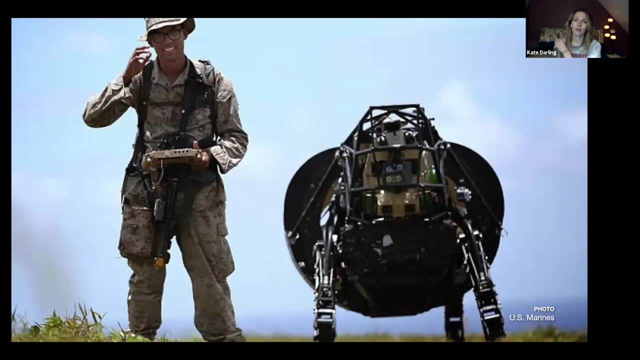 and if I'm right, then there are some questions that need to be answered sooner rather than later as we start integrating this technology. is it okay for soldiers to become emotionally attached to the robots that they work with, or is that dangerous? can robots actually be used as an emotional support? 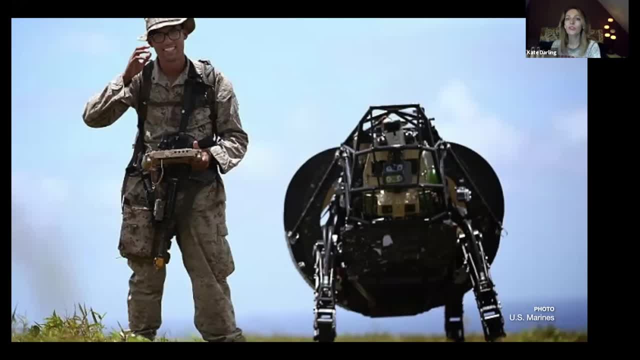 in war or crisis situations. just like horses were used in World War I, they initially started out as tools. they ended up being emotional support for a lot of the soldiers. that may sound ridiculous, but it sounded ridiculous for animals back in the day as well. other questions like: is it okay for people to behave violently? 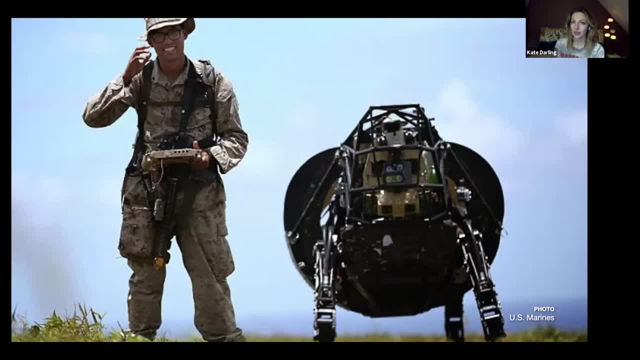 towards very lifelike robotic objects, or could that be desensitizing to violence in other contexts? are companies or governments going to leverage this very persuasive social robot technology to manipulate people and coerce them, and how can we try, through regulation or other methods, to curb some of the dangers? 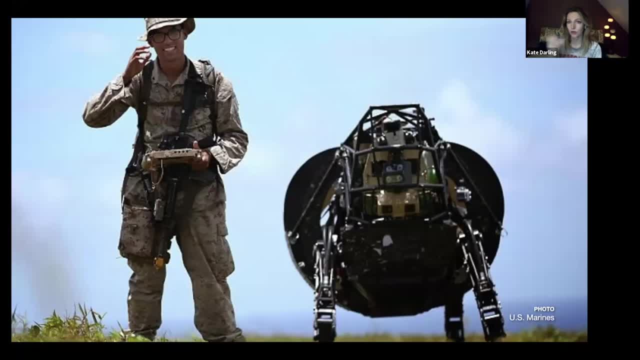 of people abusing us through this technology in a world of unbridled capitalism, and also how can we lean into some of the cognitive effects of this in health and education and really try to build social technology that benefits people. so I think that the insights that we glean from human robot interaction 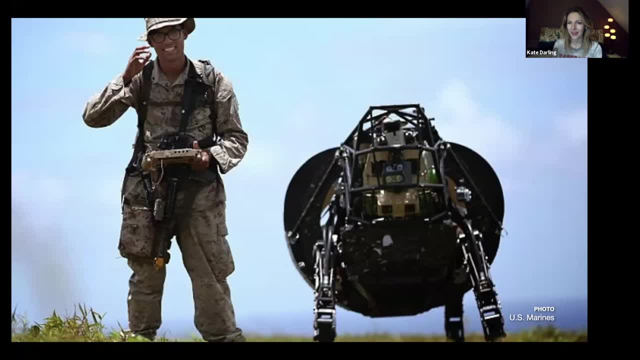 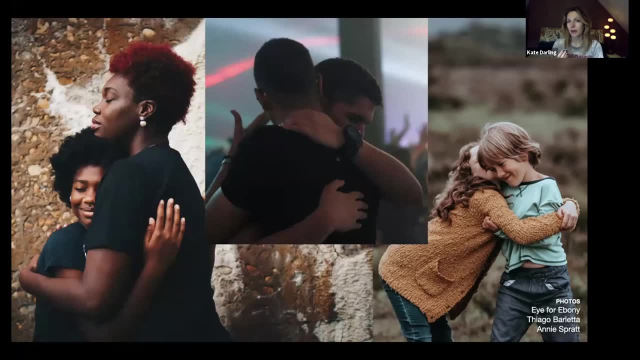 are really interesting, but also really important, and one of the things I love most about it is that we're learning not just about how to integrate the technology better. we're also learning more about people. we're learning more about empathy and communication and, in general, how we relate to each other. 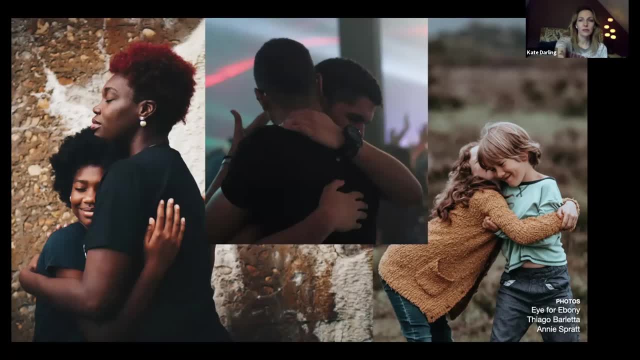 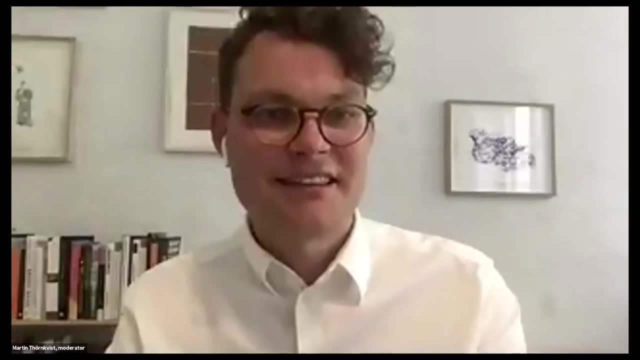 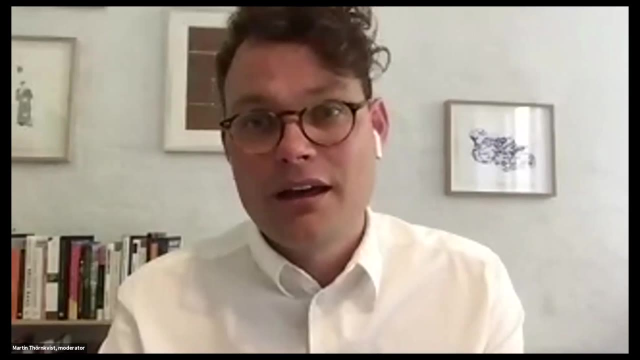 so I will stop there and I look forward to questions, and I look forward to questions and I look forward to questions. Fantastic, Thank you, thank you. thank you, Kate, and also Sami, for two great talks. we have a little bit more than 15 minutes for questions. 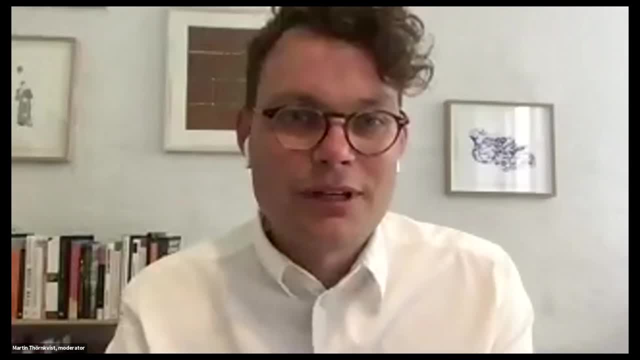 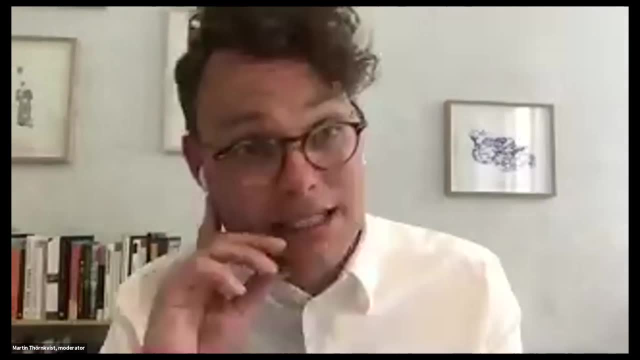 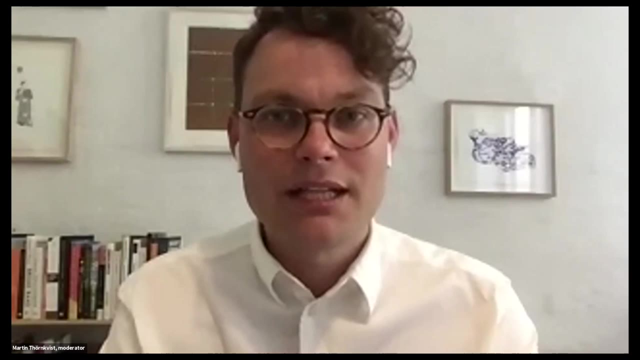 and my colleague, Jeanette will call out those who can ask their questions. I will actually ask the first one, and it's a question for both of you, Sami and Kate. so in a couple of weeks we have a lesson on AI and the future of work. 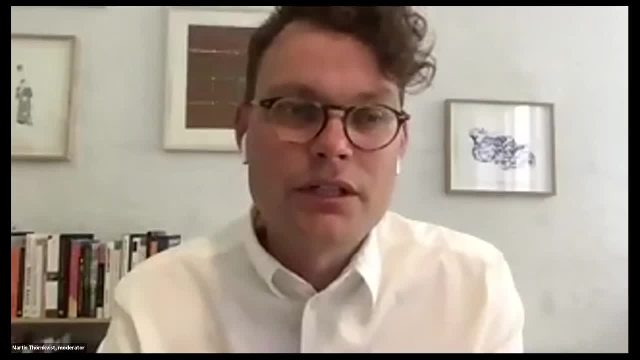 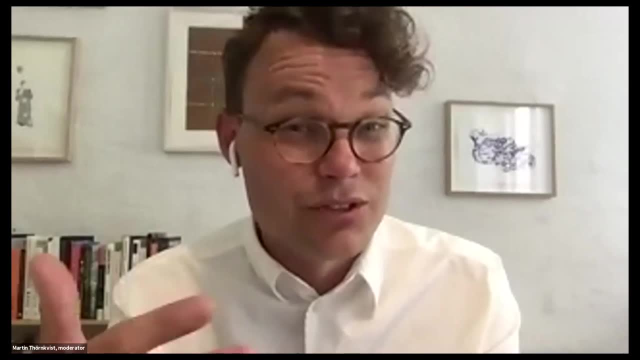 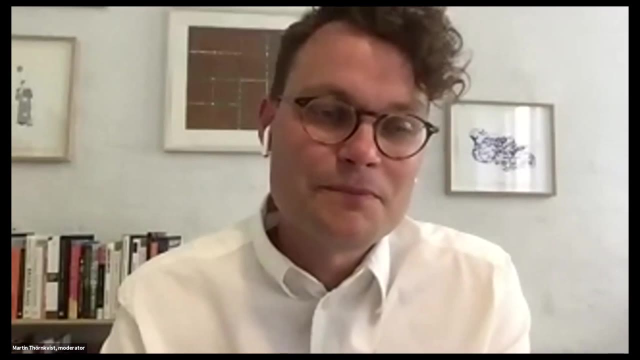 and work is something that you both mentioned in your talks, and I'm wondering, if I'm starting out my work career today, what strategies should I employ to surf this wave of robotics and automation, instead of spending my time worrying about losing my jobs to it? do you want to? 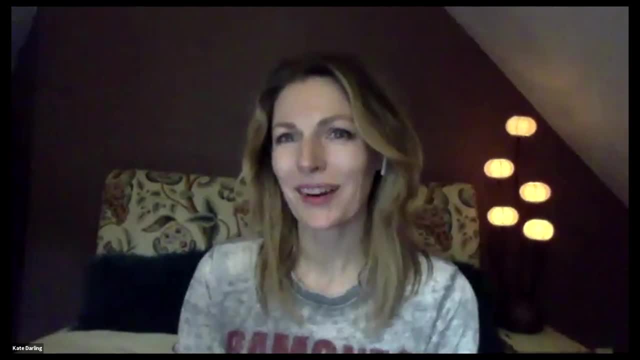 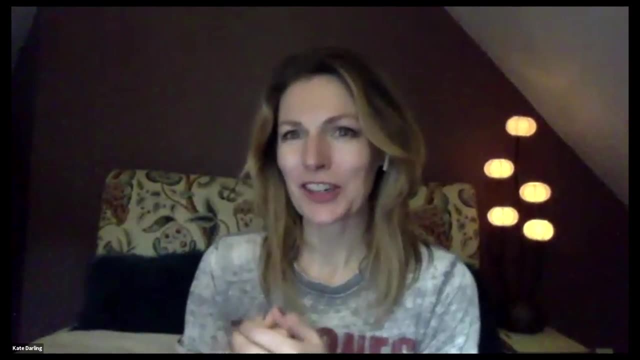 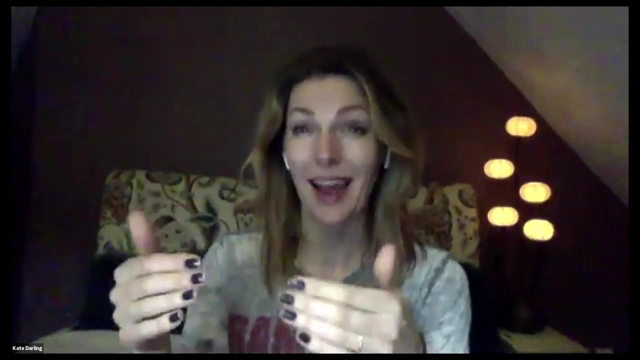 I could start. so I think that, despite the fact that the main potential of robotics is to assist us, I think there are certain things that can be automated that might be done by humans today, anything that's a very, very well defined task within well defined boundaries is something that can be automated. 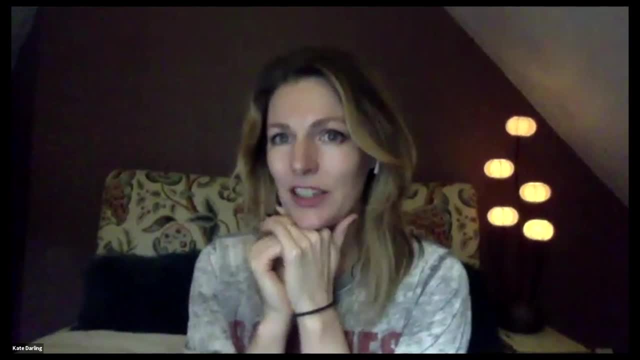 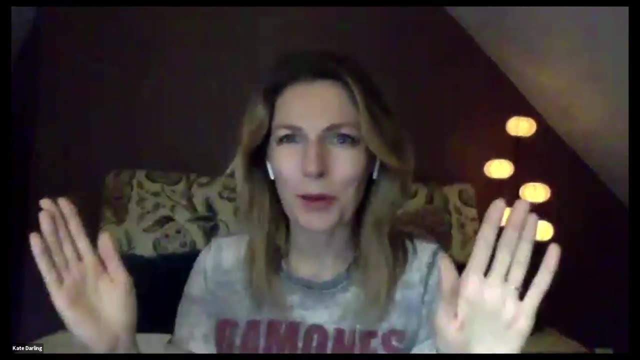 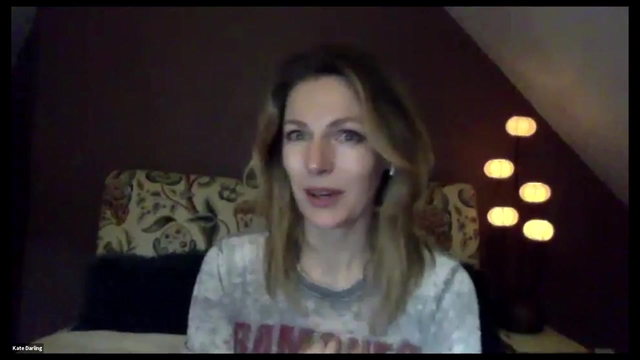 and so it's kind of industry specific- how this is going to affect different industries, but kind of like a very general. what should you be watching out for as you enter the workforce is maybe moving towards the skills that machines aren't good at doing. anything that requires. 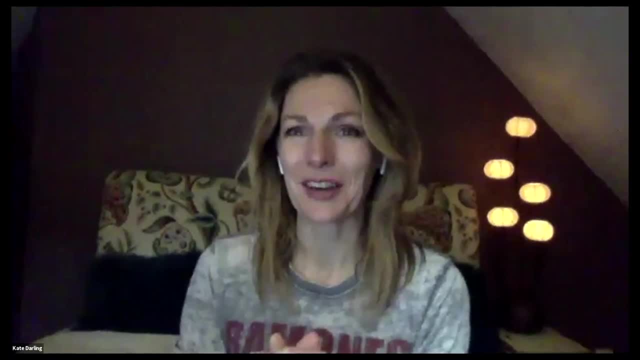 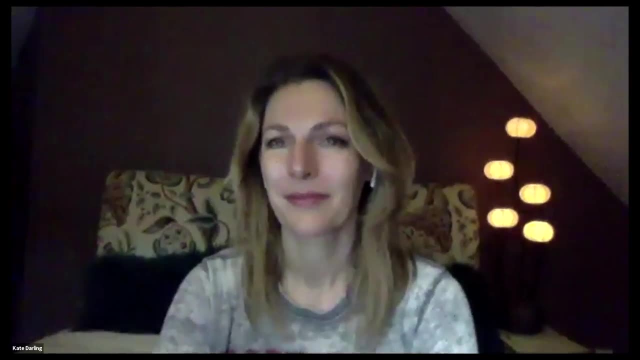 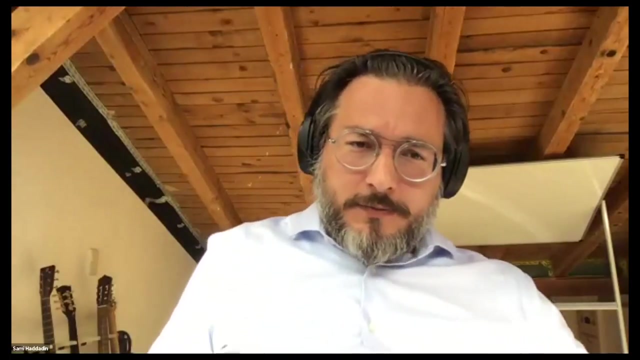 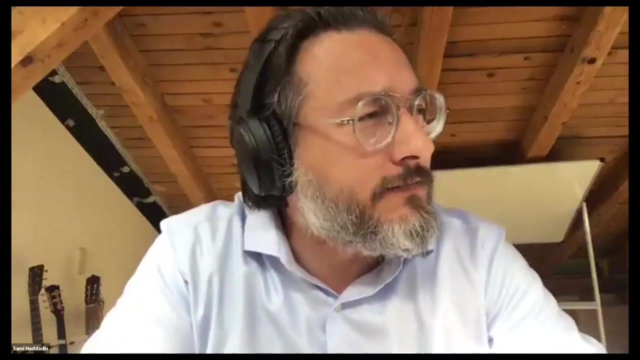 context or concepts or any human to human communication. I think that that's still a pretty good bet. if I would answer this question, I guess my answer is a little bit along the lines of: sure, that's a, it's probably a good bet and it makes a lot of sense. 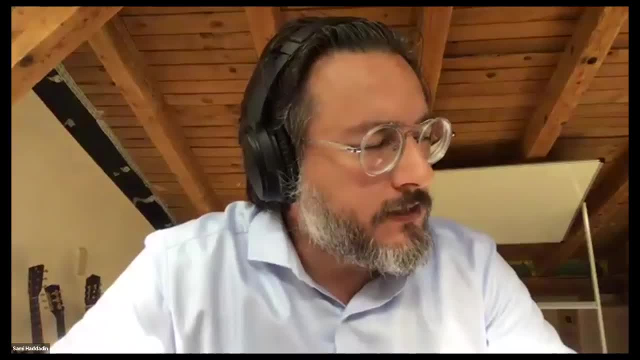 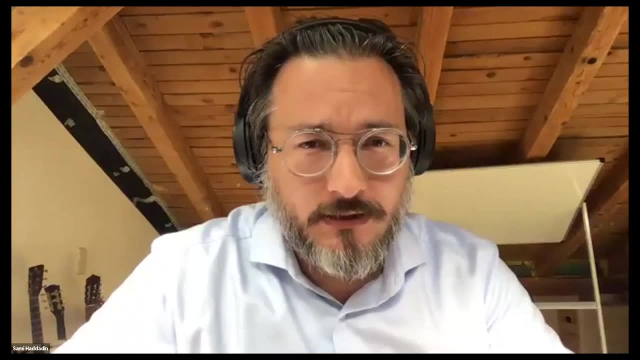 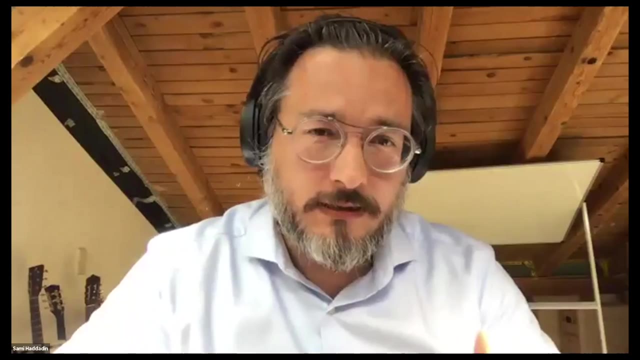 I just think that it's important to really see that this is a kind of new type of technology in a way, so it's not just we are kind of entering a new phase of machines that really show a certain type of complexity that is beyond the typical. 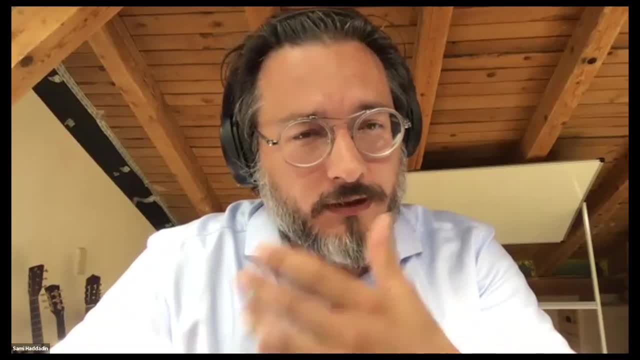 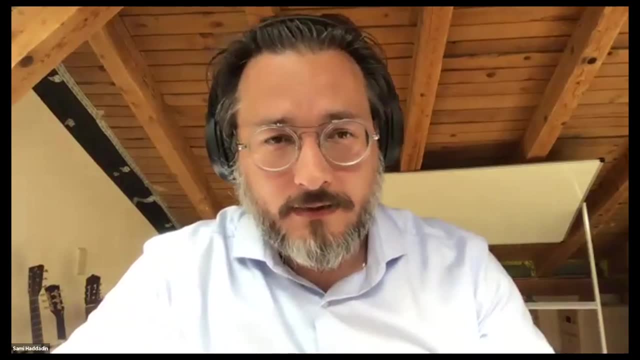 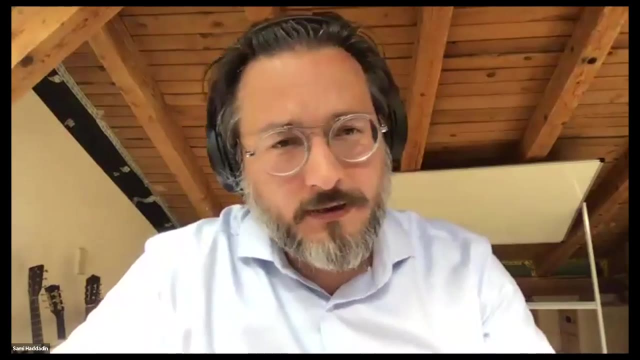 techie oriented things. so it's not only anymore for technologists and people who like to play around with technology, but it actually affects people's lives on a broad scale, beyond the usual level, I would say. so I think what is an extremely important- at least take home message. 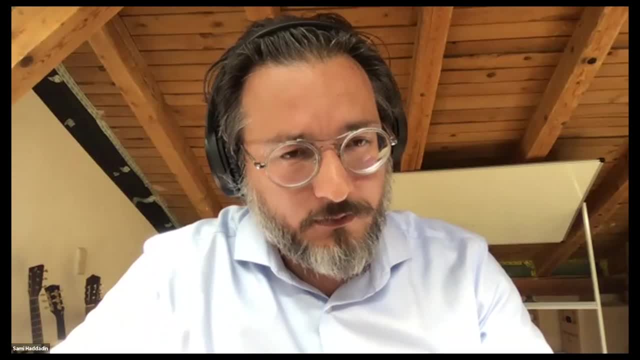 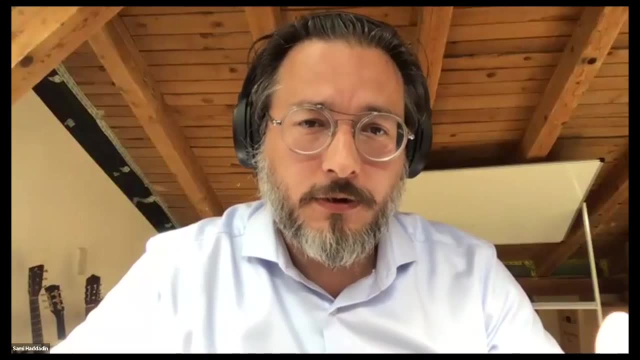 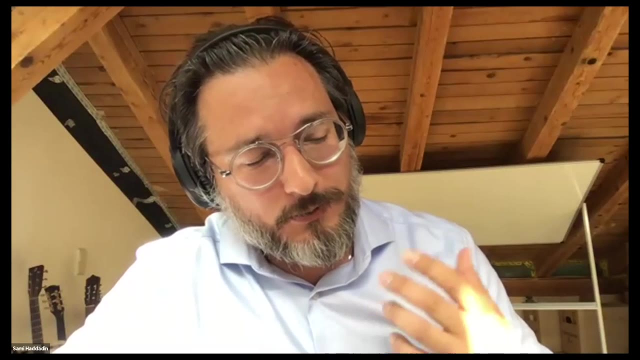 that I was able to gather from many of the projects I've been doing is that we as technologists need to really think purpose led. I mean we should be purpose led. we should really think much clearer in the long term shot and if people want to change the way that the world works. 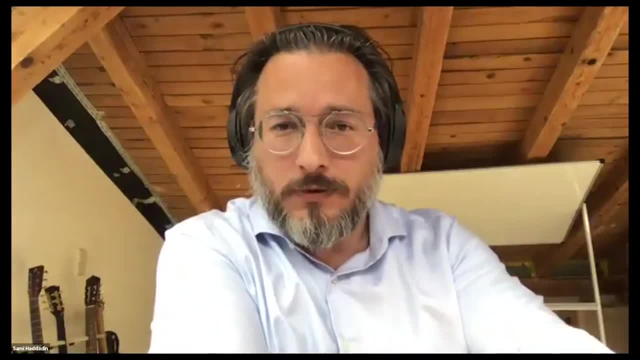 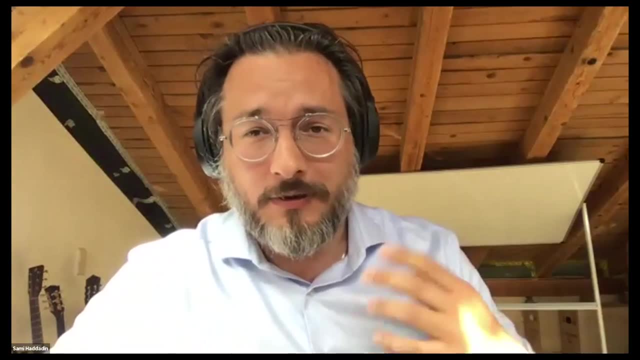 I mean, look at the wonderful tool that we have the pleasure to kind of come together with, zoom next to all the other tools. I mean this has been developed by technologists that probably did not think that this would be one of the key contributions to bring people together in a phase. 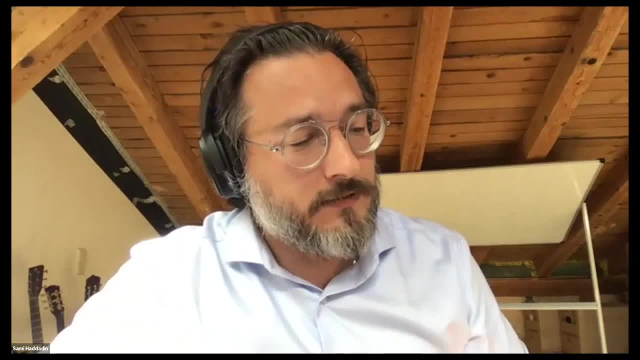 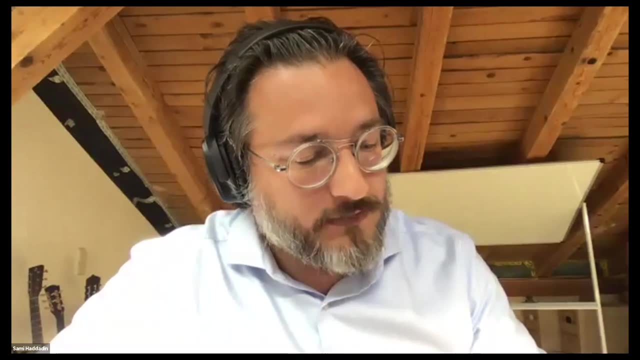 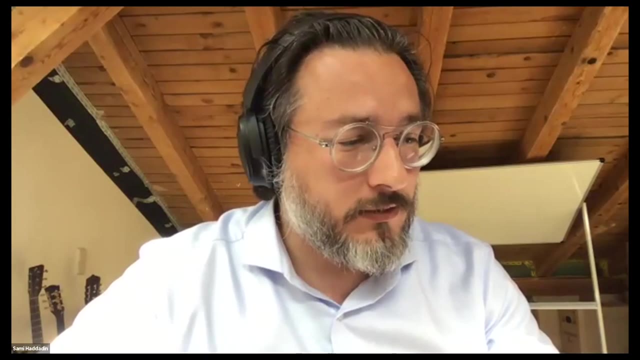 of I mean otherwise collaboration. so I think it's really the yeah, I really believe that it's a great path one could take, and it's also coming with a great responsibility, in the sense that it's the things we're doing might really tremendously affect everybody's lives. so 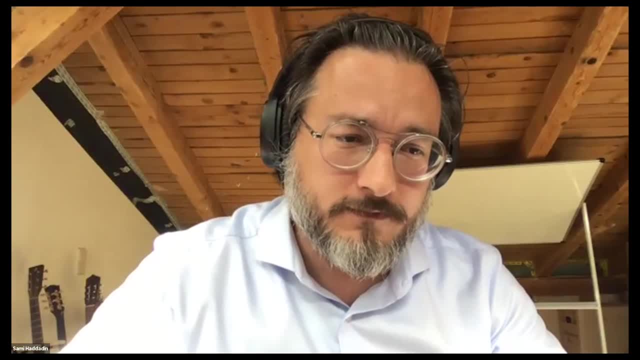 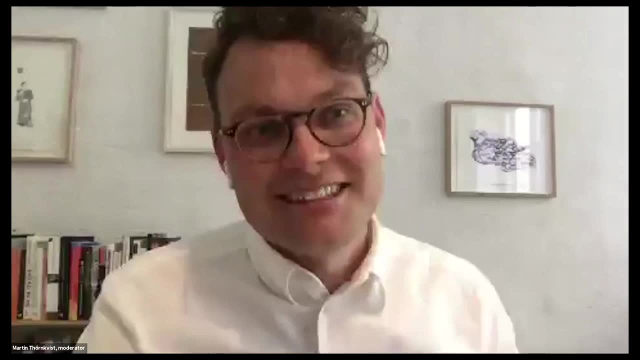 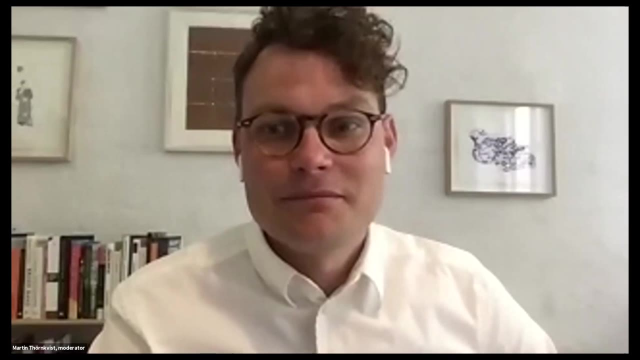 this should be very consciously in the decision, in the choices. okay, so we should all be students of yours and become robotic engineers. that's the safest bet, maybe. but now I'm going to hand over to to Chanette and she will bring out some more questions from the audience. 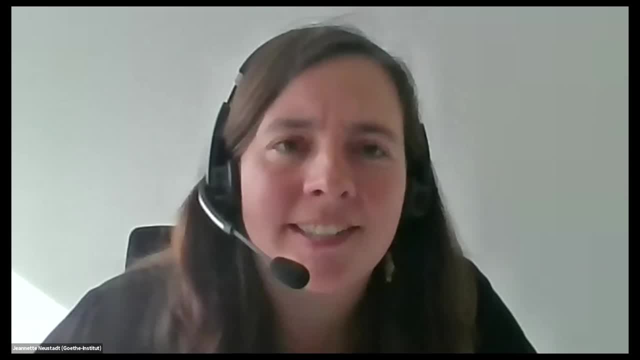 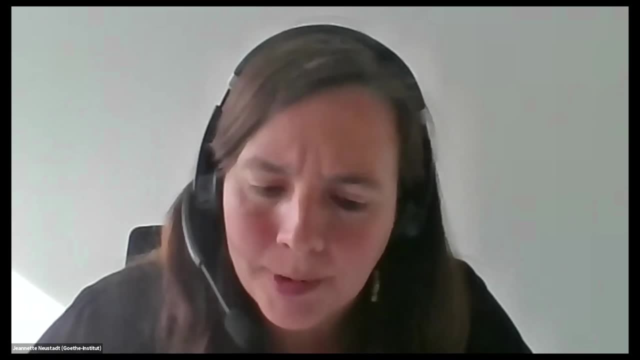 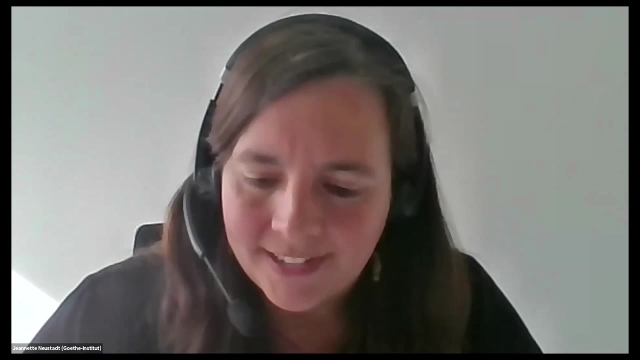 yes, there have been a lot of very philosophical questions. so can robots be aware of their existing? can they build up emotions, can they have emotions, or can robots become aware of themselves? so there are many questioners. maybe we start with Fabio Farvan, or whoever else will. 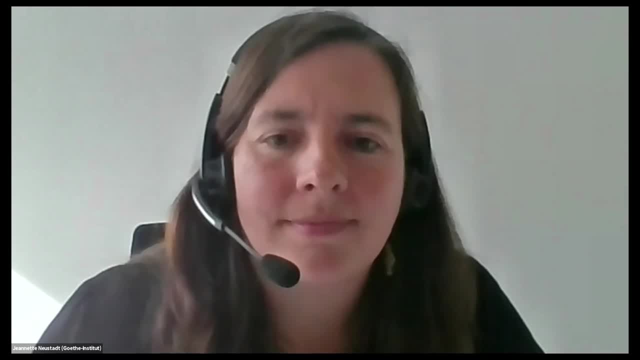 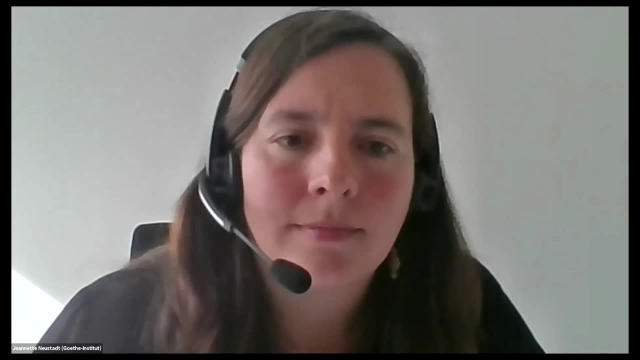 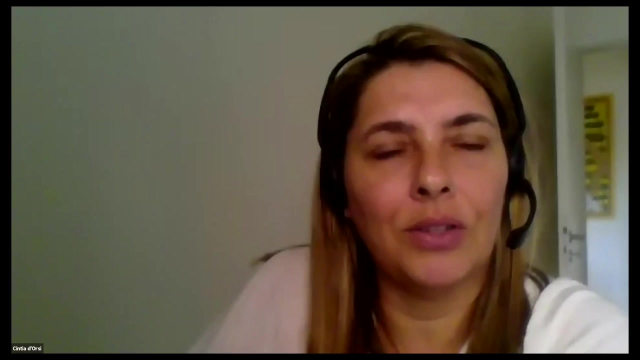 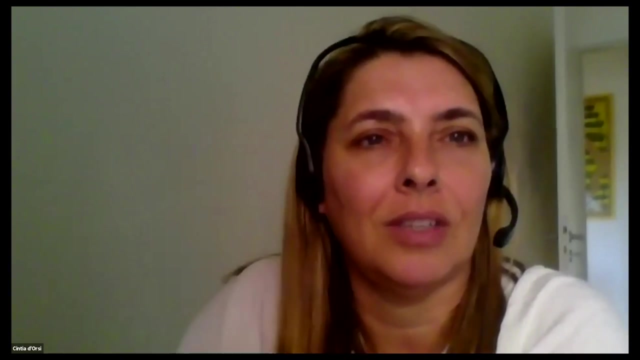 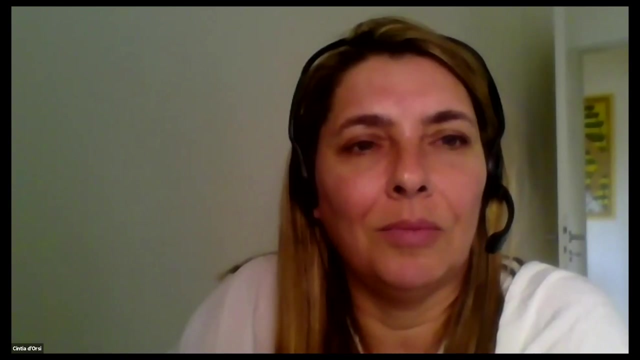 speak. can you unmute yourself? no, doesn't seem to. first question was mine. if robots are aware of existing, I mean it's going to be. I know they are not now, but if they can learn, maybe they can learn that they exist. so they would fight to survive. 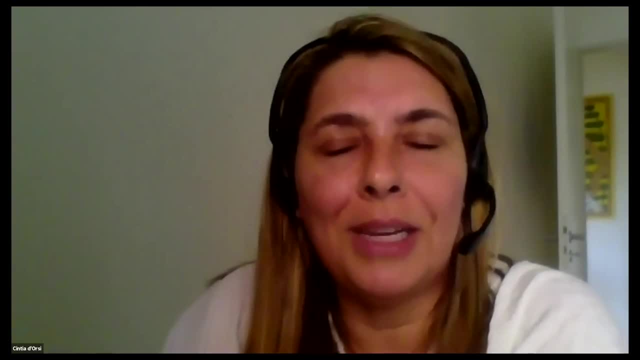 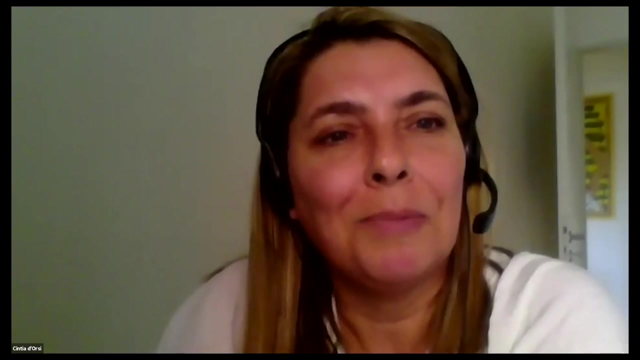 or something like that. I mean, in the future, if you do this same experience that Kate did, the robot dinosaur can run away or fight back. I don't know, it's because I am writing a story about this. oh, that's interesting. well, I would prompt you to also think about: this in terms of animals, who do we believe? I mean, we don't have a good definition of what consciousness is, which is like the main problem. but with animals, we do a lot of experiments with them and we don't seem to care and they don't seem able. 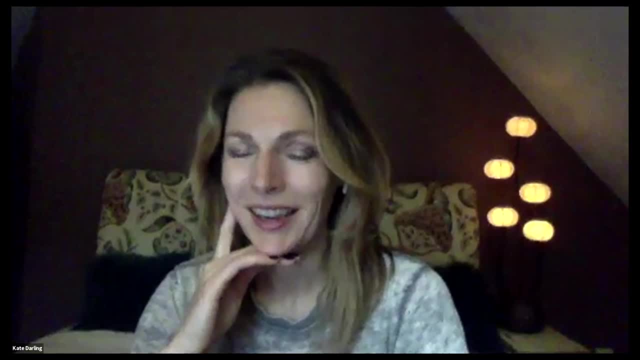 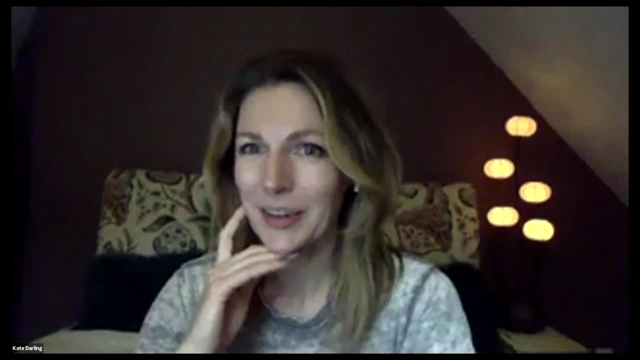 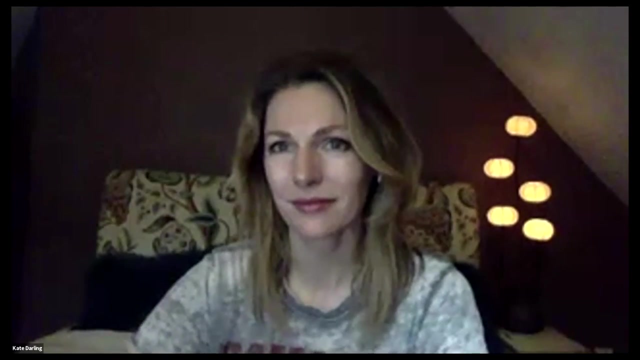 to be able to fight back in that way. so, as you're thinking about this question, think about how we've treated other non-humans who have developed or have consciousness in that sense as well. but I'll let Sami answer the technical question of programming consciousness into machines. 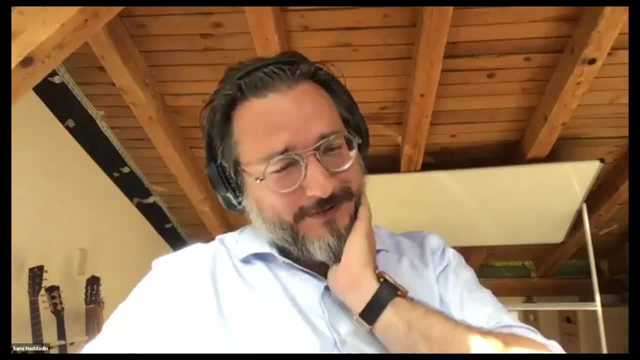 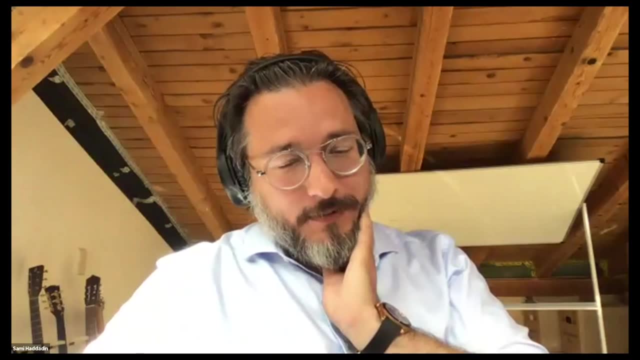 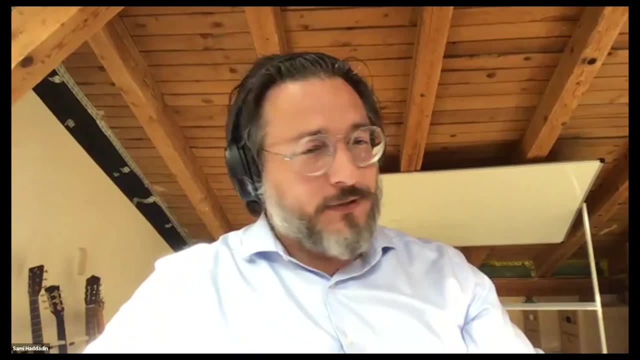 oh great, thank you for the for the pretty hard question. so I must say I pretty much agree with many things that Kate was just saying, and she was saying something very important in the beginning. that was: we don't have a good definition of what you're asking. 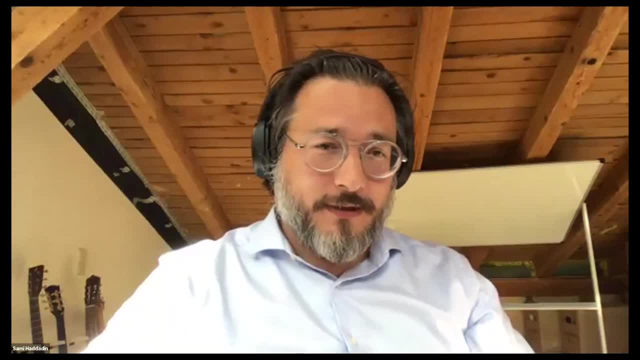 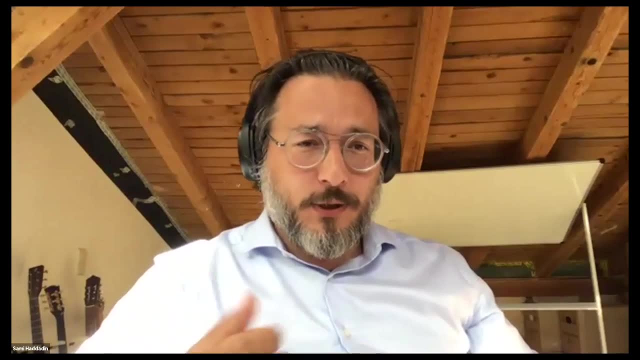 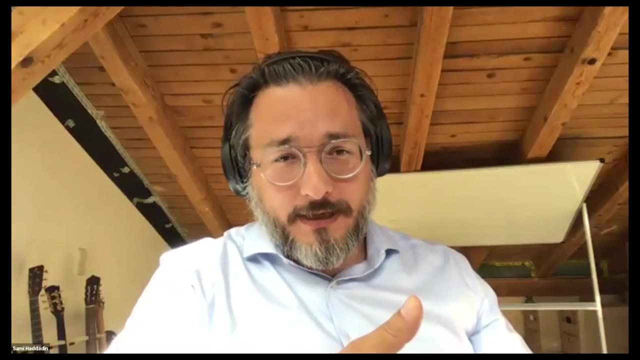 about. so what is conscious? what is the self? a very famous polymath like Leibniz was thinking about the existence and the body and the soul. that's always a problem if you ask these specific questions and you know as a human, I would say my human answer. 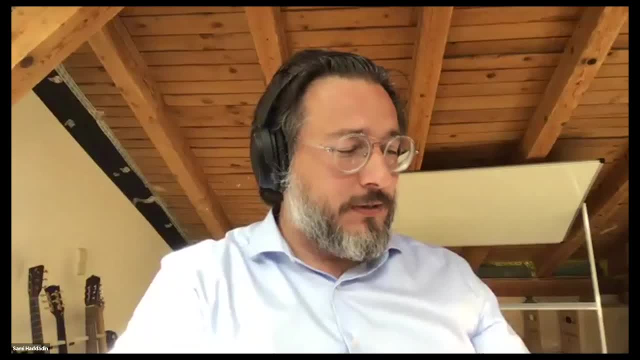 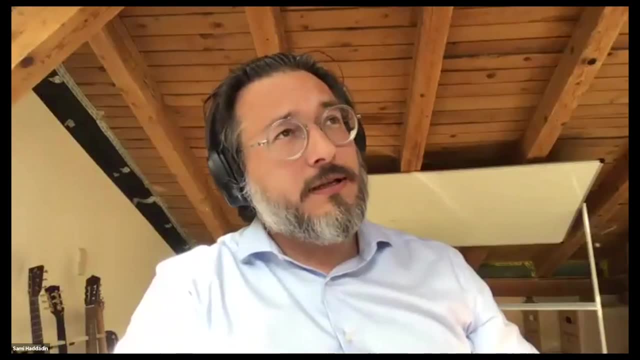 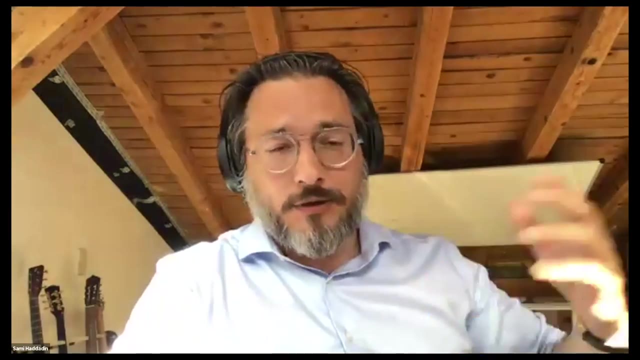 is no way, because I mean at least not as long as I'm building them, because I'm just not able to, probably. but I really think that the idea of building a machine, you can do the thought experiment of entering it, a little bit like in building a machine. 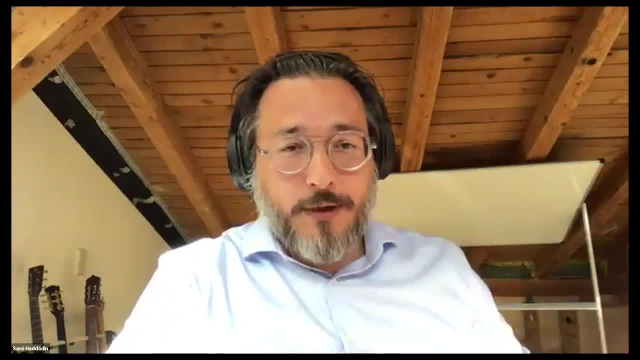 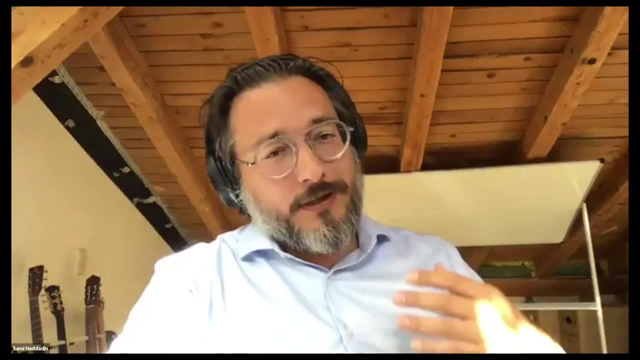 you walk into it, you look at it, it functions. it does something. you disassemble it. there is no consciousness, there's nothing right, and you build it together and voila, it functions again. so if this is the narratio and the narrative and the interpretation that we want to take, 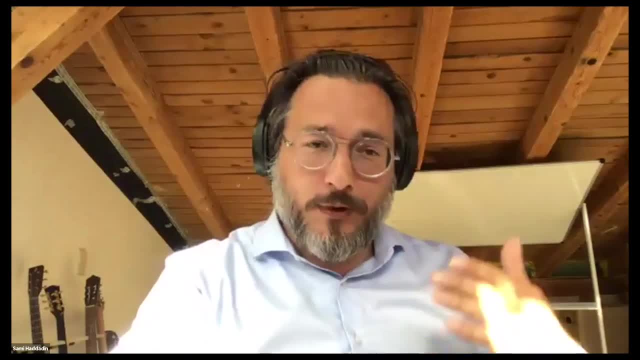 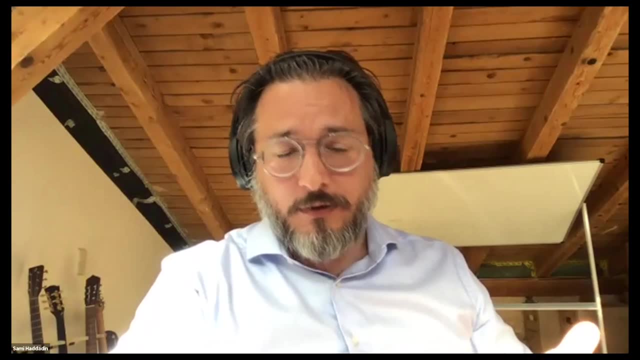 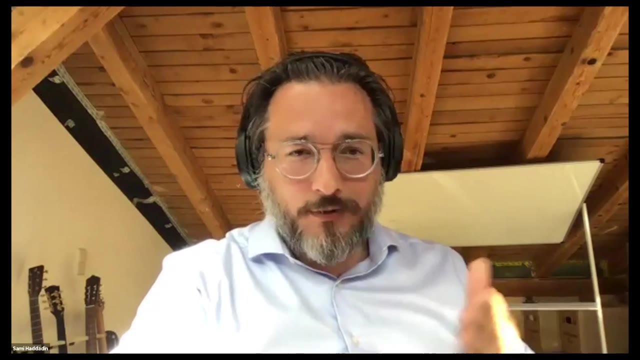 my answer would be certainly no. if you ask me define what we mean by that in technical terms, then you can call it whatever you like. we may call it consciousness, we could also call it- I don't know- fridge, and we would implement what we just defined to be consciousness. 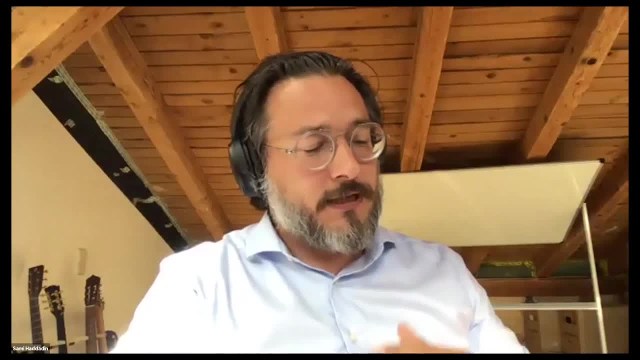 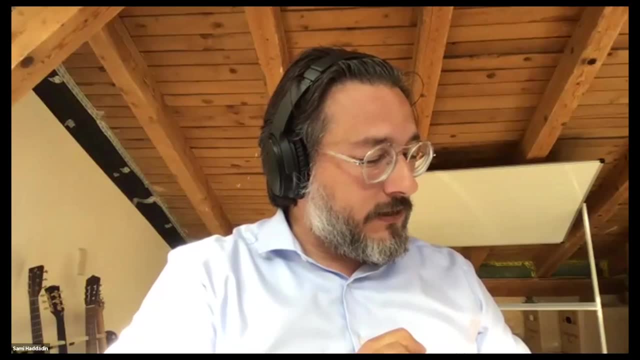 or fridge. so- and I'm giving this a little bit jokey answer because it's really in technology and science- we need to define very precisely what we mean by that, but to maybe also give you the technical answer to that, there is the concept of the self right. so 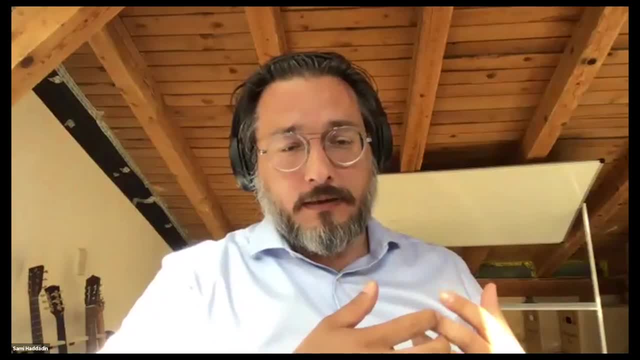 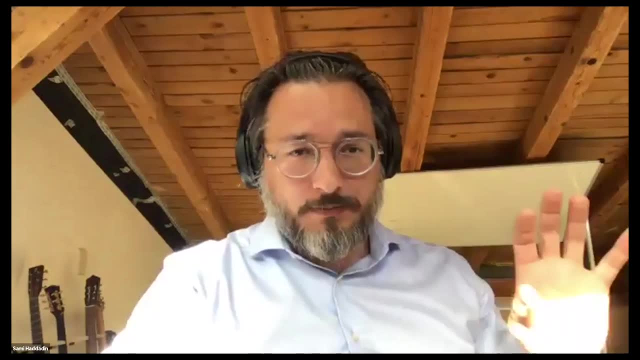 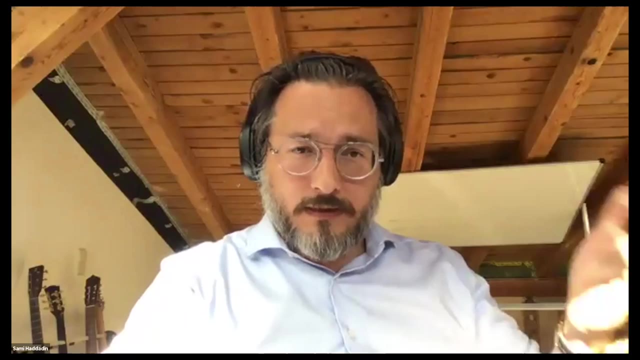 a robot that has a body, an embodiment, needs to understand that it has a body. but understand is the word meaning. we have developed a program that has a part in its storage mechanism. that is the representation of the physics of the body, and then it has to have this understanding of. 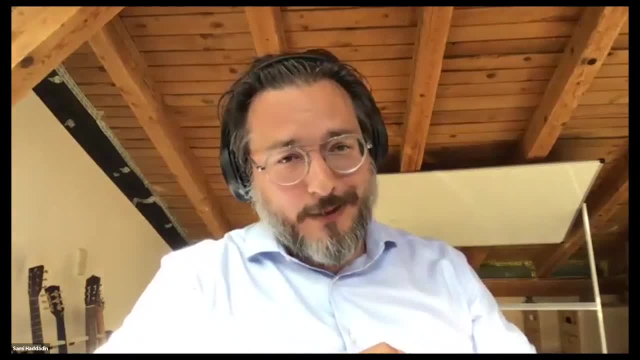 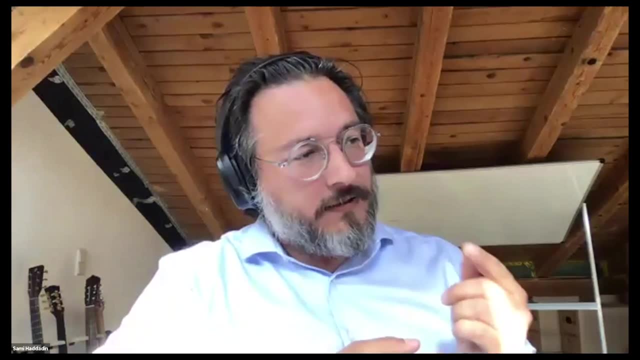 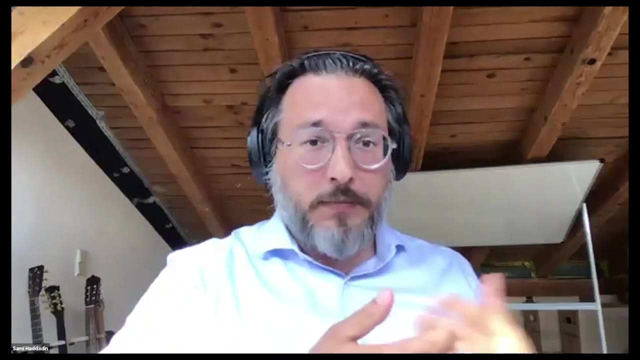 interaction right. action and reaction have to be made algorithmically readable, meaning mathematics in the end, and then to bring the kind of fighting back into the game. I mean, of course we can implement motivation into the systems- implicit or explicit motivation, and then obviously there is an action and reaction right, like with any interaction. 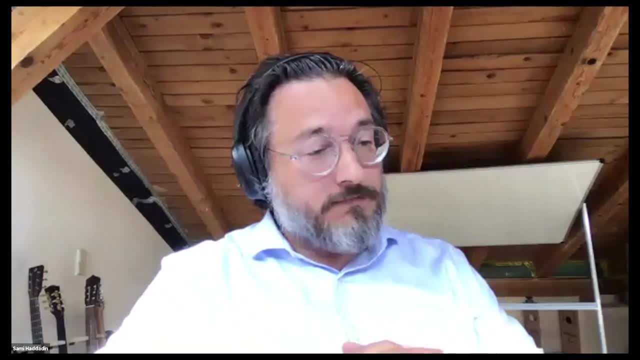 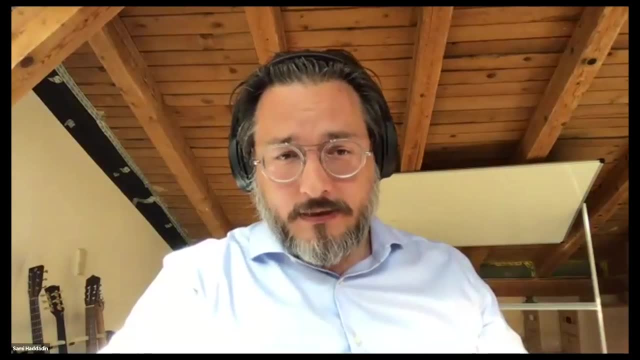 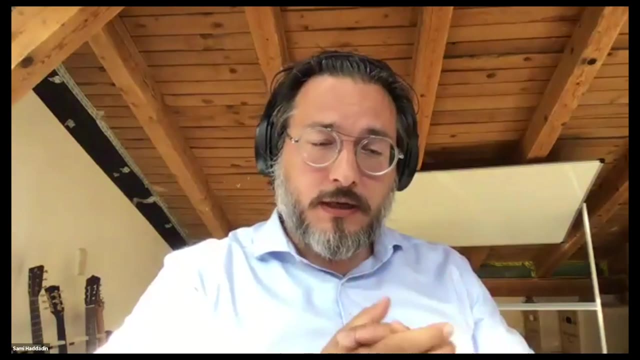 and this reaction could cause many responses and this is why a lot of our work is really about kind of regulating these reactions. so I think it's really about definition and being as specific as we can to not confuse concepts of humans and concepts of machines, I mean a mannequin. 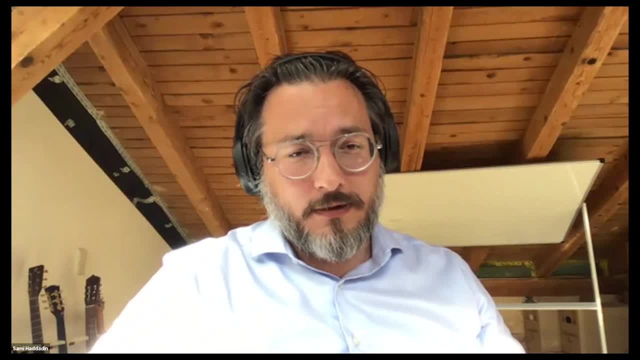 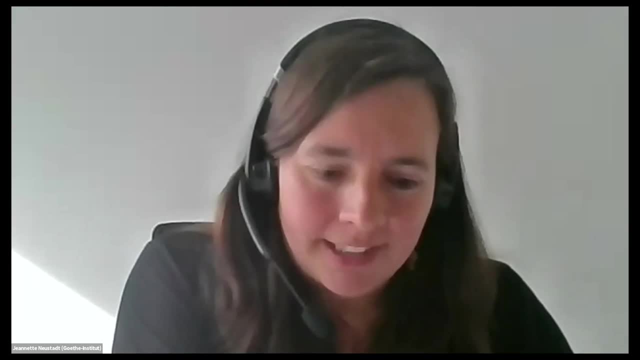 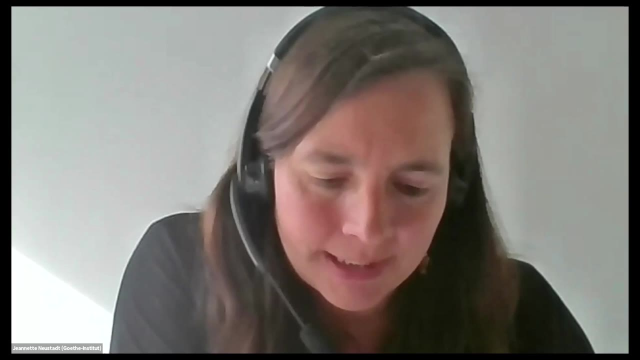 is not a human. it just looks like a human right. still there is nothing in it that. so the ghost in the shell is missing. so we have another interesting question from Madulika Matsunda- I hope I pronounced it right- about studying a robot culture. it's for. 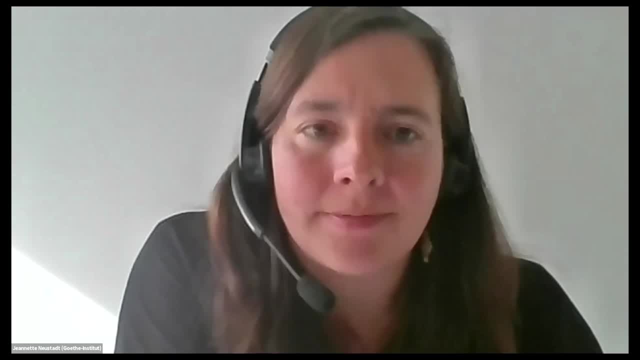 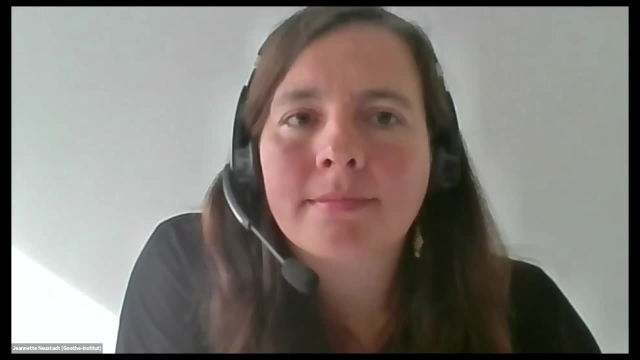 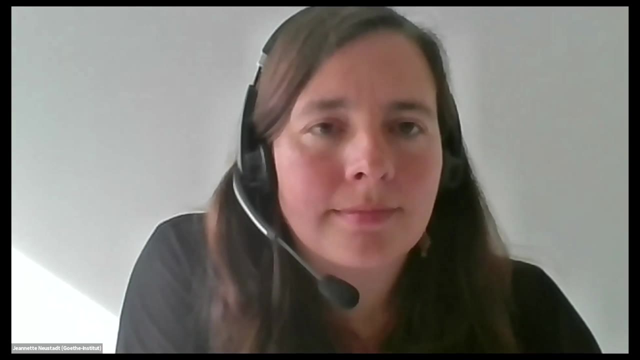 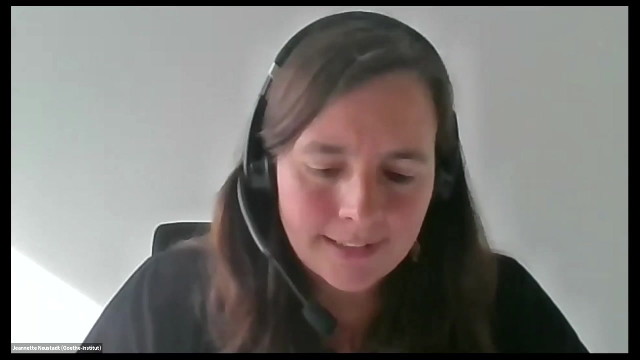 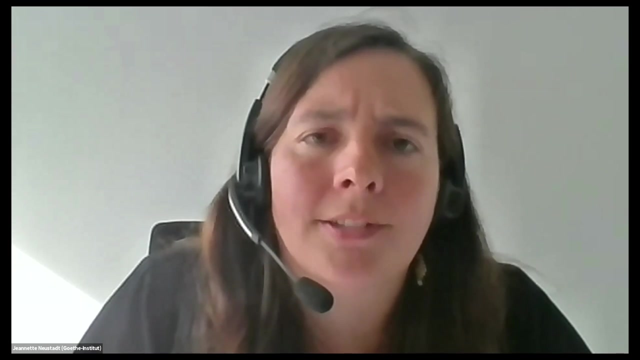 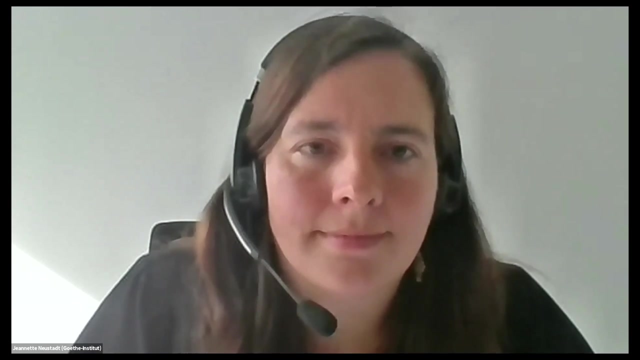 Kate, maybe you can speak up. Madulika, oh, maybe she has left already. there were also two questions about the replacement of teachers and how can AI be integrated into the education of young students. maybe one of the questioners will speak out. Hello, Hello, Hello, I'm Noura. 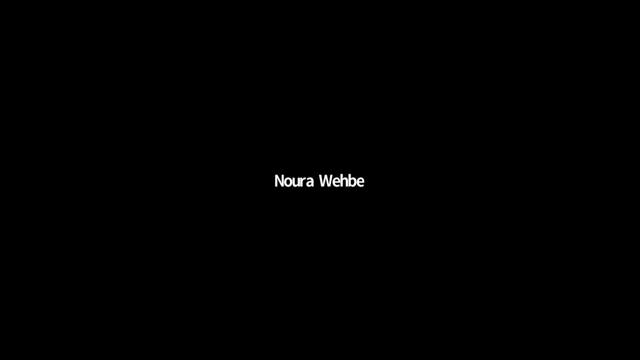 I'm a biology teacher for middle and high school students. this is really an interesting topic because I know that once robots in the future, there will be replacement of many, many jobs, but at the same time, a lot of jobs will be created. so, with respect to educational systems, how will the artificial intelligence or robots be? 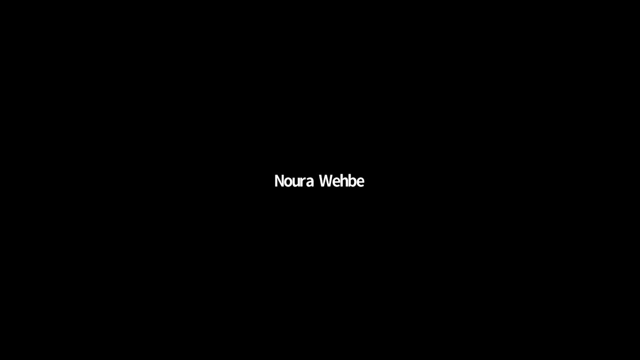 integrated, like it would be cool for me, as a teacher, to teach with the assistance of a robot, maybe hologram, or to show 3d structure, because I'm in the scientific field, you know biology and stuff. so what are the insights about education and teaching? or will there be only integration of? 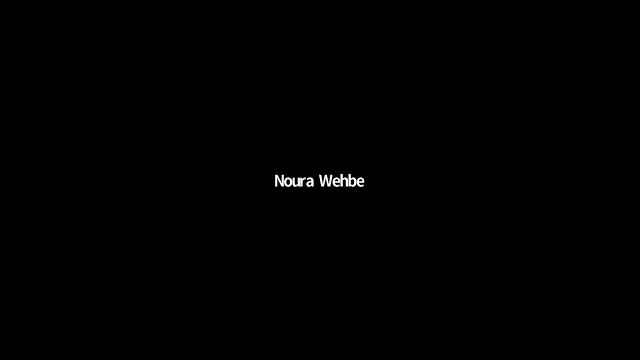 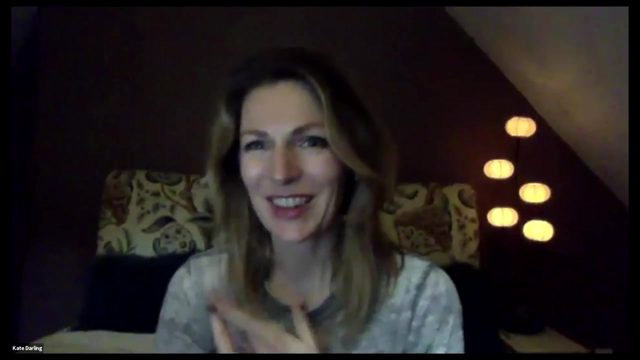 certain- maybe jobs or I don't know- tasks, but not a full replacement. so your thoughts about this, please? well, I think there are two questions here: there's what will happen, what's likely to happen, and what should happen. so if, if the question is, you know, should? 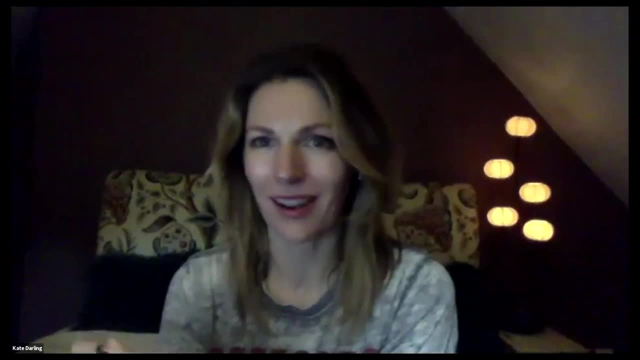 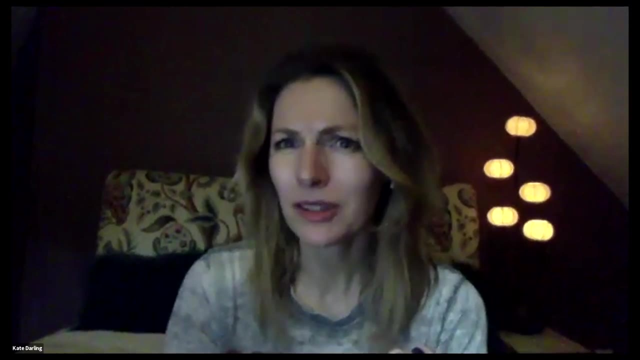 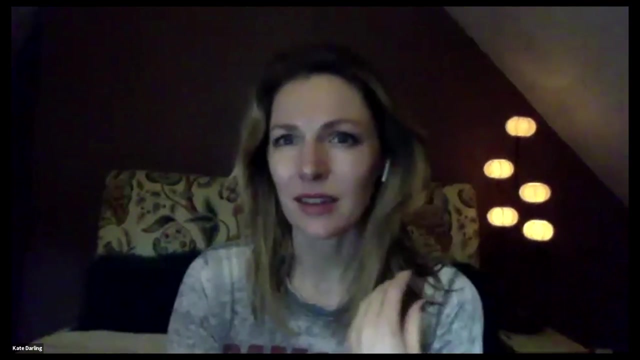 robots be replacements for teachers? absolutely not, like even as we advance the technology. I don't think that that's really again the potential to recreate some a skill that we already have, but there is a lot of potential, I think, for robotics to assist people in doing their jobs. 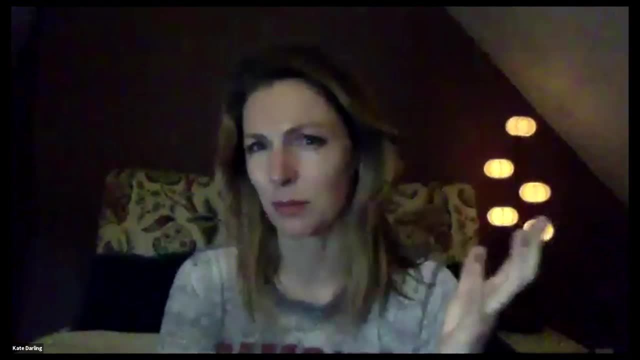 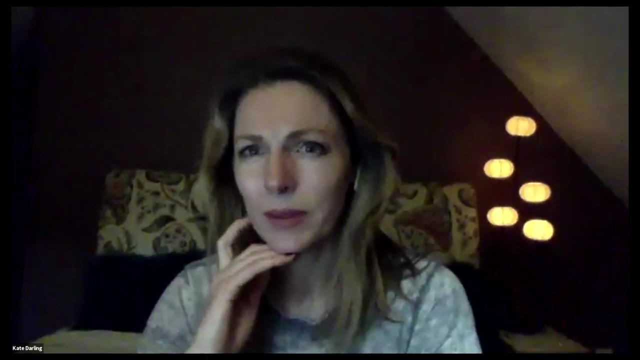 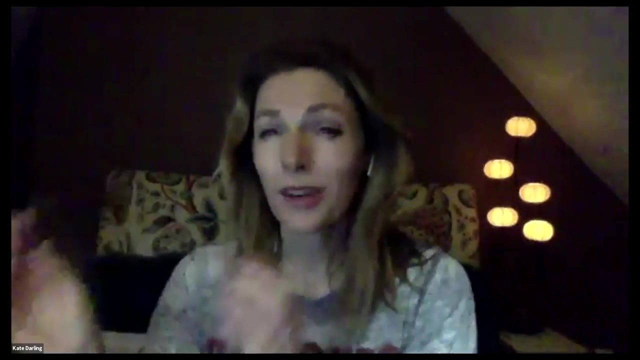 better, and so one example that I know of that has been researched a little bit in the educational space is that Brian Scazzolatti at Yale, his group, has done some work around what challenges teachers are facing in the classrooms, and, you know, one challenge needs to be solved politically, which is that they don't get enough one-on-one. 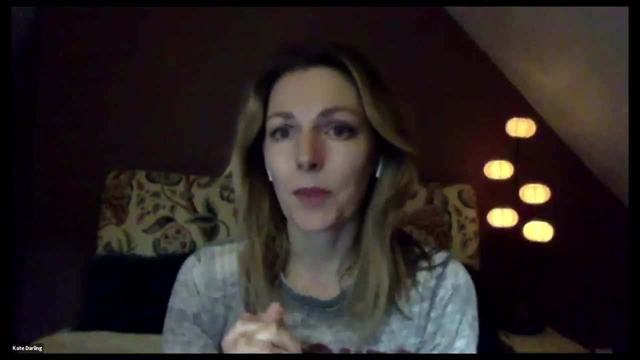 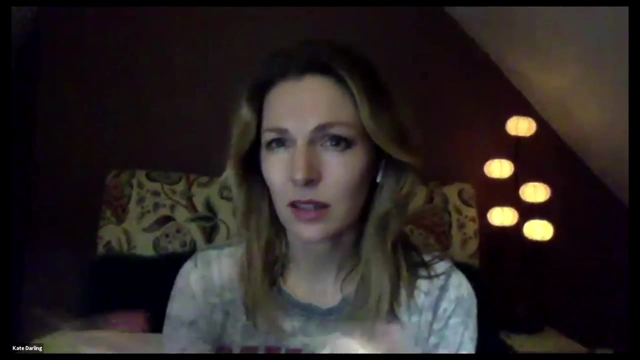 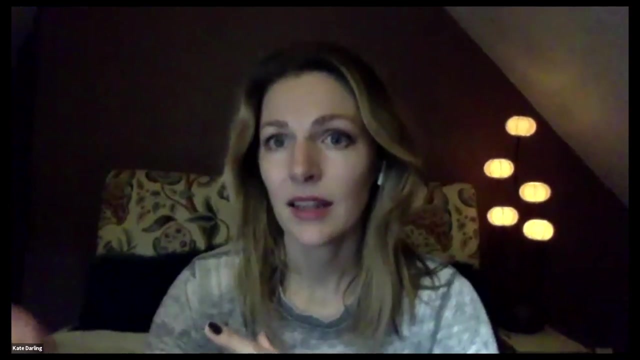 time with the students and can't help them individually. one challenge that robots might be able to help with, though, is that some teachers, so they did, they did. they worked with some teachers who teach English to non-native speakers, and they said they were struggling with the fact that the kids didn't want to make mistakes in front of others, and they 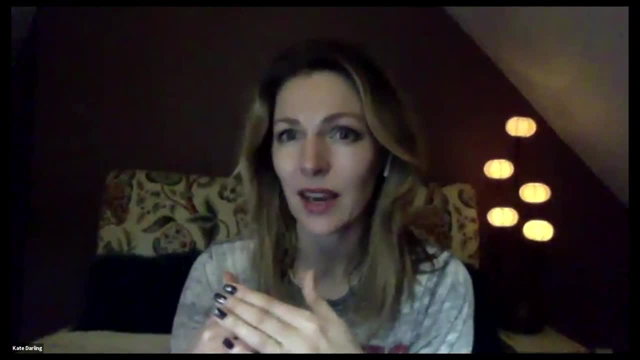 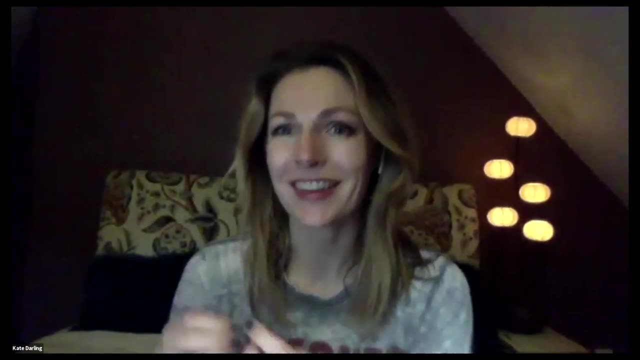 didn't even want to make mistakes, one-on-one with the teacher, because it was embarrassing and without making mistakes, the teachers couldn't assess, you know what- where the kids needed help. but they figured out that you know, introducing a robot into, like a more holistic program, having the kids 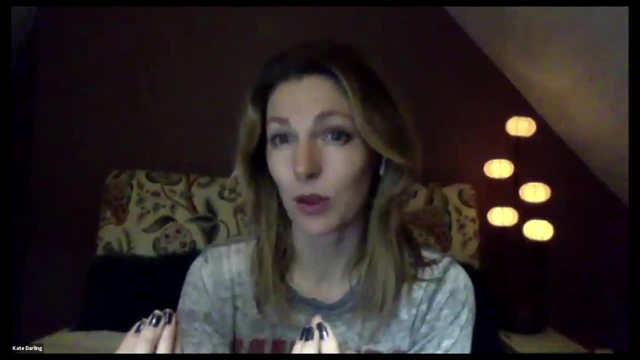 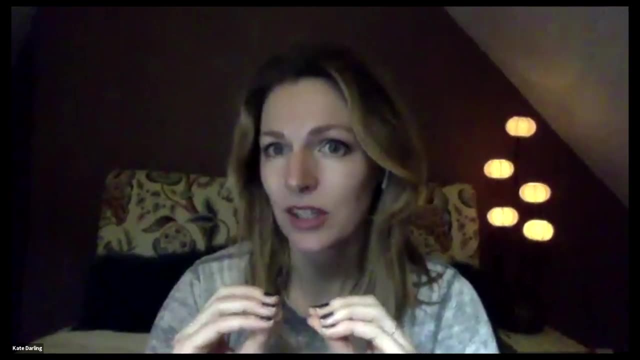 sometimes interact with a robot. they were. they were more willing to make mistakes with the robot, because there's not this idea of being judged. so I don't. I don't think that a robot is a good idea as a good replacement for a teacher, but I do think that, as part of a more holistic curriculum, robots 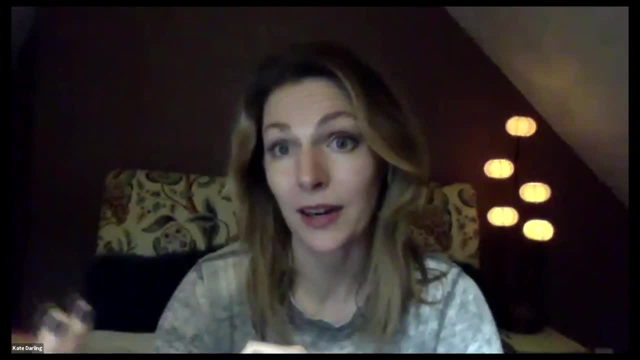 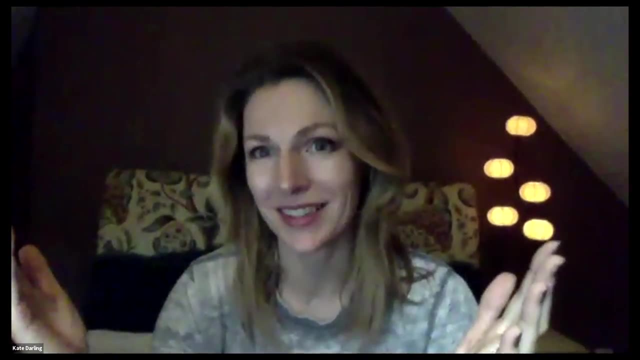 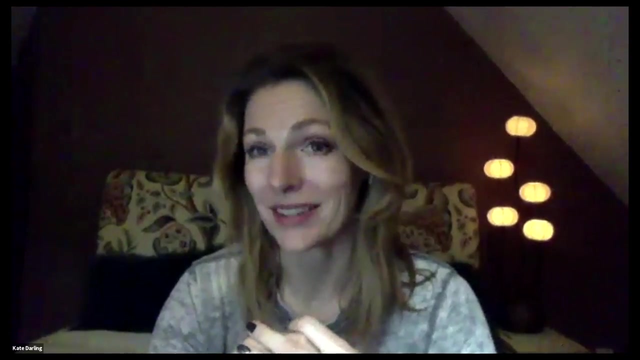 could be introduced as tools and could have something to offer, and that's how I would hope that they would be used as well. you never know it again. these are choices that we are making as a society as to whether we're using robots as replacements or supplements, and you know part. 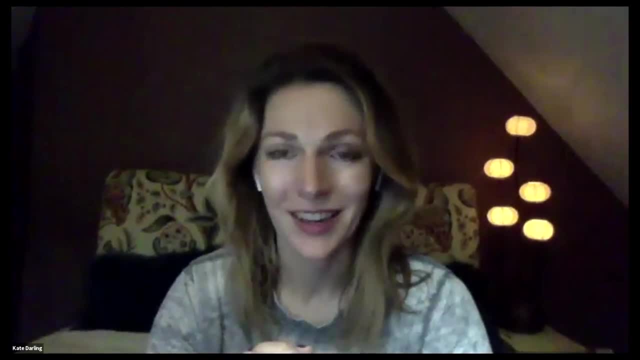 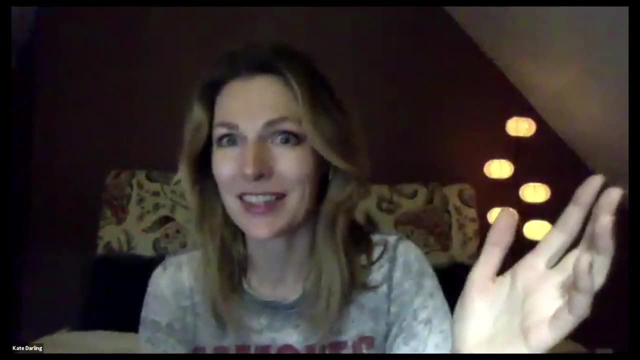 of that is on how the technology developed, but part of that is also on, you know, our schools underfunded. do they need something to replace a teacher that's not as good as a teacher? are they going to turn to technology to do that? that's unfortunate, but that's also a larger. 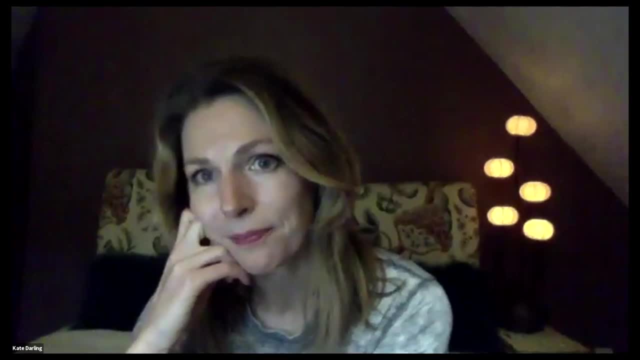 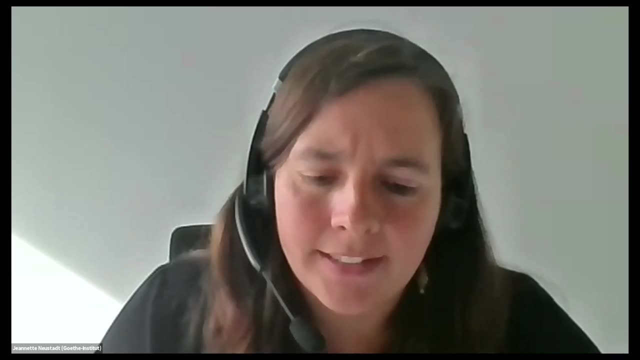 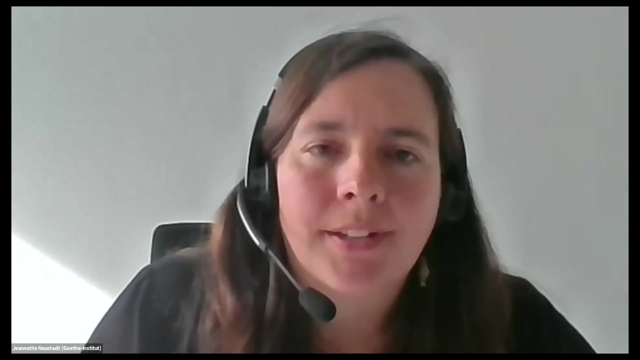 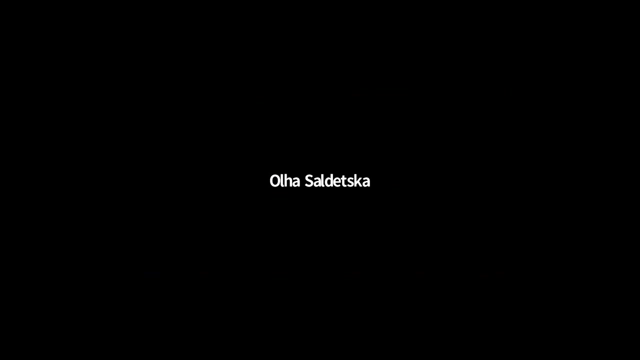 political question than just a question about the technology itself. okay, I have another question from Olga Zaldeska about the safety from robot human interactions, so maybe you want to ask this question. so, yes, hello, thank you. yeah, actually it is quite an intricate question and it will be very curious. 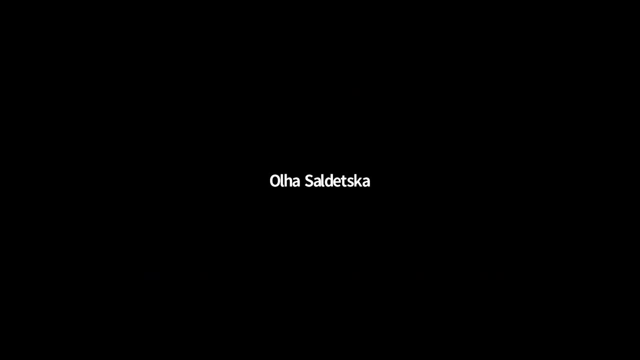 about the opinion of the specialist. as for this, there is so much to be said and there has been so much fiction written and discussions, so maybe it could be there. there is a tendency to be said, and there has been so much fiction written and discussions, so maybe it could be. 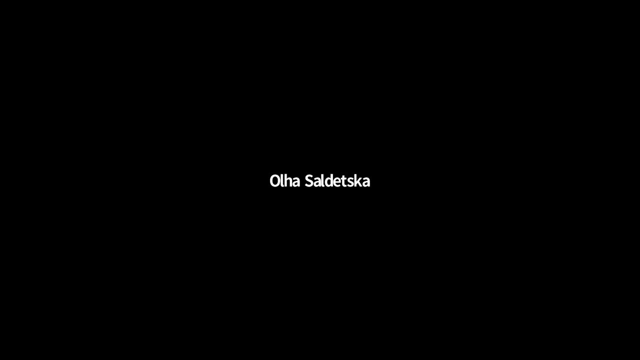 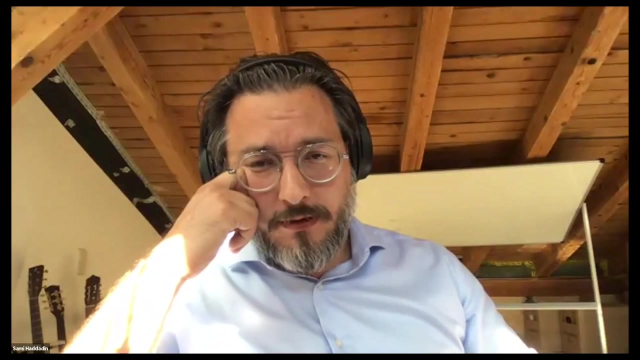 there there has been so much fiction written and discussions, so maybe it could be there. there is a tendency or the view that is already formed and followed by the speakers today. yeah sure, I mean, I can if you, if you like, Kate, I can take the first shot and 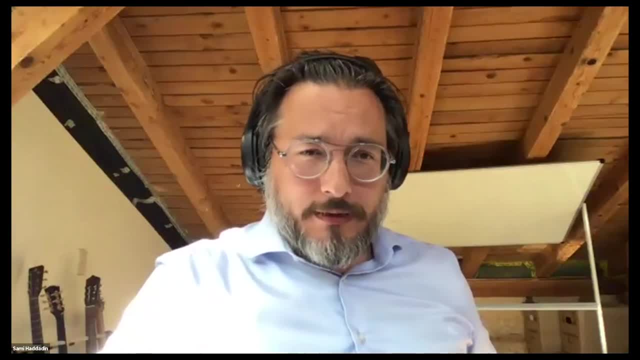 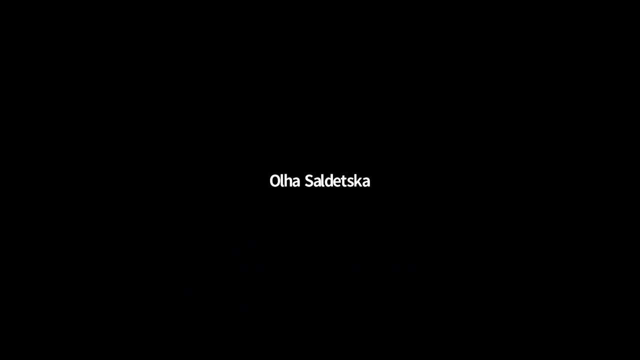 since at least I have an opinion, let's put it this way. my dissertation was was called towards safe robot approaching azimuth's first loss. so I feel a little bit obligated to to say: at least, you know, I'm not going to say anything about it, but I'm going to say that I'm not going to. 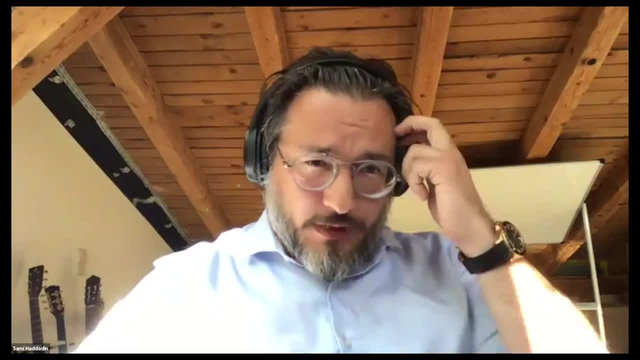 say that I'm not going to say anything about it, but I'm going to say that I'm not going to one or two things about that. it's a pretty important question. it has always been an important question with any machinery. so, regardless whether you talk about a car, 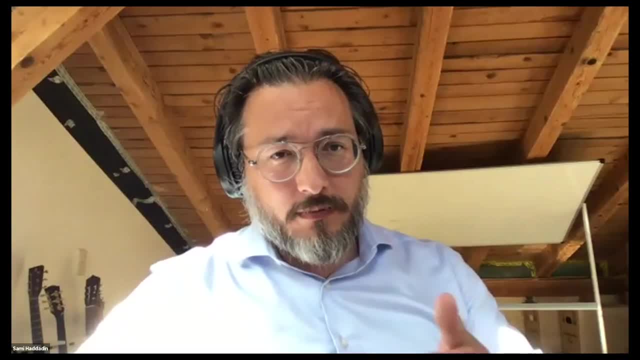 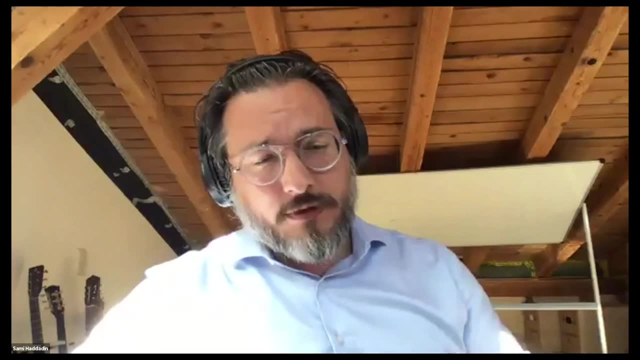 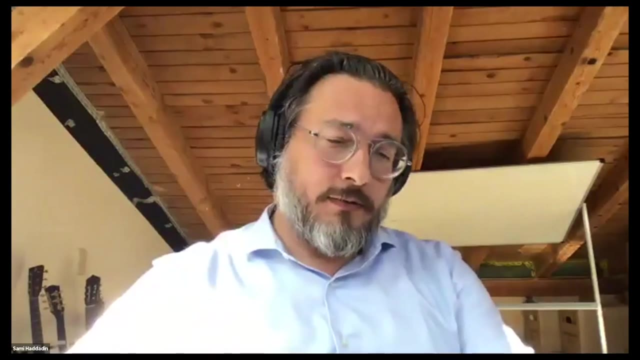 a plane, classic industrial robots, driver's assistants, what? what martin was saying in the beginning? and, and it's always the first question is always: who's responsible? right, that's in the real world, right, philosophical or ethical question, but really on legal terms, everything boils down to who's responsible and who's not responsible, and who's not responsible and who's not responsible. 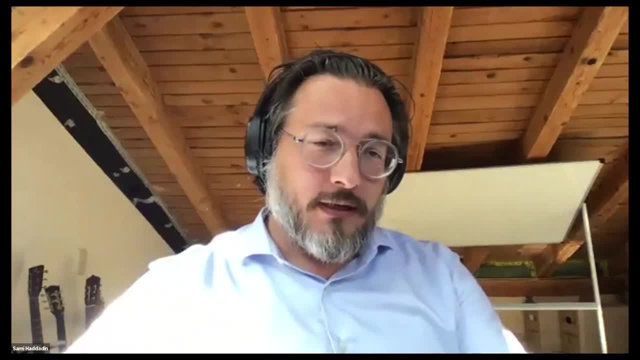 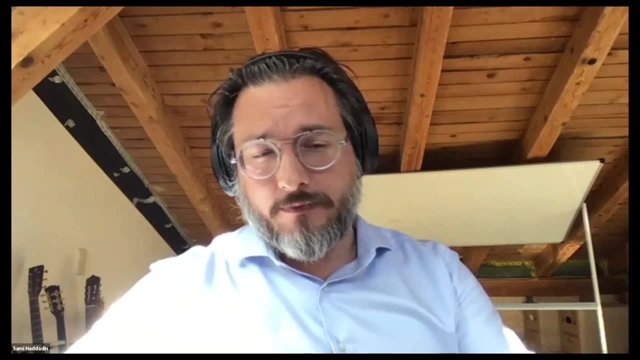 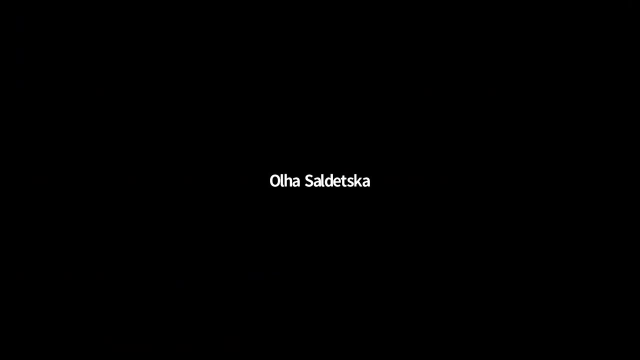 that's unfortunately, unfortunately one of the core questions we have to to deal with in many directions and, I think, just out of necessity, safety is always, at least if you go to the real world, not only stay in the labs and in the research environment as soon as you go out to. 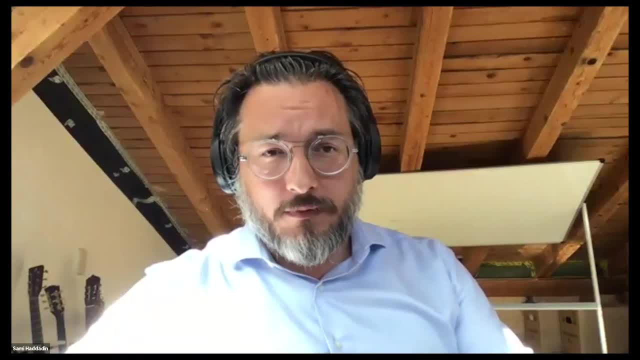 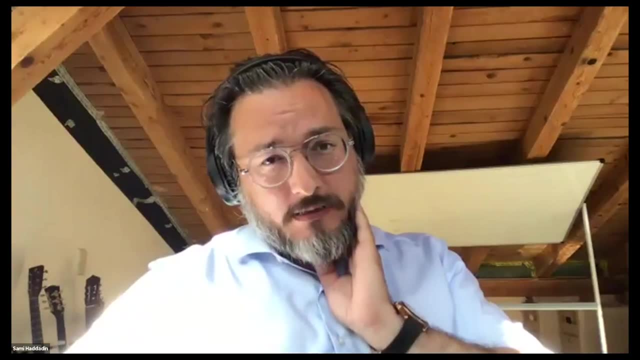 the real world, safety is prime, and without safety, you are in legal trouble, right? I mean let's, let's be clear on that, especially if this is a- it's a real machine- that is potentially dangerous, meaning that if you didn't do your job as an engineer, if you didn't do the right safety, 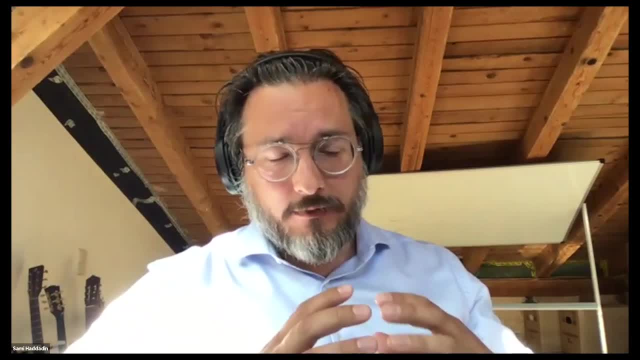 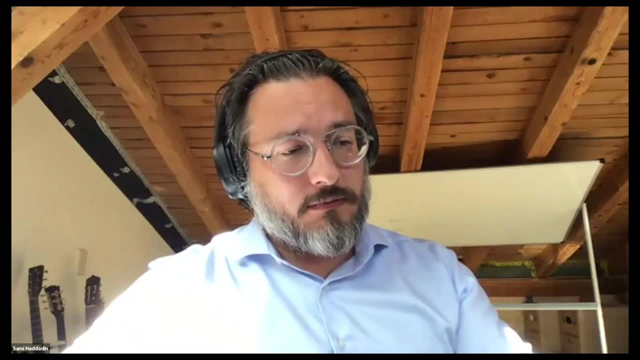 developments. but this is just a kind of a kind of a legal aspect. at the same time, there is a huge body of work all over the world over the last 20 years that has targeted for making increasingly autonomous systems aware. so now we're coming to this concept of the of two questions. 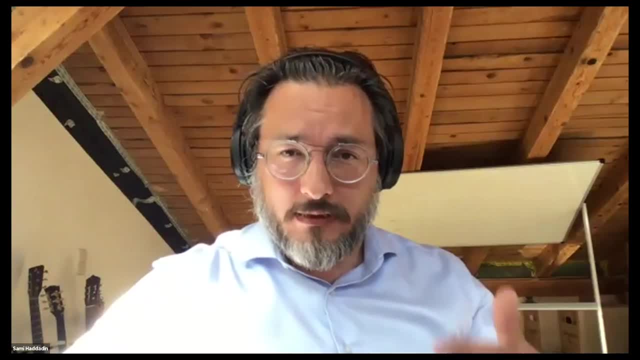 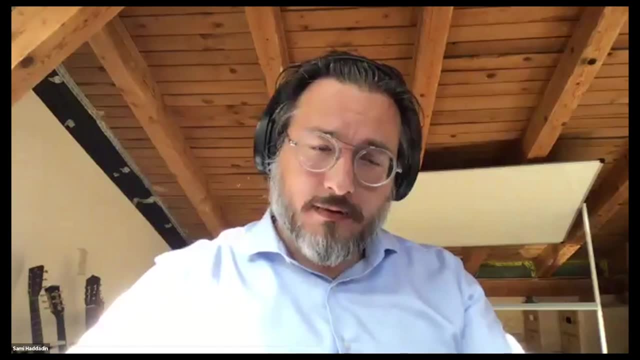 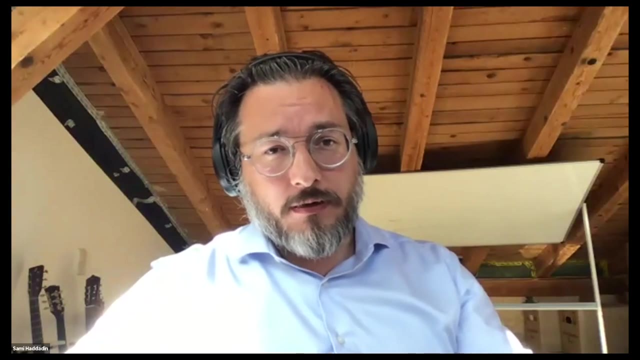 four about the stealth and the motivation and the causality of of systems own actions, to understand how can robots reason even about potentially unsafe situations and increase safety. so there is a lot of body of work, starting from making a system from a design point, of from a design. 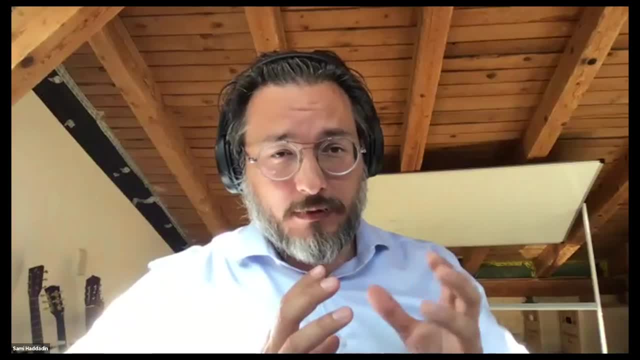 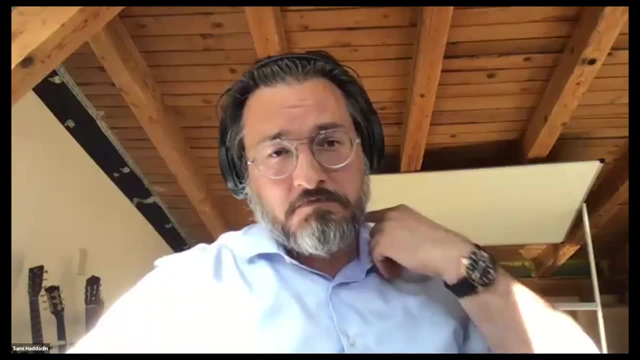 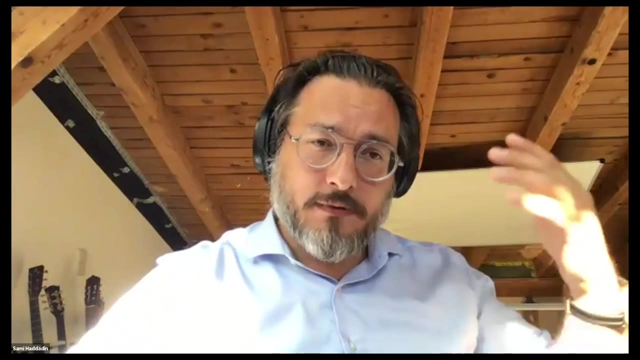 standpoint as safe as possible, meaning extremely light, right, I mean flexible, compliant, sensitive. that's why the sense of touch is so important, because if I crush your hand when I'm shaking your hand, I'm probably not a pretty safe robot. so I need to have this dexterity and tactility. so this is kind of an embodiment, and then comes 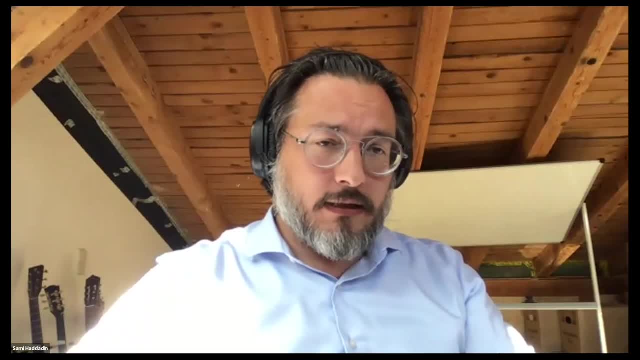 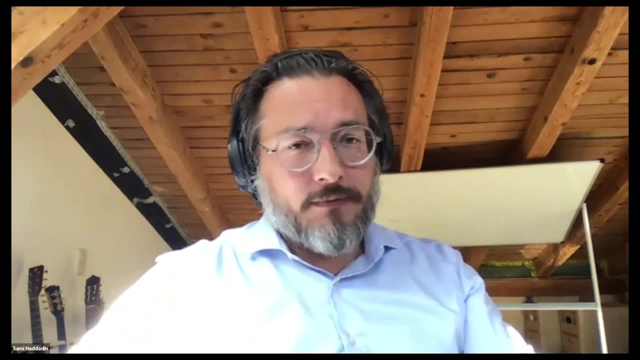 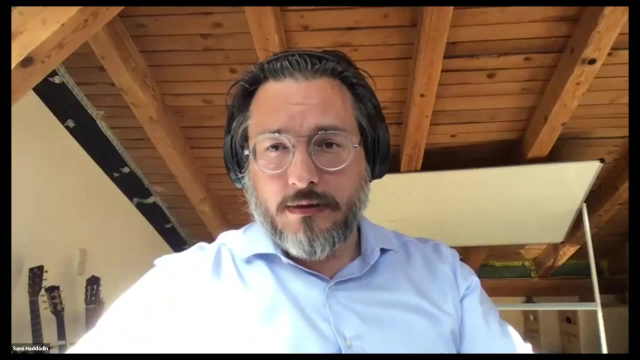 more and more of this abstract reasoning and- and this is a lot of work that is existing there. however, I must I must also say that bringing them to the real world, meaning applications, products that reach you guys- is still a large hurdle. so you can see this in cars. I mean just a lane. 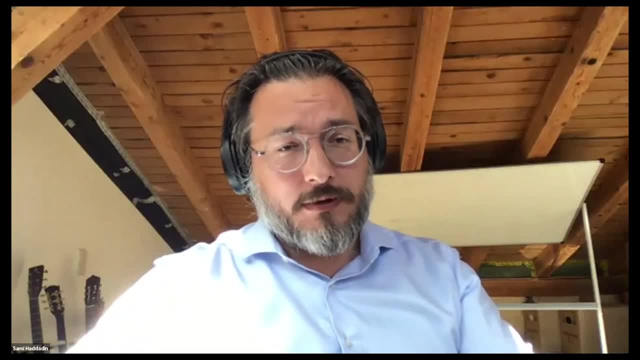 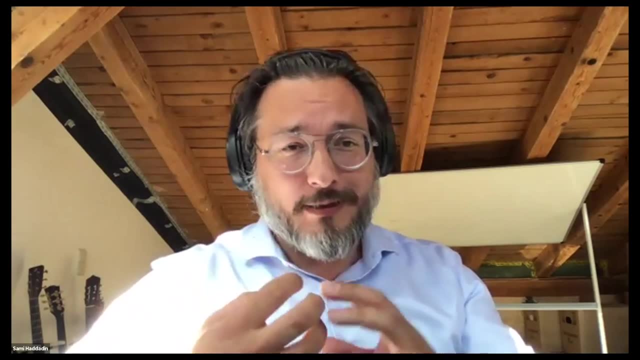 using a car is already a big challenge, right? I mean you also. there's some incidents and an accidents also with autonomous cars, and I try to give you a little bit of the understanding that mobility is not the same thing as manipulation and and there's increasing complexity about that. 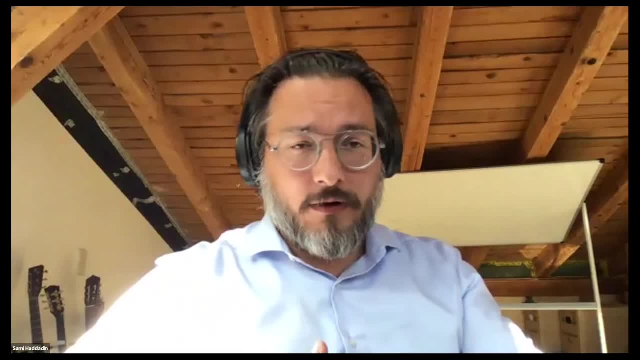 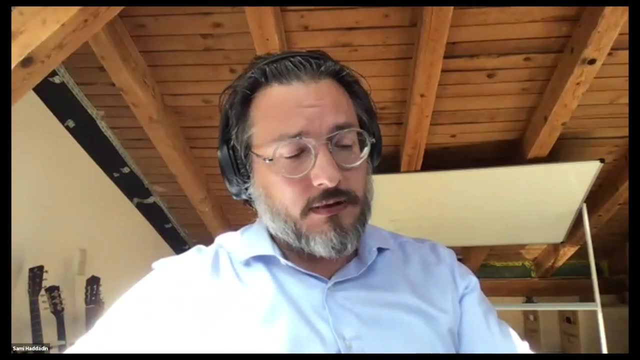 so the answer is it's. a lot of our work is centered around safety, especially because we have bodies that might hurt humans and we try to design them as as safe as possible. there is even entire standards dealing with that, and this is a huge and important issue in terms of safety, and then also in 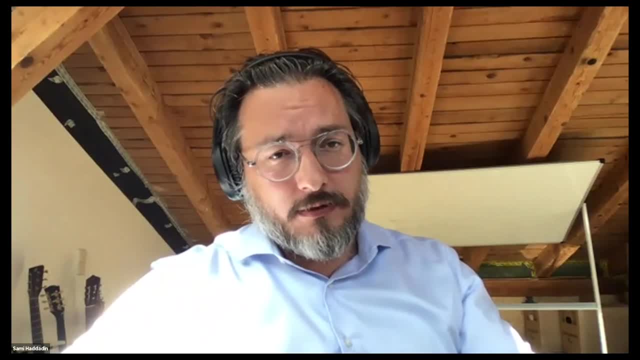 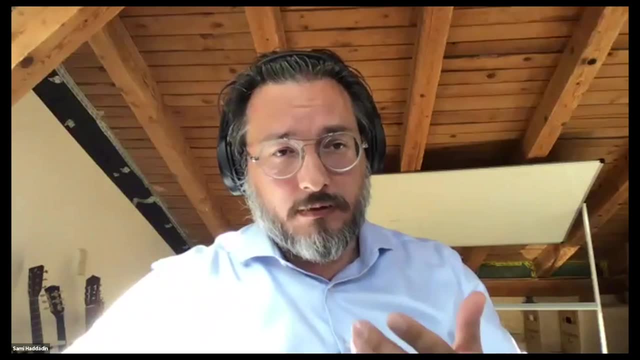 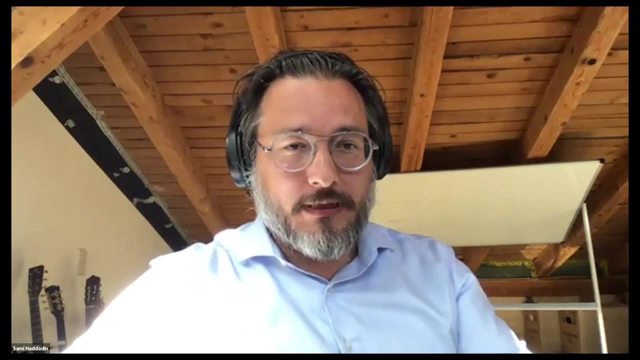 important step to be done, and this also kind of relates to the question that i was asked before about education. it's also about educating people to be able to understand robots, to to learn to interact and use them, so kind of driver's lessons- uh, i mean robot driver's licenses in some sense. 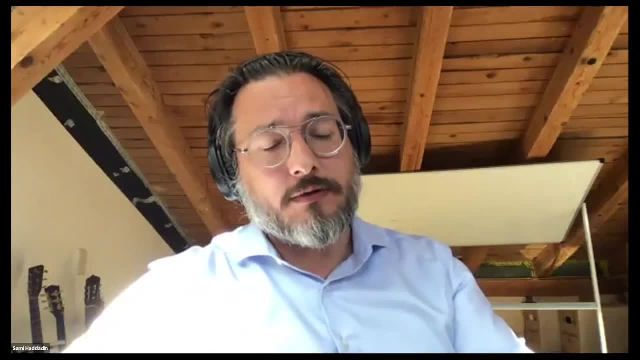 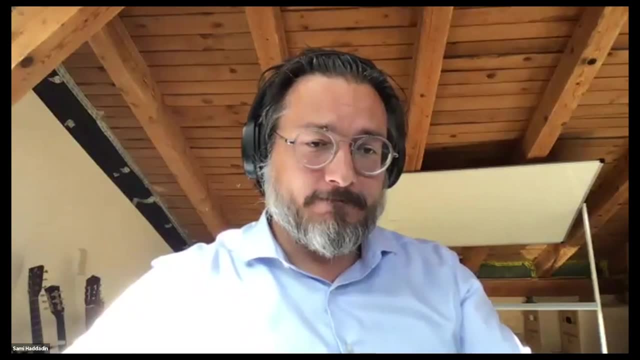 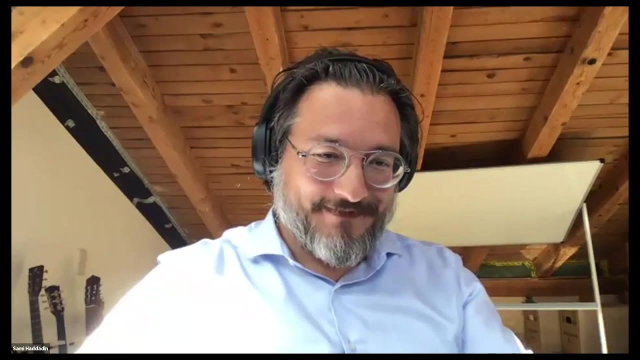 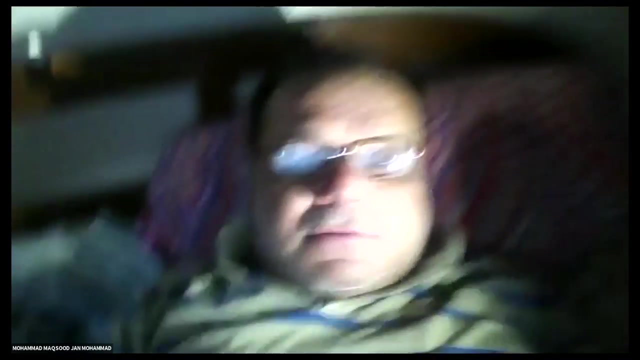 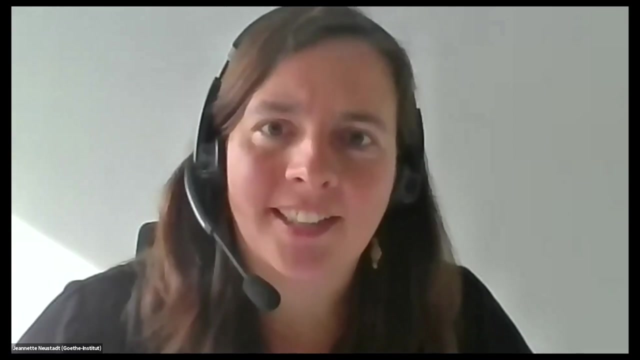 i mean only if you, if you're educated, if you know how to use these systems, then true safety can be achieved in a way. right, it's like with any tool, i guess. yeah, yeah, thank you, sounds very soothing. thanks for the question. so i think we have to come to an end. unfortunately, there are so many. 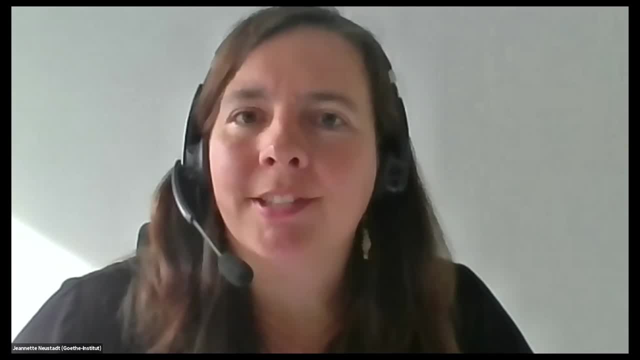 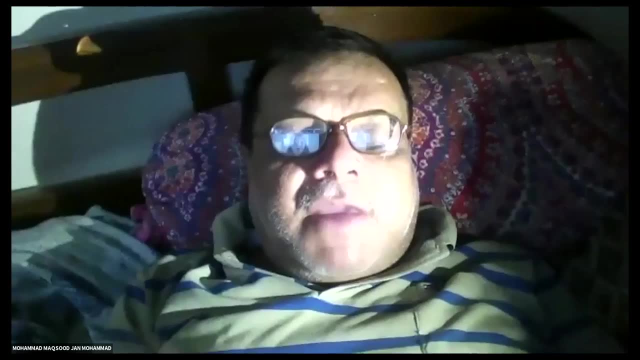 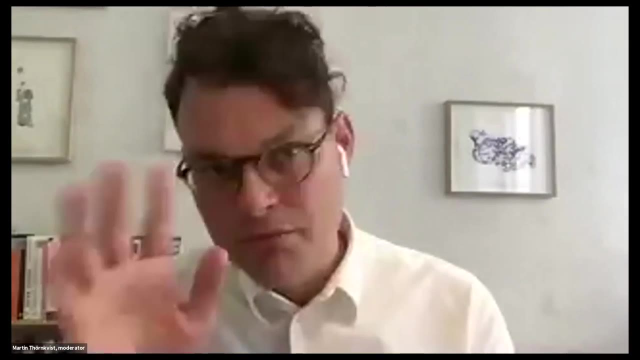 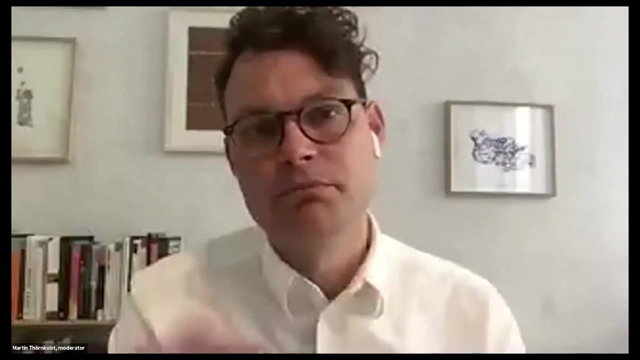 questions left, um, but, martin, you wanted to do the poll one more time. yes, it's, it's we. so what we're going to do? we're going to leave the everybody, we're going to leave the session open, but since it's now 6 pm, uh, we're gonna. we're gonna wrap up, um, but there. 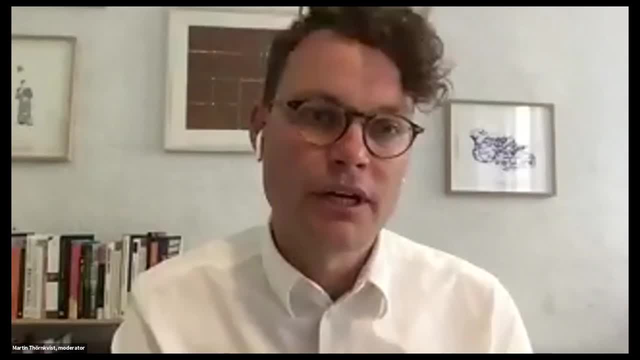 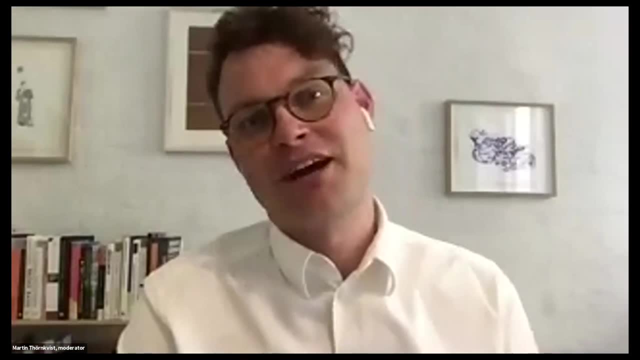 will be time for those that want to sort of hang out and keep the conversation going afterwards. um, in, in in doing so, but i've now launched the poll again and it's going to be interesting to see if we have any different answers from when we started. 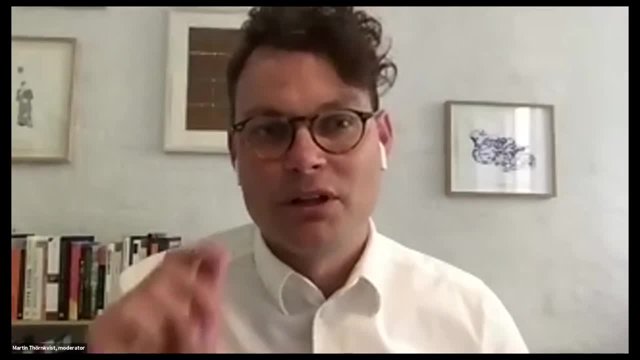 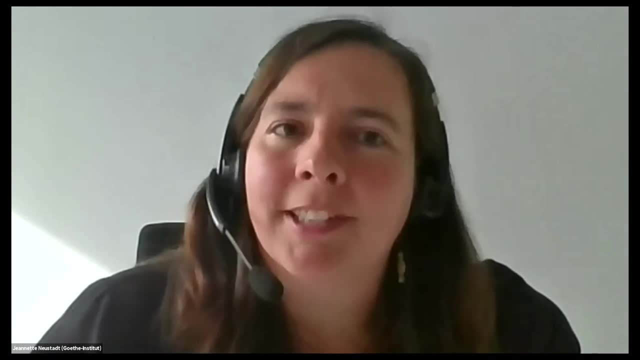 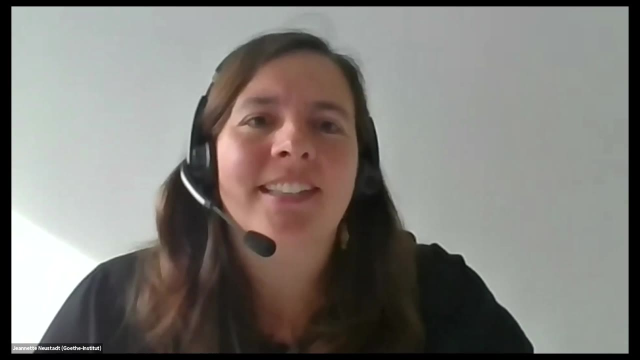 and maybe you want to, to wrap up, as people are answering the questions again. yes, i will, so at the end of our second or our third lesson. already, i want to thank kate and sami, you, martin, my colleagues and all of you that you joined the lesson. 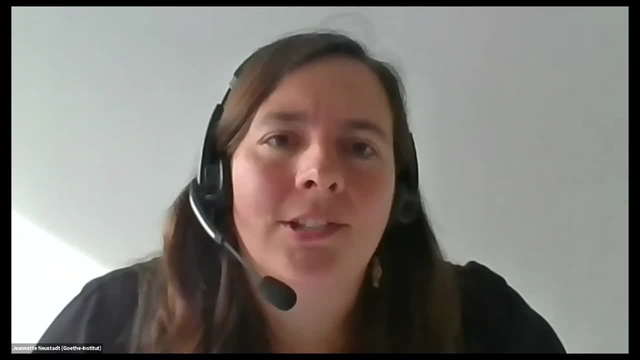 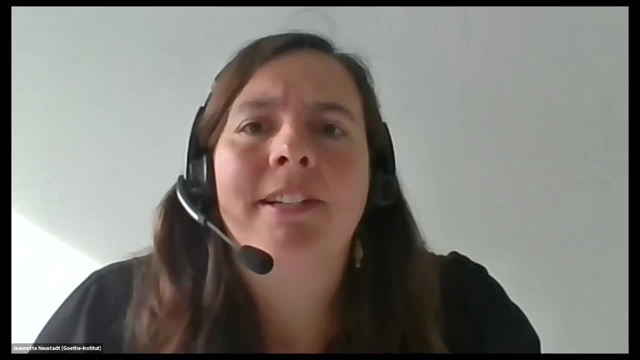 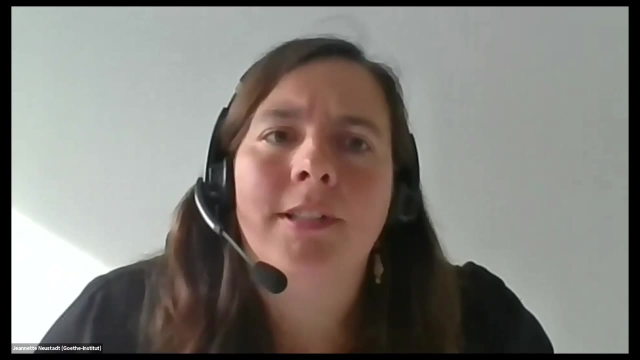 and i would like to draw your attention to the upcoming couch lessons about ai and ethics, ai and creativity, ai and the future of work, and after this couch lesson, seven more will follow. at least next time we will speak about ai and climate change with victor gallas from the stockholm. 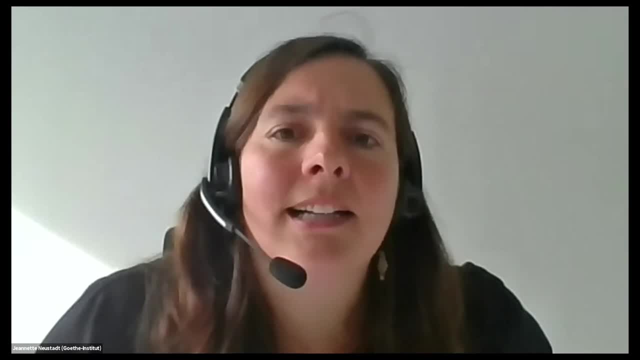 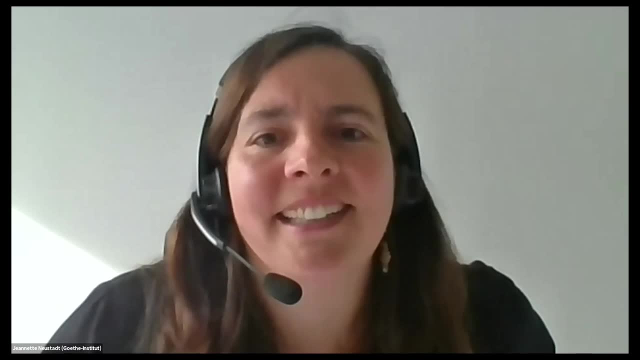 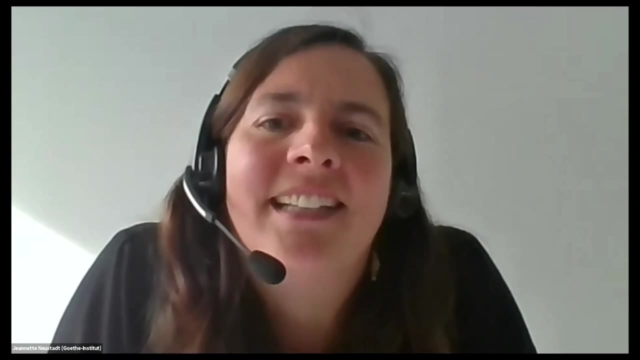 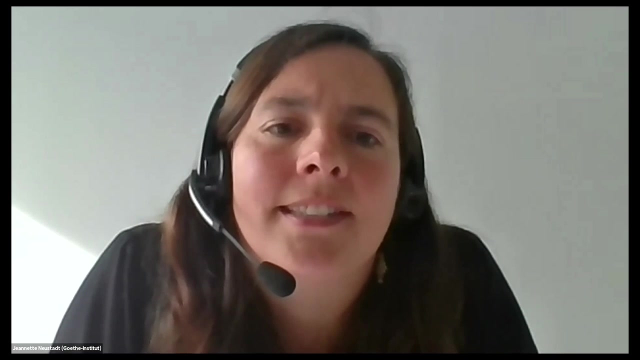 resilience center with lynn kark, co-chair of climate change, ai, and with sims winterspoon from deep mind. so please join us again next wednesday. tell your friends about the couch lesson and share them with our followers. your followers and you can find more information on our website. go to the a slash couch lessons and if you are interested in the topic, 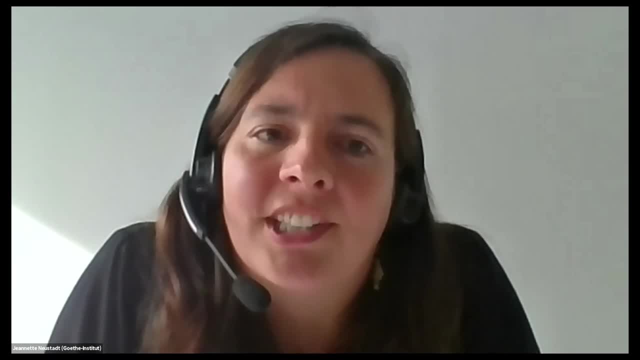 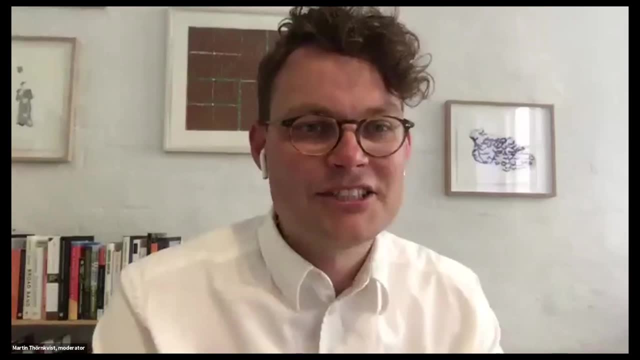 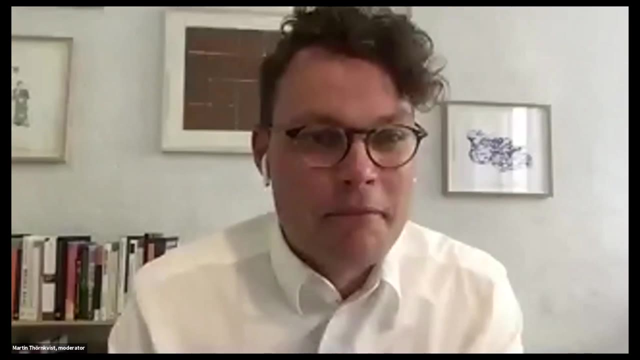 of climate change and ai. please join us next wednesday. thank you, and i can just say that the the results from the poll are actually quite similar to to the very when we started. uh, maybe there is a slight change in that. on in the first question: will robots work? 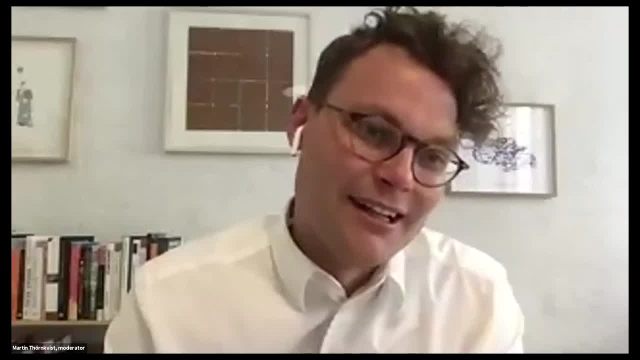 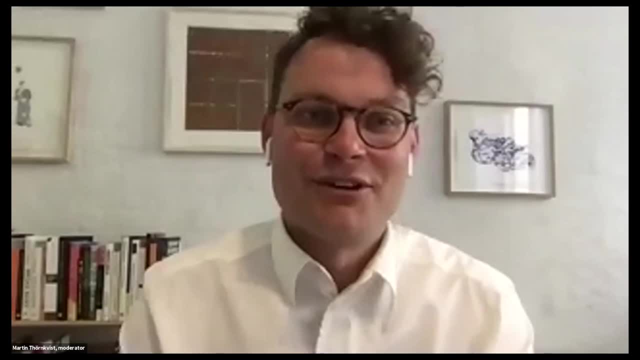 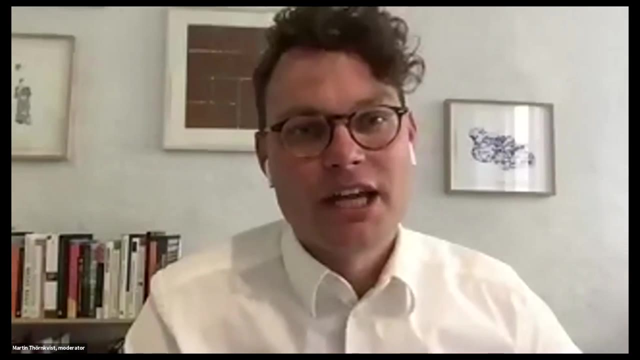 in the future. yes, so if we replace humans, more of us are now saying no, never. so i don't know if that's a positive or a negative thing, but that's at least what we think. so thank you very much to our speakers and have a good rest, a good day. everybody thanks everyone. thank you for having us.